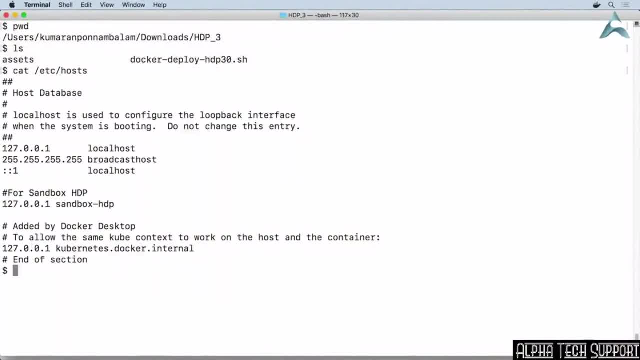 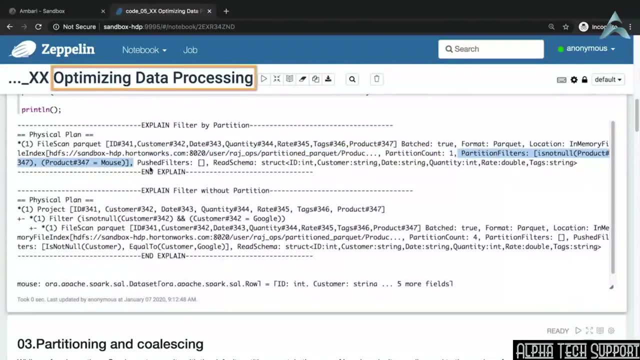 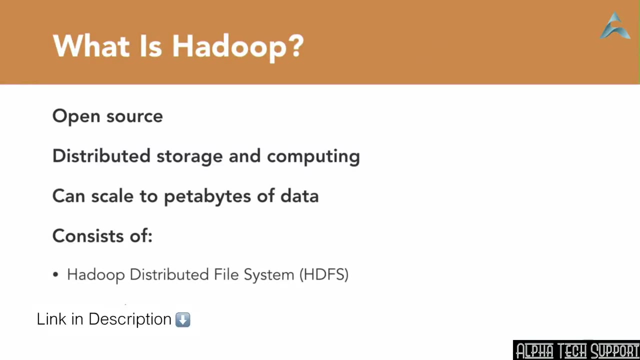 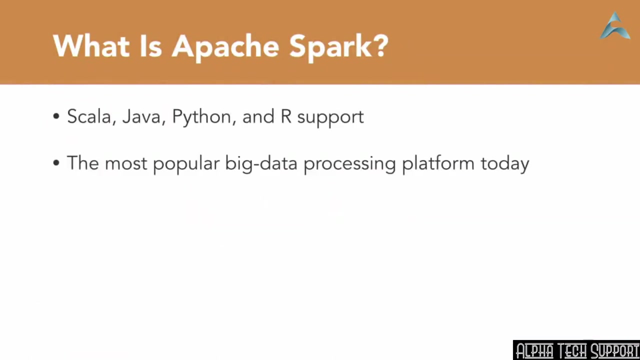 Data engineers often use tags to leverage the power of multiple technologies. For example, there is often a need for not just scalable storage, but also fast processing. Many teams find themselves using the combination of Hadoop for storage and Spark for compute, because it provides unparalleled scalability and performance for analytics pipelines. In order to harness this, 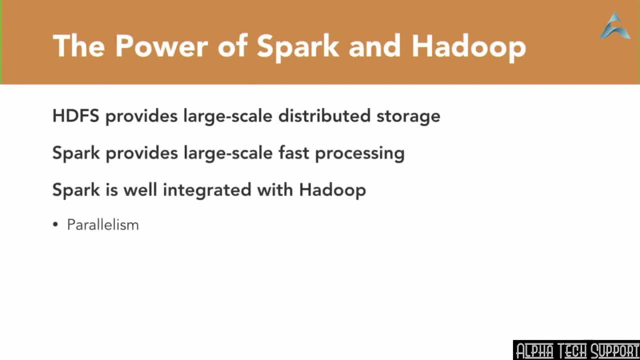 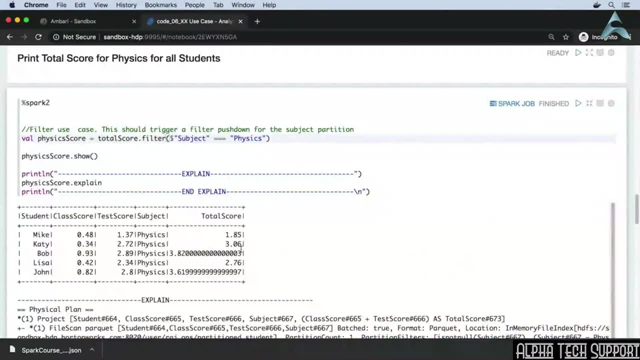 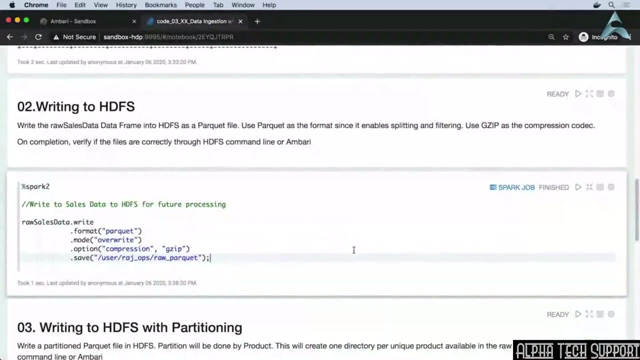 power. it is important to understand how Hadoop and Spark work with each other and utilize the levers available. I will only discuss key tools and best practices for taking advantage of this combination. We will use a Hoturnworks sandbox for this course. You need prior familiarity with. 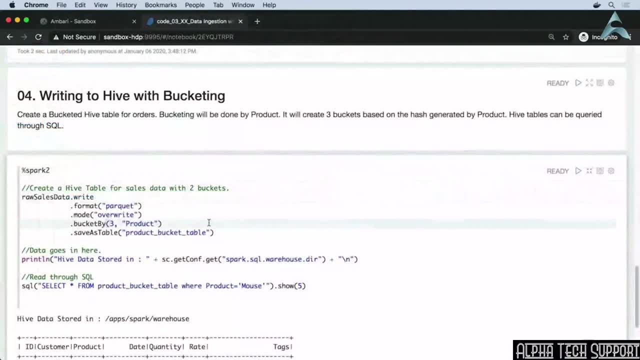 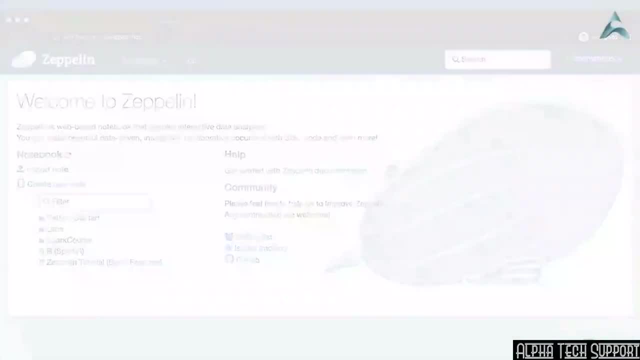 both Apache, Hadoop and Spark. In this course, we will only focus on using Hadoop and Spark together. We will also use Zeppelin notebooks for our examples. In this video, we will discuss how Hadoop and Spark work with each other. 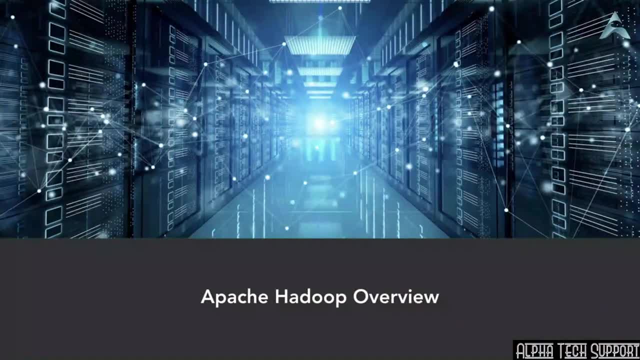 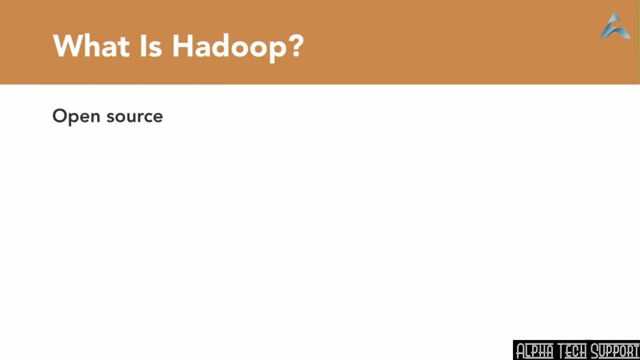 In this video, I will review the key features and the current state of technology for Apache Hadoop. Hadoop is an open-source technology that started the big data wave. It provides distributed data storage and computing using low-cost hardware. It can scale to petabytes of data and can run. 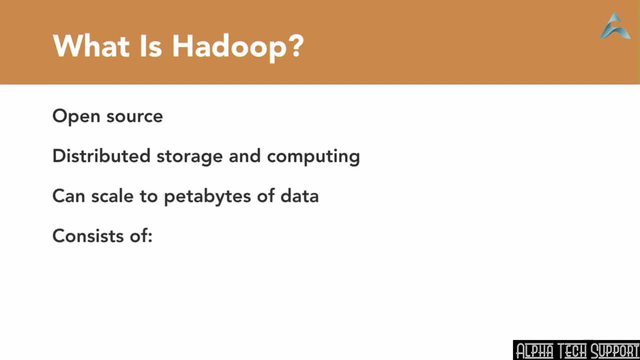 on clusters with hundreds of nodes. Hadoop mainly consists of two components: the Hadoop Distributed File System, or HDFS, that provides data storage. MapReduce is a programming model and implementation that provides distributed computing capabilities with data stored in HDFS. Where does Hadoop stand today? Let's look at HDFS and MapReduce separately. 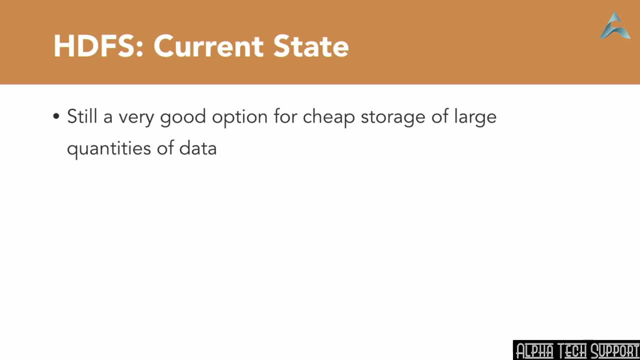 HDFS is still a very good option for cheap storage of large quantities of data. It provides scaling, security and cost benefits that help in its adoption. It is most suitable for enterprises with in-house data centers who want to host the data within their 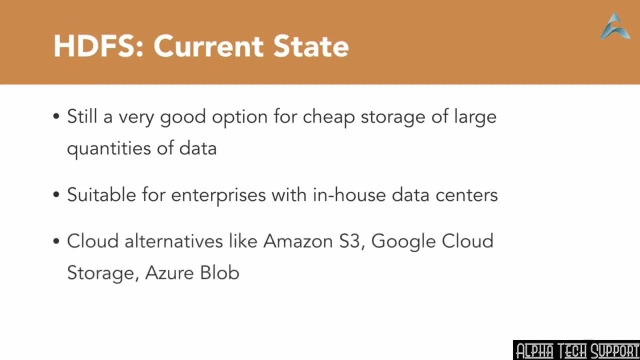 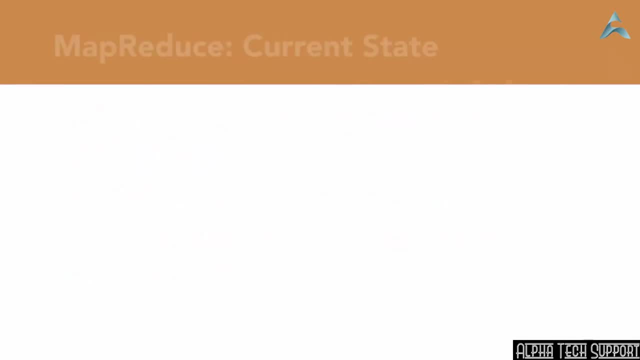 network Cloud alternatives like AWS S3, Google Cloud Storage and Azure Blob are becoming increasingly popular too. MapReduce, on the other hand, is becoming old. While it scales horizontally over hundreds of compute nodes, it is very slow as it primarily uses disk storage. 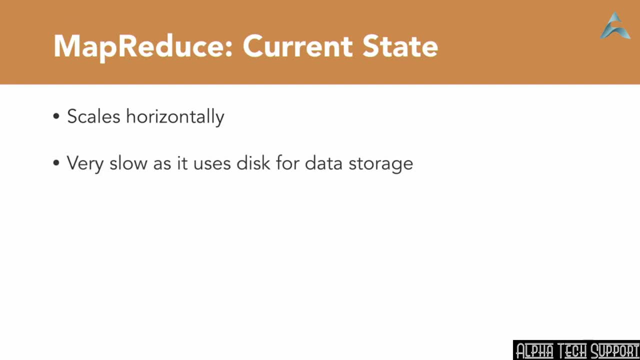 for intermediate cache. Inline connections such as client nodes and data storage are now much more convenient, as they are now even more efficient than existing nodes. The use of Hadoop is now much easier. Newer technologies, such as Apache Spark and Apache Flink have emerged that can execute. 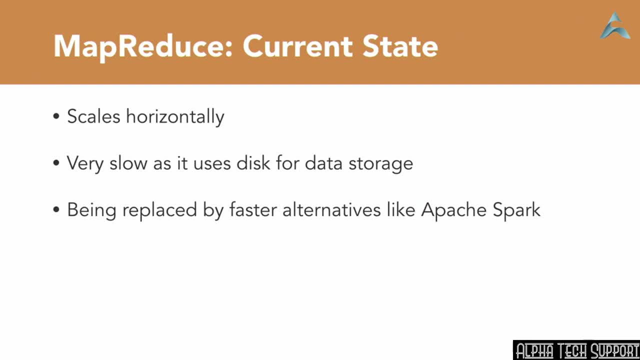 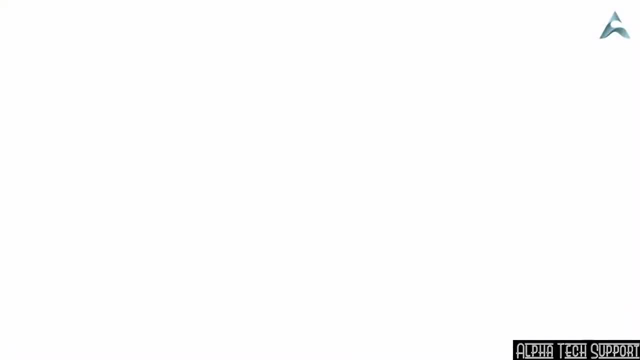 the same processing at much faster rates. The newer technologies also support other capabilities and a growing library of connectors, which makes them a better choice than MapReduce. In this video, I will review some of the salient features of Apache Spark technology that started out as a more efficient alternative to Hadoop MapReduce. It is a large-scale 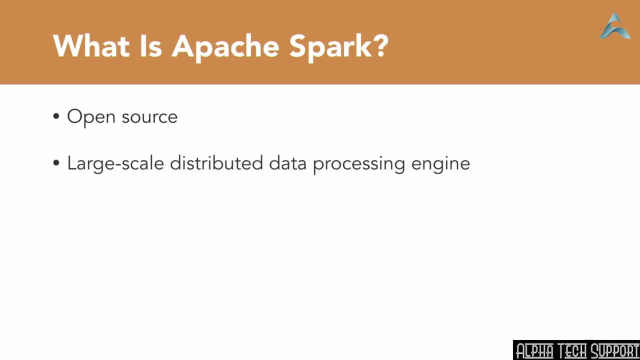 distributed data processing engine, Spark stores its data primarily in memory. to speed up computations, It has also grown to add a number of capabilities like batch processing, real-time streaming, machine learning and graphs. Spark can be programmed with Scala, Java, Python and R. 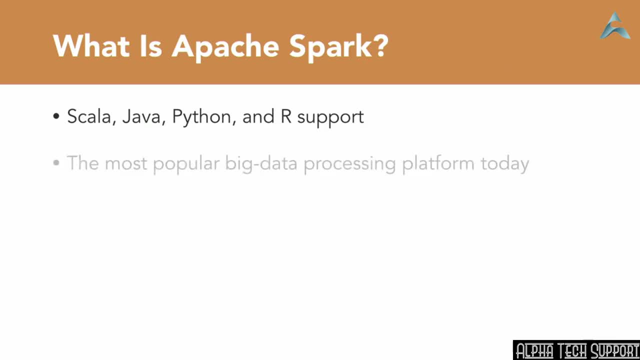 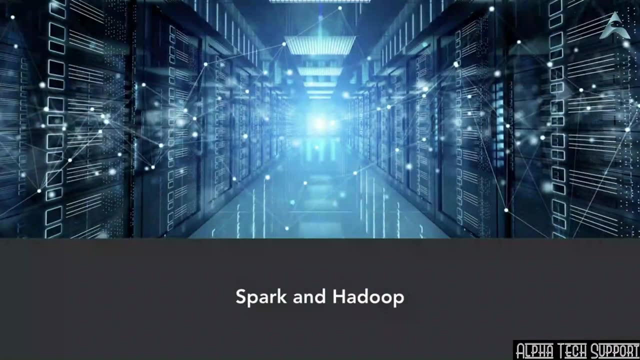 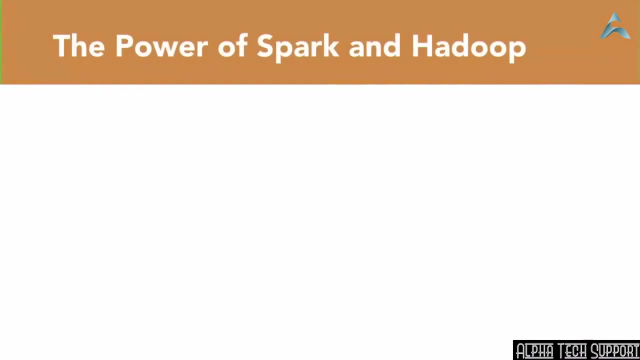 Its performance, features and programming support makes it the most popular big data technology today. In this video, I will review the benefits of using Hadoop and Spark together for big data analytics. Why is the combination of Hadoop and Spark so powerful? HDFS provides large-scale. 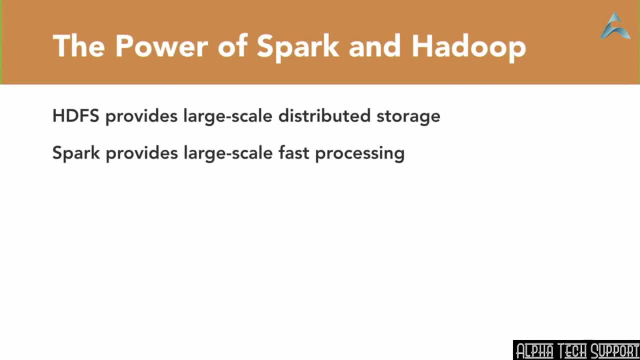 distributed data storage. Spark provides large-scale, fast processing of the same data. Together they make an excellent combination for building data pipelines. Spark is well integrated with Hadoop natively and makes optimal use of that integration. For example, Spark can access and update HDFS data. 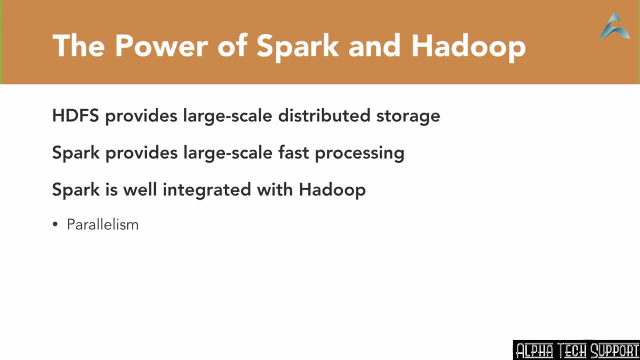 using multiple parallel nodes. There are a number of data read optimizations that use less memory and IO. Spark can use HDFS for intermediate data caching. Also, YARN provides a single cluster management mechanism. Spark can use HDFS for intermediate data caching. 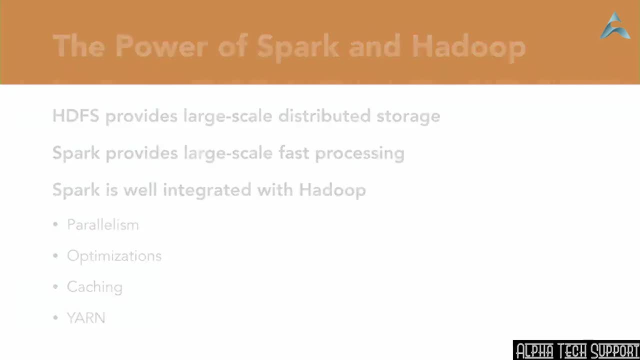 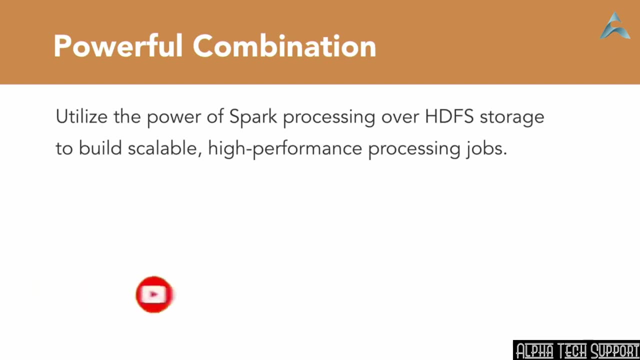 So my recommendation, especially for enterprise deployments, is to utilize the processing power of Spark with the scalable storage of HDFS to build high-performance processing jobs. In this course, I will demonstrate the strengths of this integration and provide samples and best practices for building big data pipelines with Spark and Hadoop. This course requires a number. 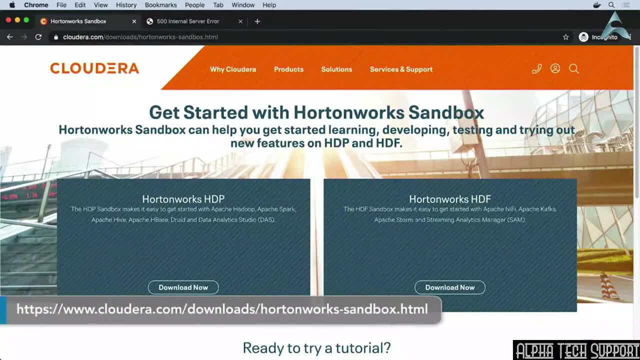 of components to be installed and set up, including Apache Hadoop and Apache Spark. We also will use Apache Zeppelin as the notebook for building our exercises. For ease of installation, we will use the FranTon Works sandbox that already pre-bundles all three components, Since you are familiar with these technologies. 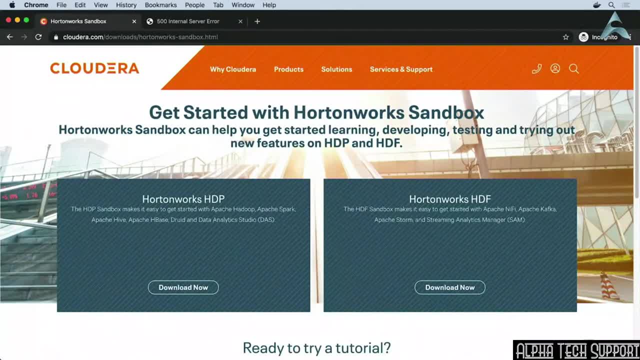 you may also try out these examples in your own setups. We will use the docker version of the sandbox for the same task on Mac. Please join your team and leave comments and subscribe to the channel if you are interested in staying updated on it. As we move on to the next chapter, we will also разбackly talk about processes and integrations by the software and the hardware. We will also discuss how you can create strong space for data type and whether data type has been added for it. 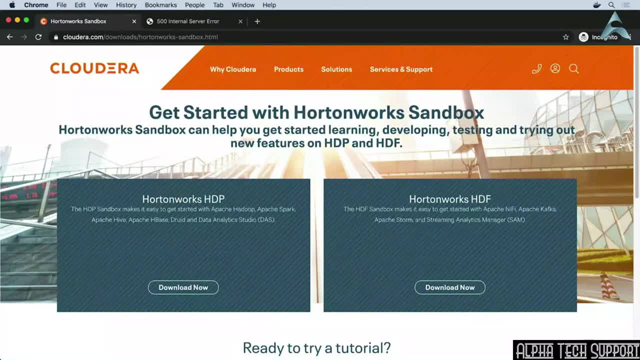 Please install docker. if you do not already have it. The sandbox itself can be downloaded from this website, cloudiracom. slash downloads. slash hotonworks sandbox dot html. You should download the hotonworks http sandbox. It provides downloads and instructions for Mac, Windows and Linux. 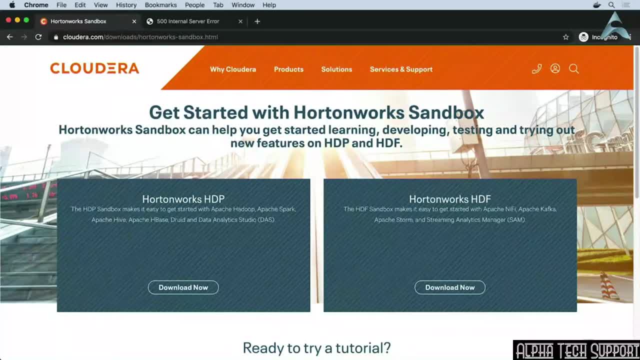 There is also documentation to set up and troubleshoot. Please use the same if you run into issues with other versions of the sandbox. Windows installation can get tricky and may require hacks to get it running based on your individual setup. Before we begin, please make sure that the docker's 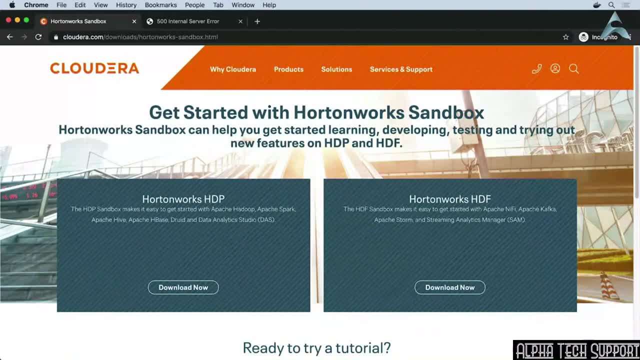 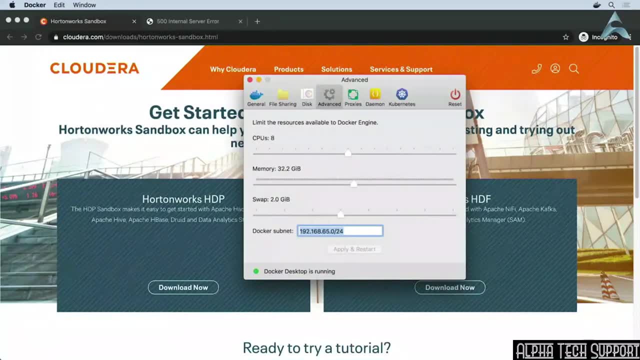 setup has sufficient memory and CPUs allocated to it. Please provide at least two CPU cores and 8GB of memory to docker. If you notice sluggishness in the UIs or services frequently stuck, you may want to fix it. If you have any issues with the UIs or services frequently stuck. 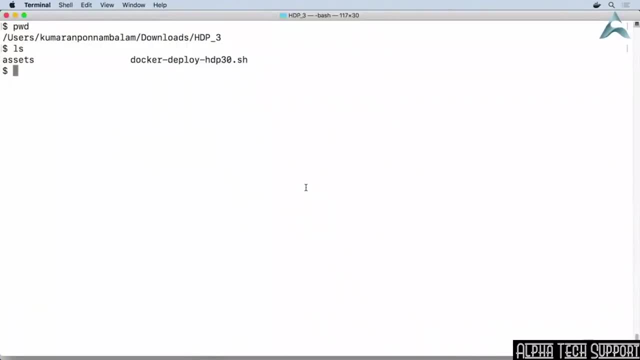 then please increase your RAM allocation. I have already downloaded the installation package and unzipped it in this specific folder. Before you move forward, please update your ETZ host file to add sandbox http to 127.0.0.1.. Now we can proceed to install the sandbox. 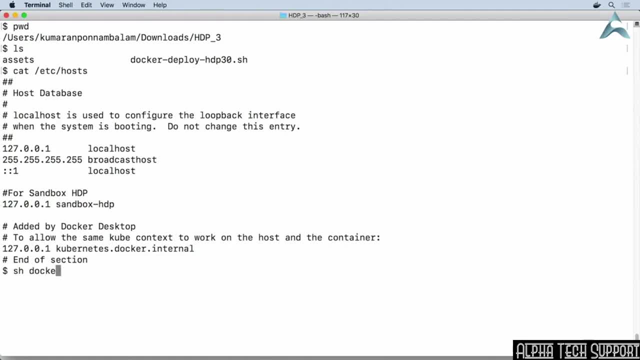 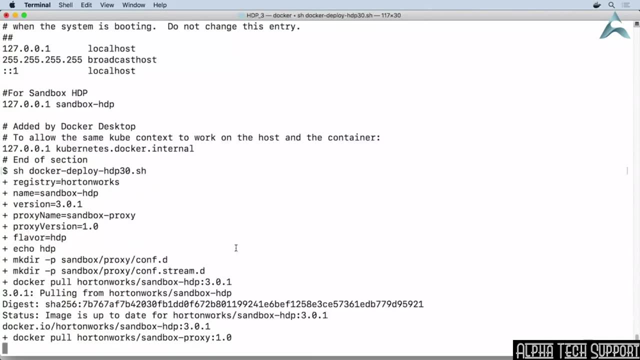 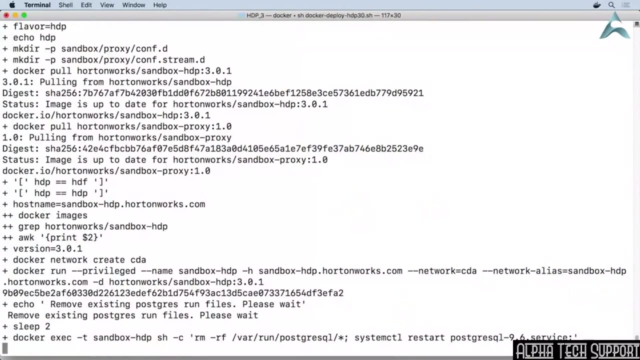 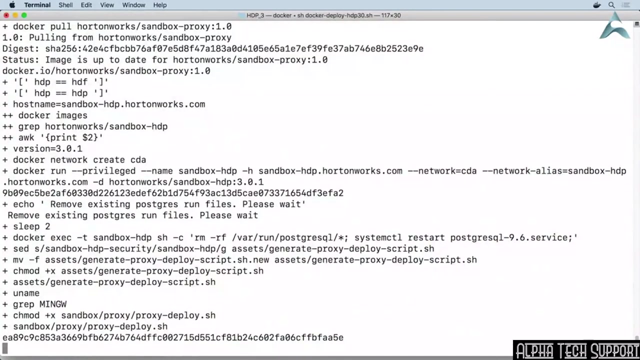 We can do so by executing the command sh docker deploy-http30.sh. It will install two docker images. sandbox-http is the main image that runs all the software. sandbox-proxy is a reverse proxy that is required for the main image to work. The installer will also start both the containers. 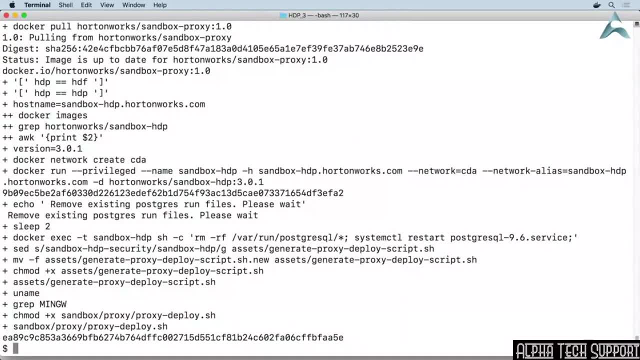 Please note that they are already in my local docker repository so it's skipping the docker pull step. The images are huge so the pull may run into many minutes. The containers usually take some time to start up, say 30 minutes to start all the services. 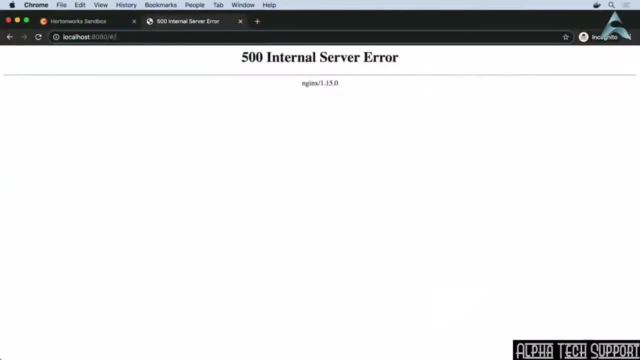 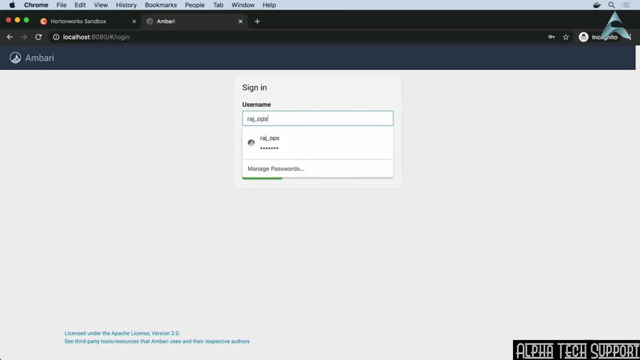 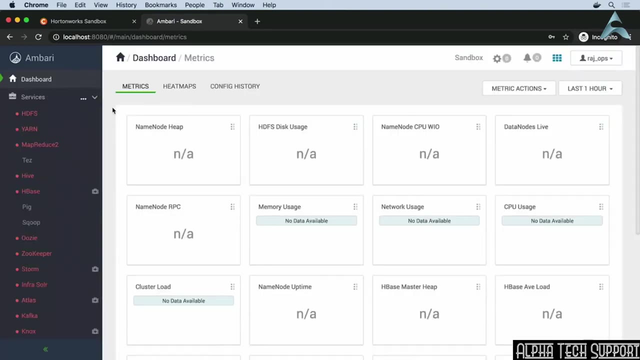 Please check the status of the services by visiting the page localhost 8080.. You can log in using the account raj-ops with the password raj-ops. again, This ambari dashboard shows the status of the service. You can see the status of all the services installed and most of them will be in the. 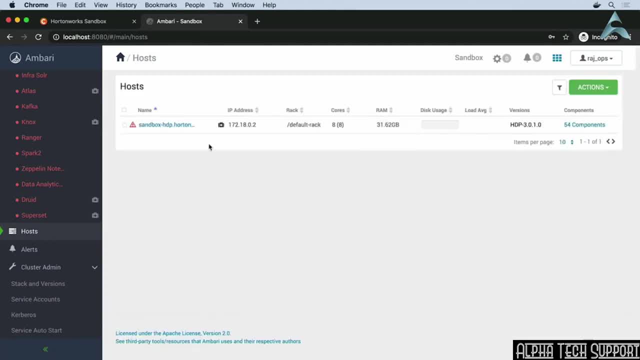 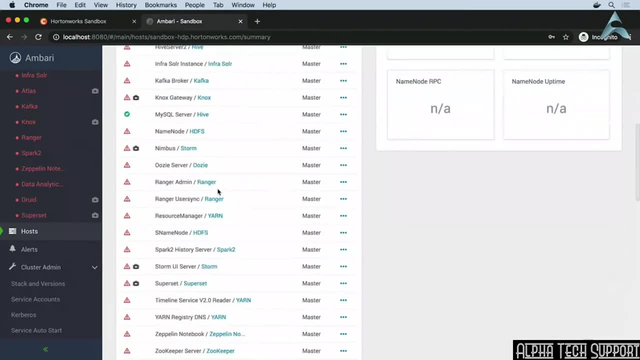 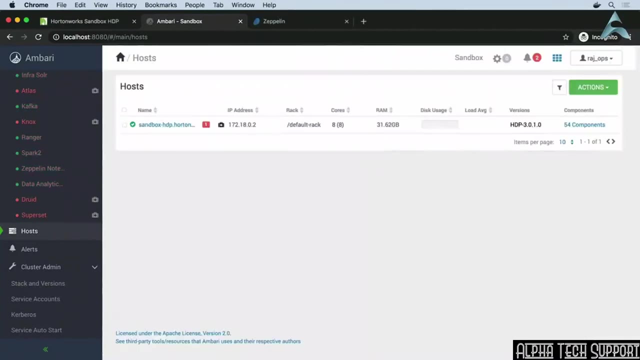 starting state. Go to hosts and click on the hosts link. here You will notice that the services are in starting state for most of the time, so give it about 30 minutes for all the services to come alive. In this video, I will show you the steps to set up the exercise files. 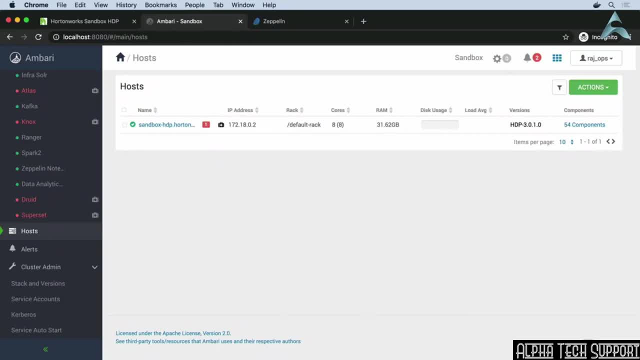 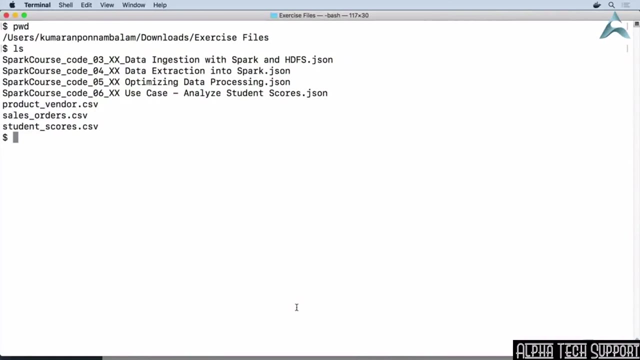 Before we go there, let's make sure that the sandbox is fully installed. We can do so by checking the host link in the ambari UI. Please make sure that the green checkbox shows up for the host. Next, I have downloaded the exercise files for this course in this directory. 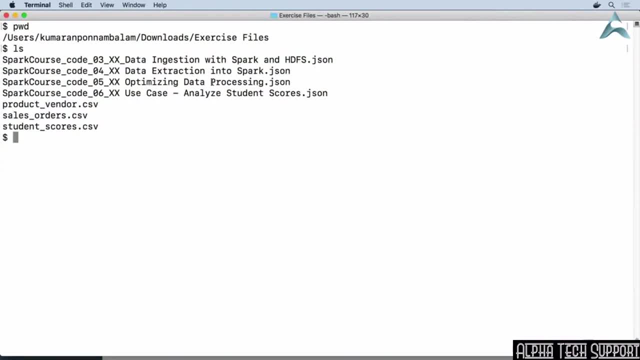 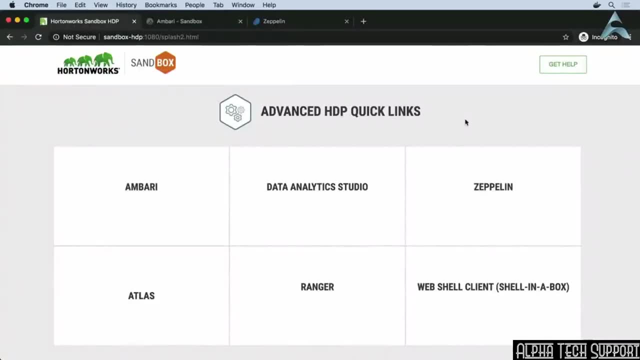 It has 3 csv files, which are data files, and 4 json files, which are zeppelin notebook files. Let's now load them into the setup. Go to the Hortonworks landing page on port 1080.. This shows all the application UIs available. 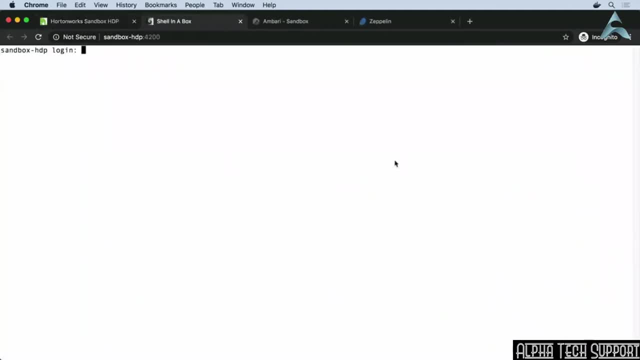 Go to the shell client available here. Login as raj underscore ops with the password as again, raj underscore ops. We want to provide full access to the rajops directory in HDFS to all the users. We can do so with the following command: htfs, dfs, mysql. 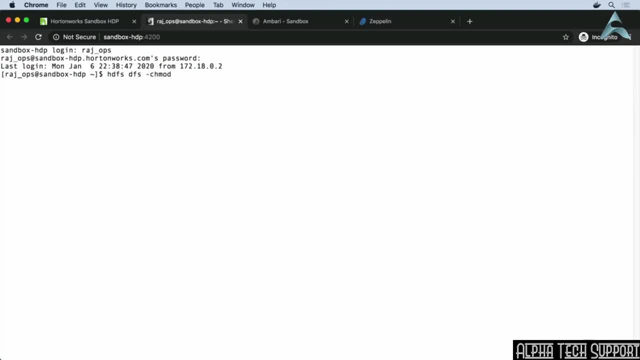 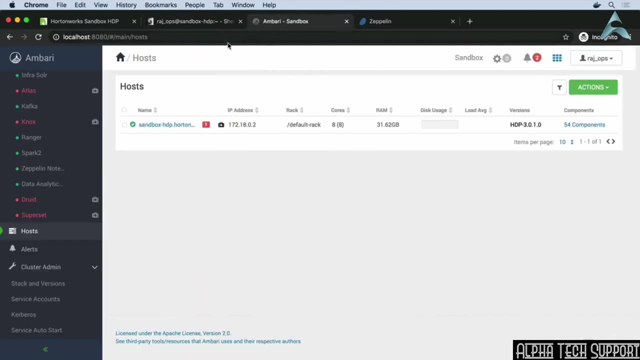 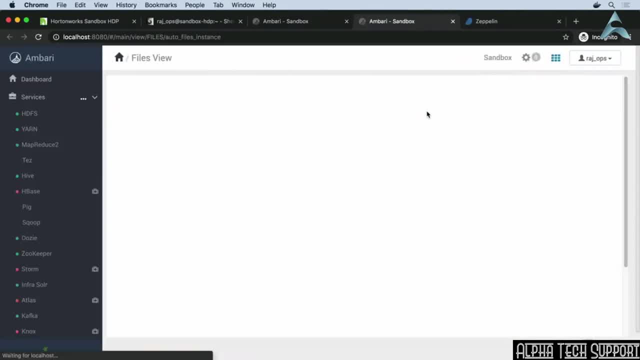 Click on files view to open the viewer for HDFS files. This shows all the HDFS human contract for lag When we click fast forwarded files in ourencia window, he will not get what we just recorded. This files view can be seen in aspects of volunteers: team members. 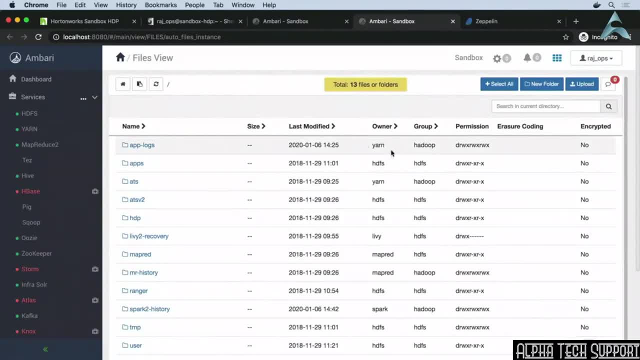 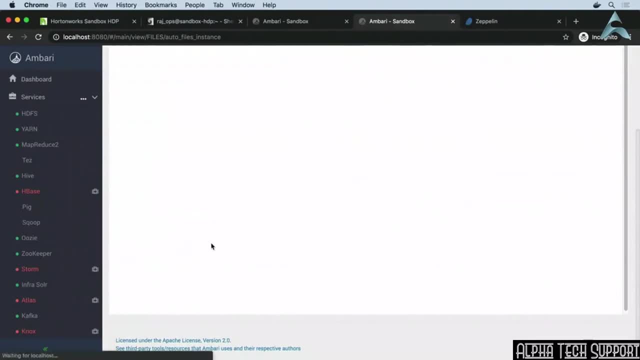 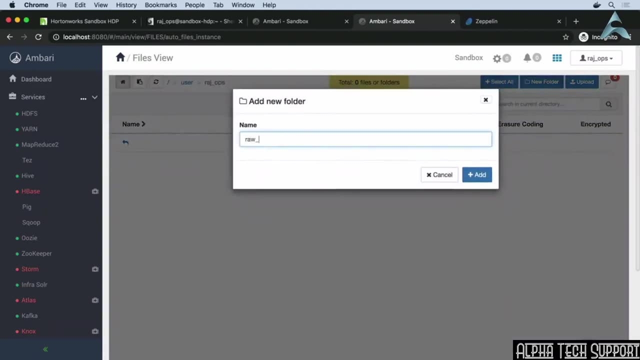 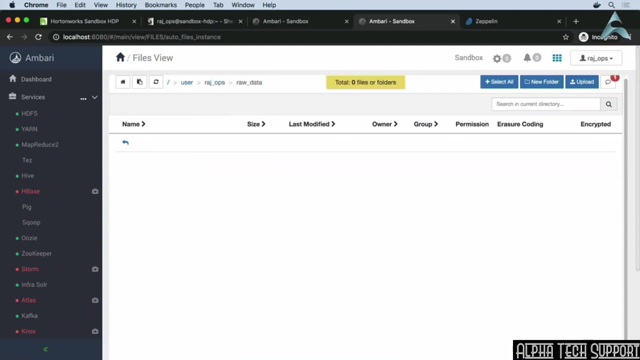 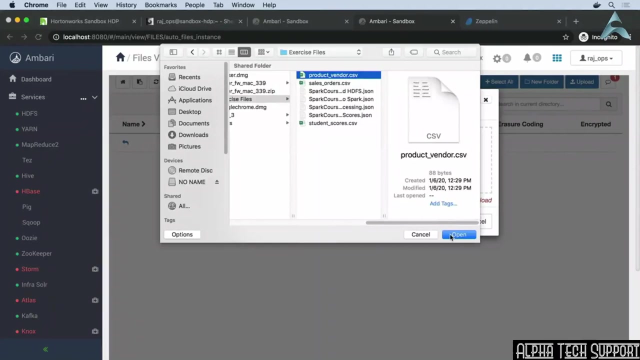 htfs directories available inside this instance. Navigate to the user rojobs directory. You can create a new folder here called raw underscore data. Navigate to the raw data folder Now. upload all the three csv files we have in the exercise files to this folder. 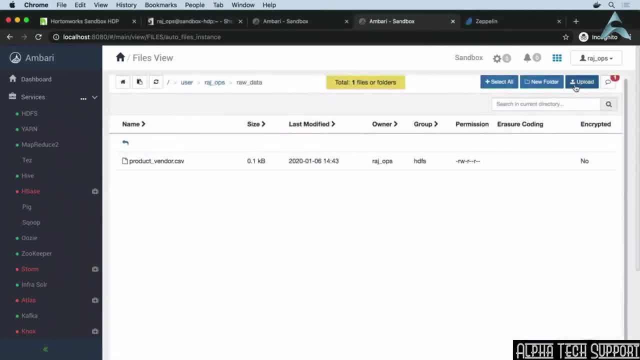 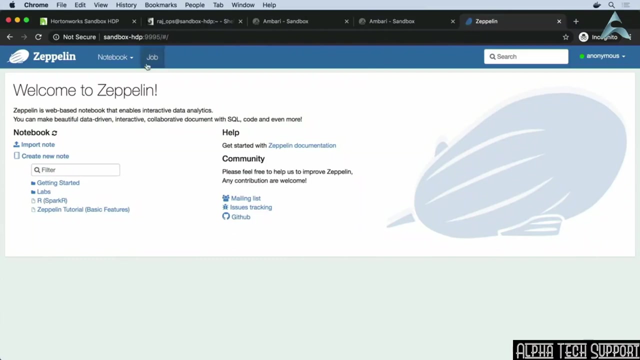 We first load product vendor- dot csv, Then we load sales orders- dot csv And finally we upload students course dot csv. Verify if the uploaded files show up in the folder correctly. Next we go to the zeppelin notebook. The zeppelin notebook runs on port 9995 on the sandbox. http website. 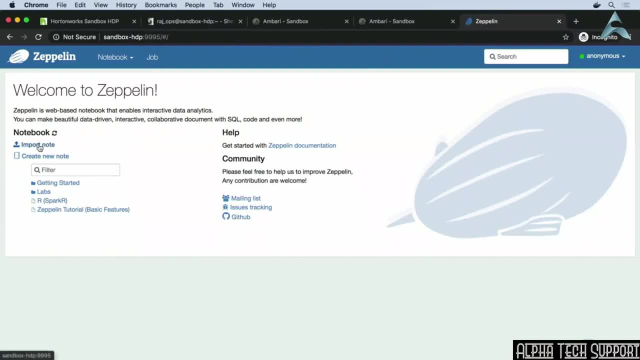 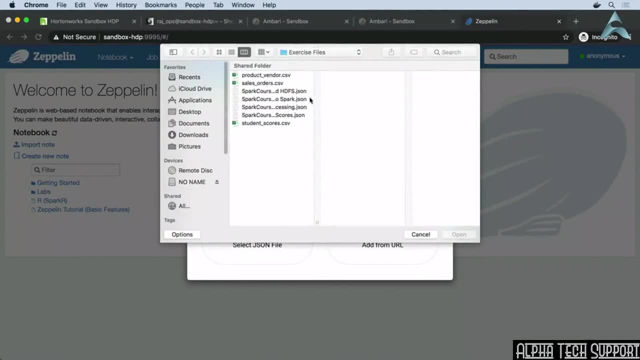 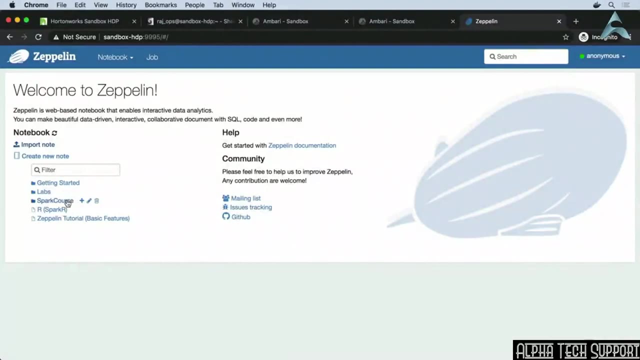 We first want to import all our exercise notes. So click on the import note link. Click select a json file. Now upload each of the json files one by one. The json files will start showing under download. Next we go to the zeppelin notebook. 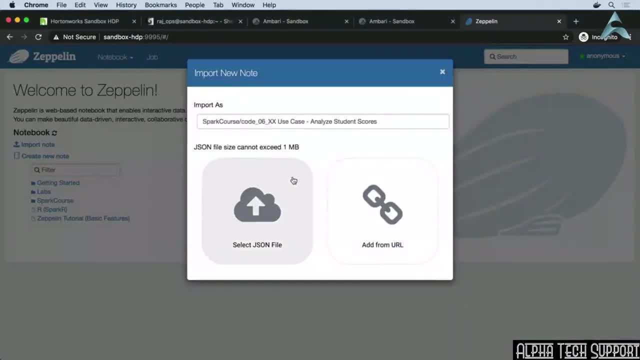 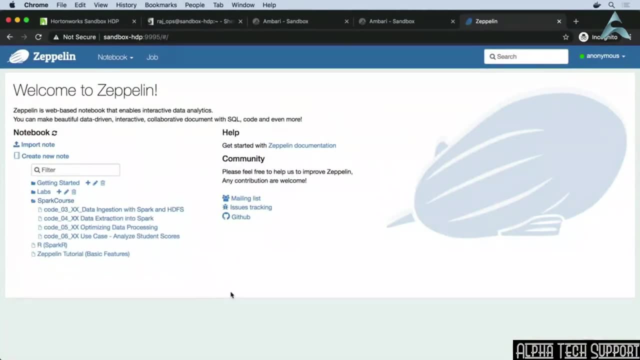 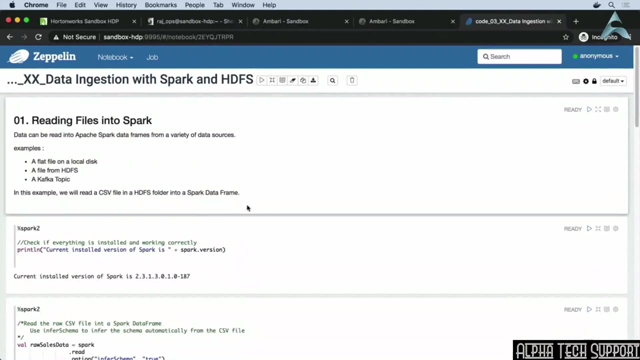 The zeppelin notebook runs on port 9995 on the sandbox http website. We first load product vendor dot csv, Then we upload all the products into it. We command to print the current version of spark. click on the run paragraph button here now. this should immediately run and print the version of spark. typically when you run spark. 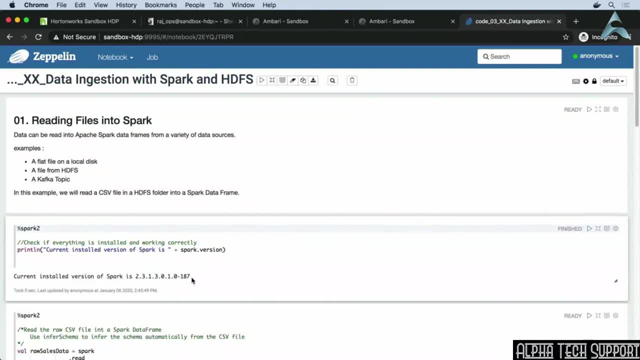 for the first time, it may take some time, even a couple of minutes, for the first command to run and successfully come back. this is perfectly okay. you just have to be patient for the command to execute. this confirms that our setup is up and running and now we can start using it for our 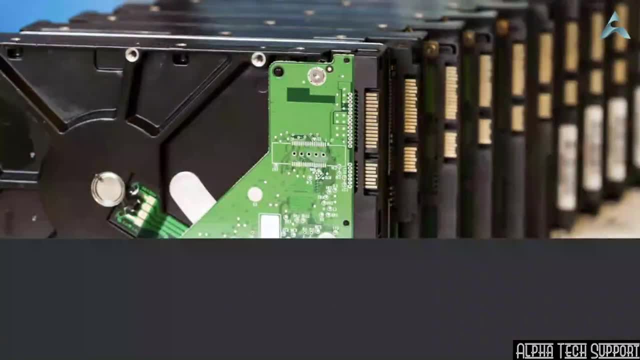 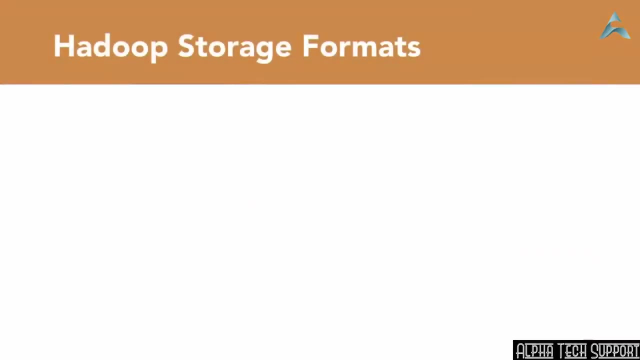 course. in this chapter i will review various options available and best practices to store data in hdfs. i will start off with storage formats in this video. hdfs supports a variety of storage formats, each with its own advantages and use cases. the list includes raw text files. 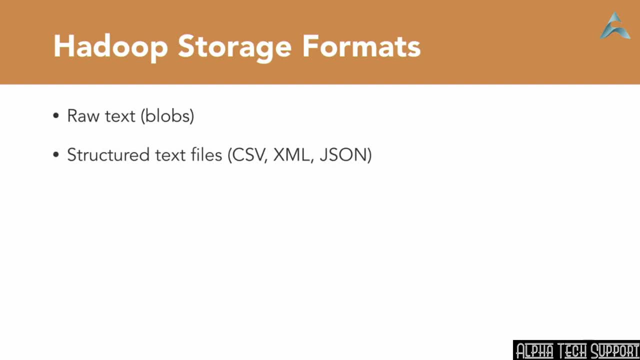 hdfs supports a variety of storage formats, each with its own advantages and use cases: structured text files like csv, xml and json, native sequence files, avro formatted files, arc files and parquet files. i will review the most popular ones for analytics now. text files carry the same format they have in a normal file system. they are stored as a single physical file in hdfs. 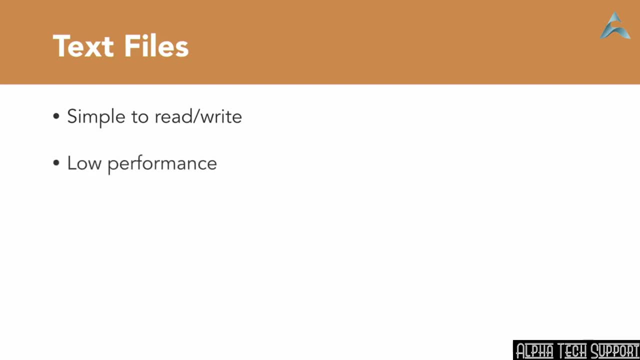 they are of low performance as they do not support parallel operations. they require more storage and do not have an enforced schema. in general, they are not recommended. avro files support language neutral data serialization, so data returned through one language or tool can be read with another with no problems. data is stored row by row. like csv files, they support a self. 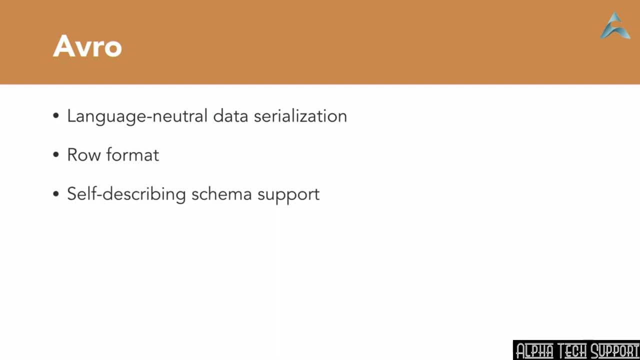 describing schema and is used to enforce constraints on data. they are compressible and hence can optimize on storage. they are split double into partitions and hence can help in parallel reads and rights. they are ideal for situations that require multi-language support. parquet files store data column by column, similar to columnar databases. this means each column can. 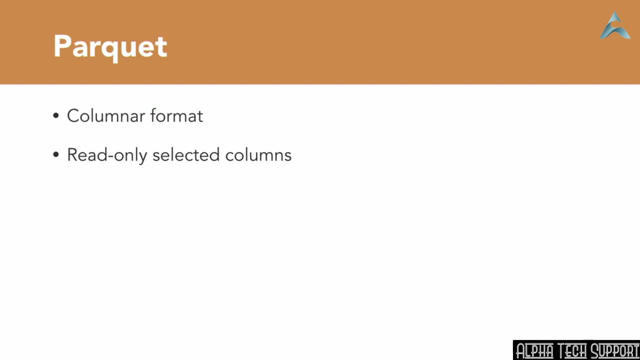 be read separately from disk without reading other columns. this saves on i? o. they support schema. parquet files are both compressible and splitable, and these are should be used for running the per Plus string sequence and, since these are also available for you to plug into your mobile. 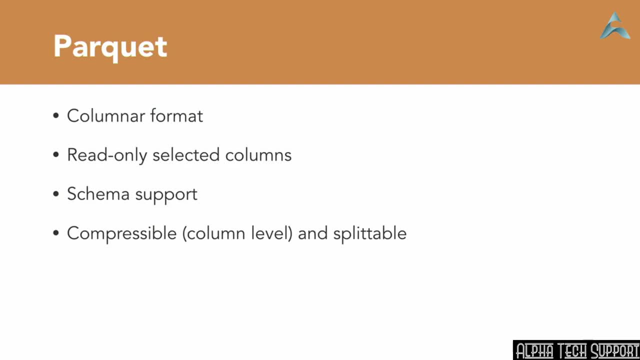 and hence are performing a lot of work with this program. we grease the hell out of each other if you performance and storage optimized. They also can support nested data structures. Parquet files are ideal for batch analytics jobs for these reasons. Analytics applications typically have data stored as records and columns. 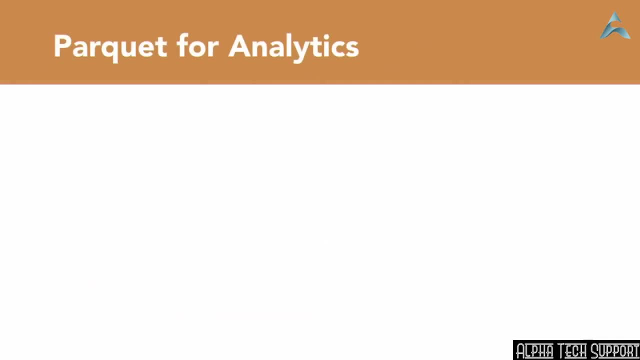 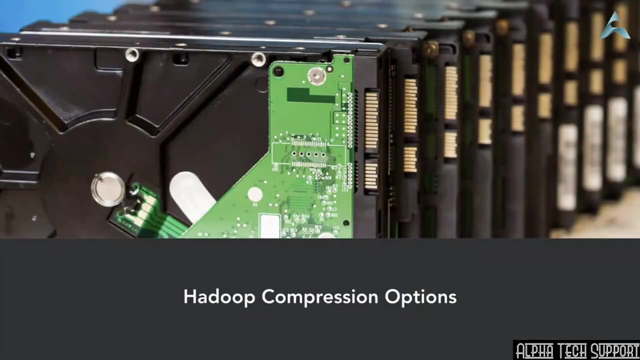 similar to RDBMS tables. Parquet provides overall beta performance and flexibility for these applications. I will show later in the course how Parquet enables parallelization and IO optimization When storing big data. compressing data is important as it saves significant disk space and hence reduces operational costs. 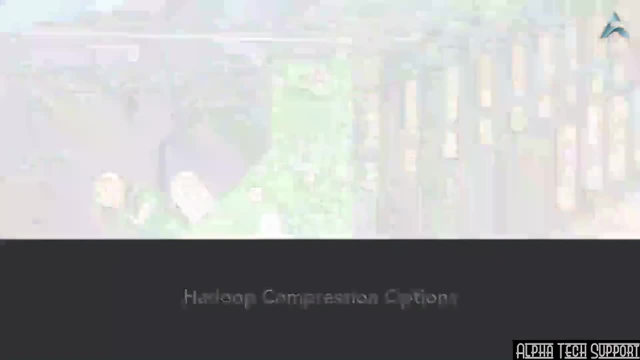 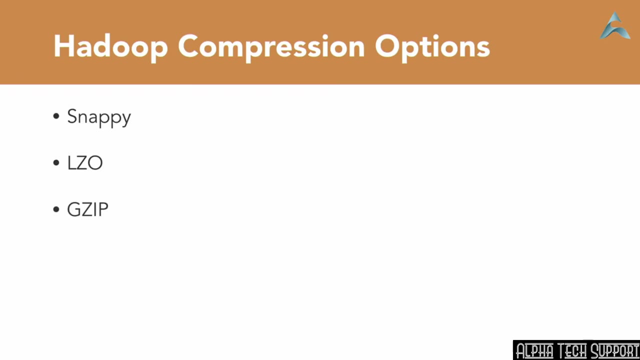 In this video, I will review the various file compression options available. The most popular compression codecs available are Snappy, LZO, Gzip and Bzip2.. You can also develop your own codec if required. Snappy is a compression codec developed by Google. 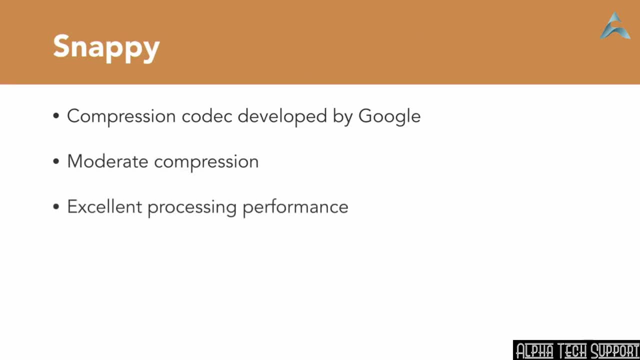 It provides moderate compression but excellent read-write performance. Snappy compresses the entire file, as opposed to compressing it element by element. It is not splittable and hence not suitable for parallel operations. LCO is similar to Snappy in that it provides moderate compression and excellent processing performance. 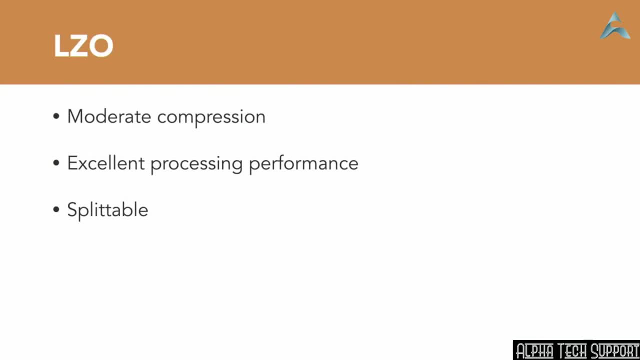 It can also be used to split files and hence has an advantage with parallel processing, But it requires a separate license that needs to be carefully evaluated for possible costs. G-SIP is a popular codec that provides very good compression, It has moderate read-write performance and it is not splittable. 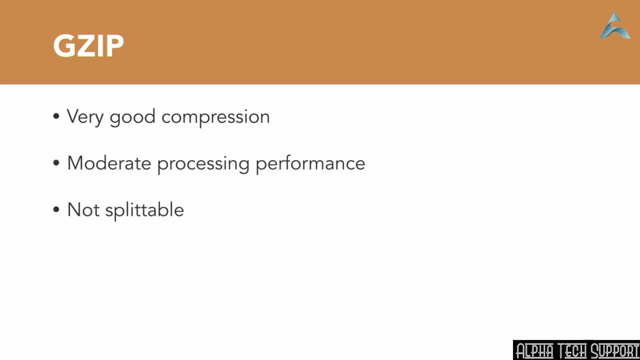 It combines well with Parquet, where each column can be individually compressed within a partition where splitting is not needed. Hence it is suitable for analytics applications, especially when combined with a partition. G-SIP2 is another codec that offers excellent compression but slow read-write performance. 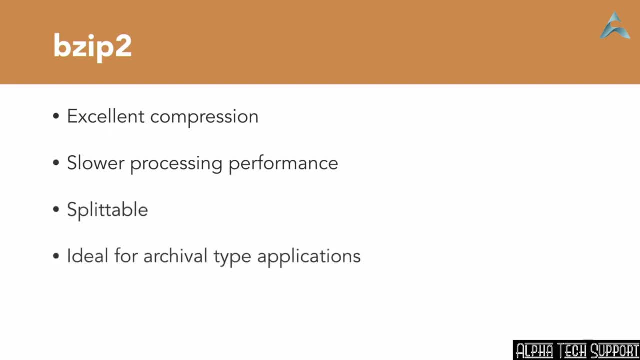 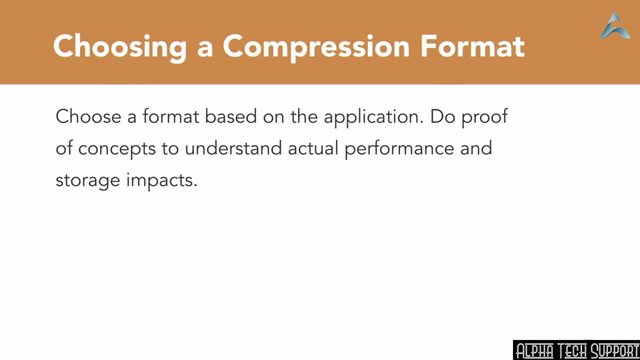 It also supports splitting. It is ideal for data archival type of applications, where data is written once for archival or backup cases and rarely read back. Choose a compression format based on the type of application and the expected access patterns for data. It is recommended to do proof-of-concept projects. 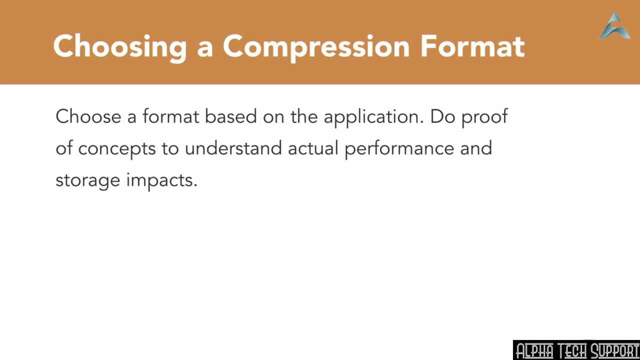 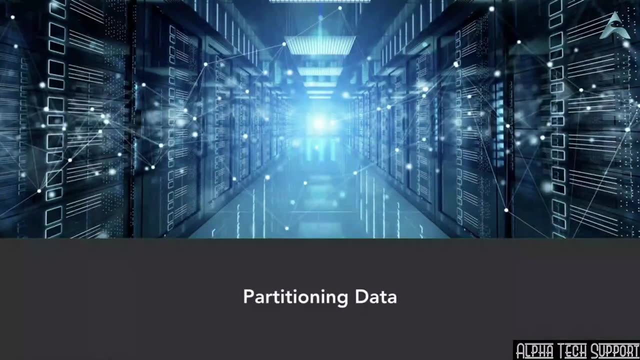 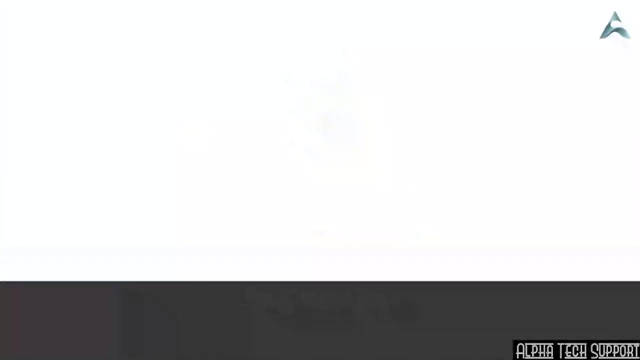 to understand the actual impact of codecs on both storage and processing, based on the specific use case. Partitioning is a key concept to use while working with HDFS data. In this video, I will review the importance of partitioning and how it works. 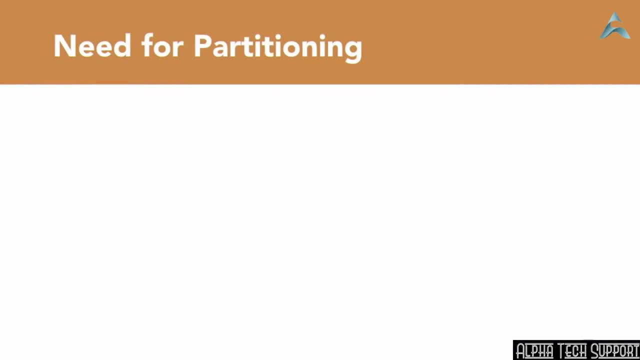 Why do we need partitioning Relational databases? speed up data access by using indexes on columns used in filtered conditions. HDFS does not have the concept of an index. Even if a single row is required from a large petabyte file, the entire file should be read to extract the record. 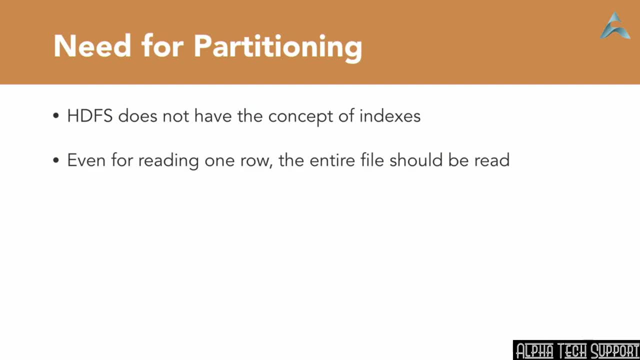 This introduces significant disk IO and delays Partitioning. provides a way to read only a subset of data based on a partition key Similar to indexes. partitions can also be based on multiple attributes. Typical attributes suitable for partitioning include dates and entries for information to be read. 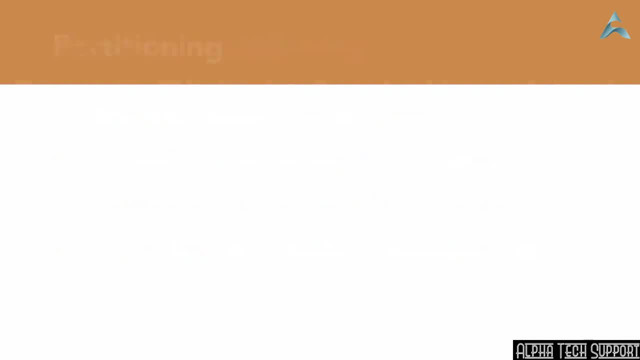 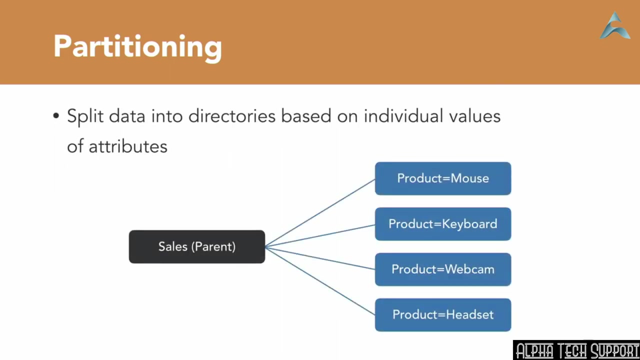 element identifiers like customer or product names. How does partitioning work? When we create a HDFS file specifying a partition key, Hadoop creates a separate directory per partition. Records corresponding to a specific partition key is stored in the same directory. For example, if we use product as a partition key, a separate directory will be created. 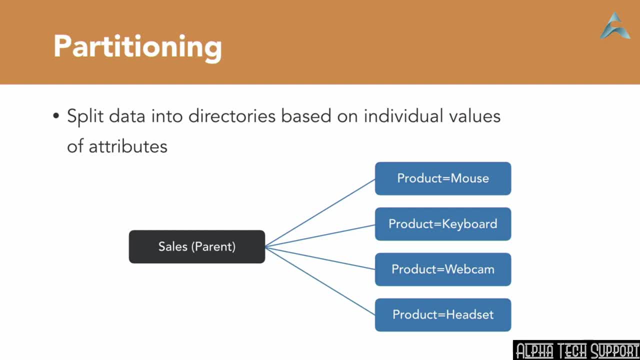 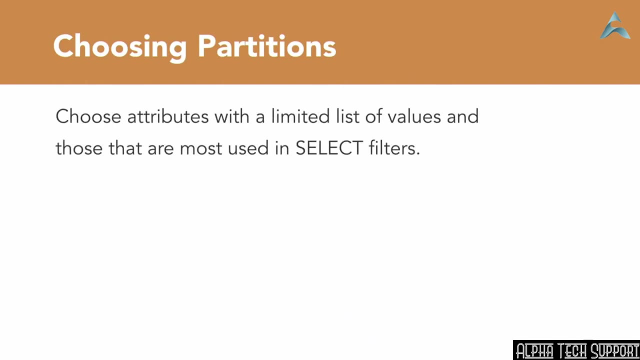 for each product and corresponding records will be stored there. If we use a filter on the product attribute, while querying, only those subdirectories that match the filter need to be read. While selecting attributes for partitioning, choose attributes that have a limited or controlled. 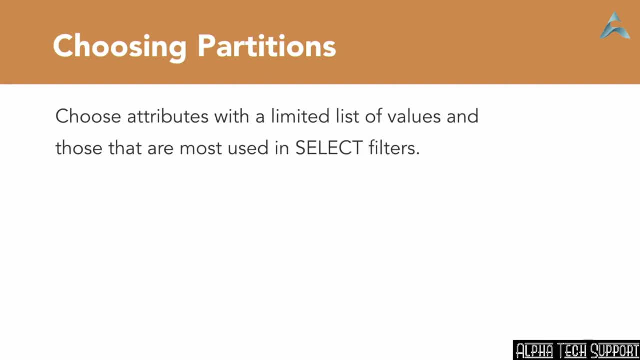 set of values. Otherwise, too many subdirectories might be created. Also, ensure that the records are equally distributed among the various values. Choose attributes that are most used in query patterns. Likely, candidates include dates, customer IDs, product IDs, among others. 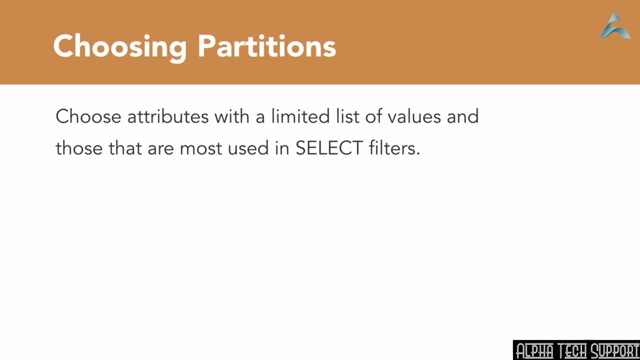 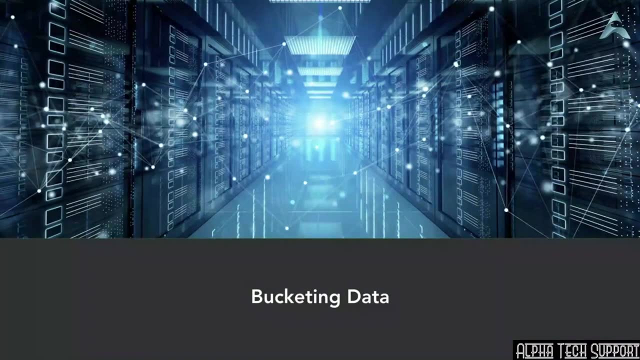 In the next video I will discuss an alternative to partitioning, called bucketing. As seen in the previous video, partitioning is only optimal when a given attribute has a small set of unique values. What if we need to partition for a key with a large number of values? 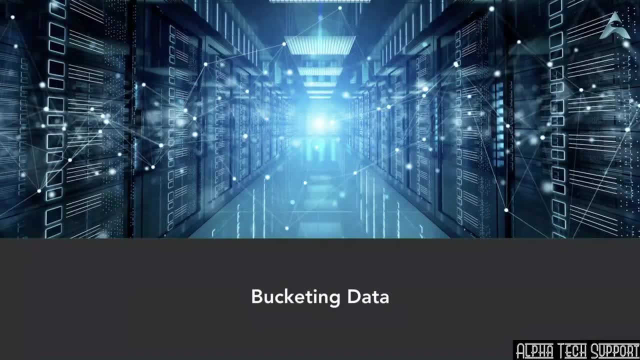 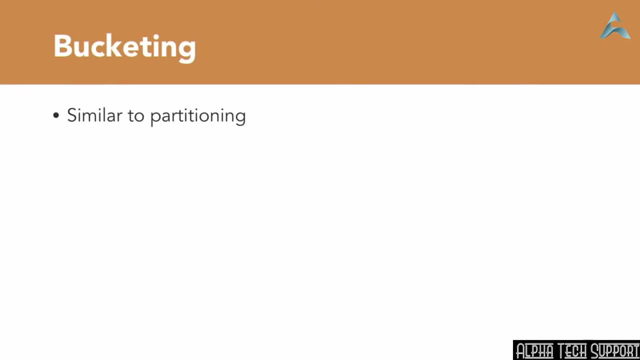 What if we want to keep the same number of values within the same directory? I will discuss this in a later video. Bucketing works similar to partitioning, But instead of using the value of the attribute, it uses a hash function to convert the value. 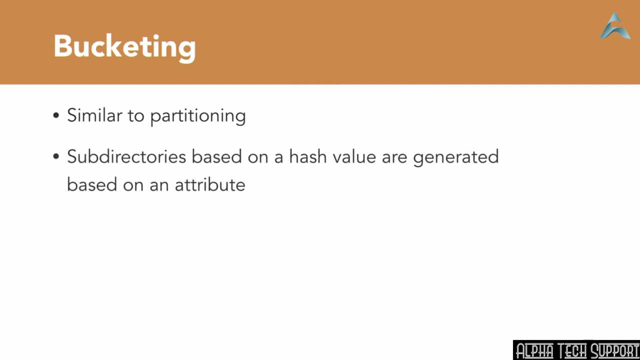 into a specific hash key Values that have the same hash key end up in the same bucket or subdirectory. The number of unique buckets can be controlled and limited. This also ensures even distribution of values across all buckets. It's ideal for attributes that have a large number of unique values, like order number. 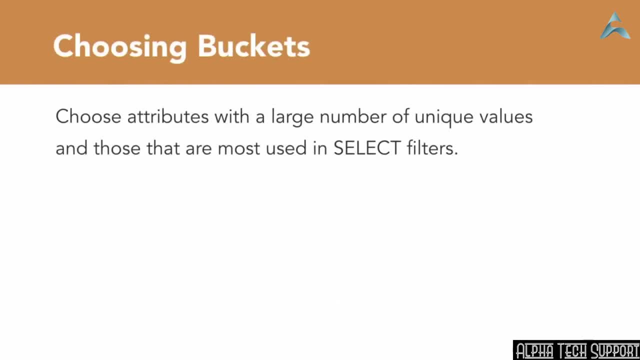 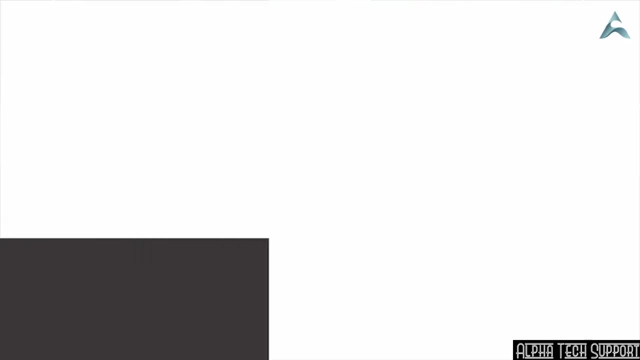 or transaction ID. Choose buckets for attributes that have a large number of unique values and those that are most frequently used in query filters. Experiment with multiple bucket counts to find optimal read-write performance for the specific use case. In the next video, I will review some best practices for data storage. 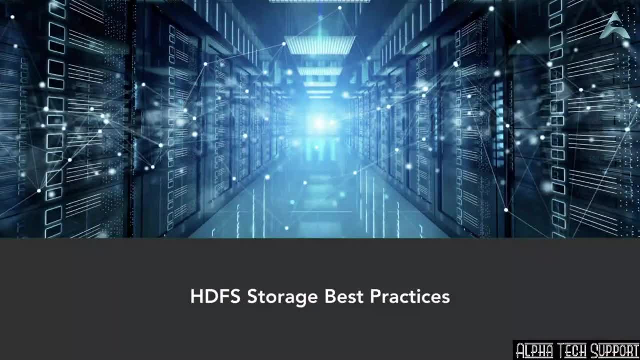 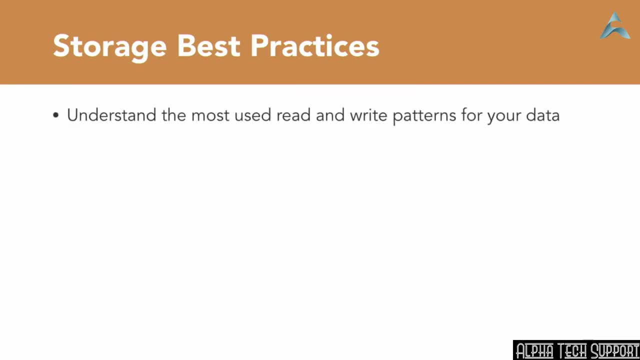 In this video I will walk through some of the best practices for designing HDFS schema and storage. First, during the design stage, understand the most used read and write patterns for your data. Identify if it's read-intensive or write-intensive or both. 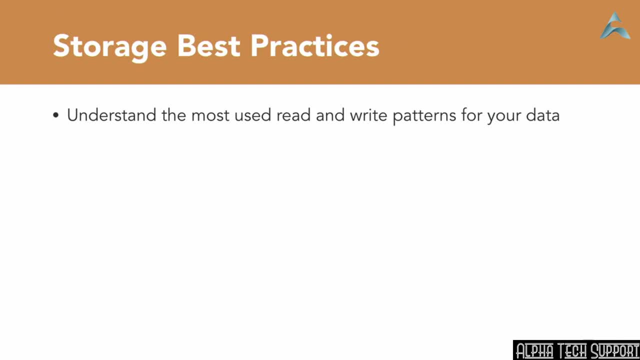 For reads. analyze what filters are usually applied on data. Determine what needs optimization and what can be compromised. Is it important to reduce storage requirements or is it okay to compromise on storage for better read-write performance? Choose your options carefully, as these cannot be easily changed after the pipeline is deployed. 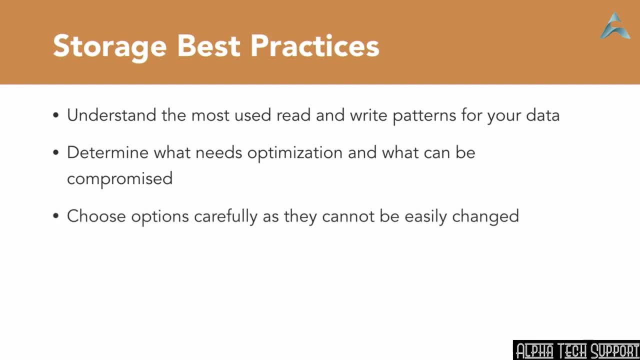 and data is created. Changing things like storage formats and compression codecs would require reprocessing all the data. 3. data to understand performance and storage characteristics. Experiment, if required, to compare between different storage options available. Choose partitioning and bucketing keys wisely, as they incur significantly additional. 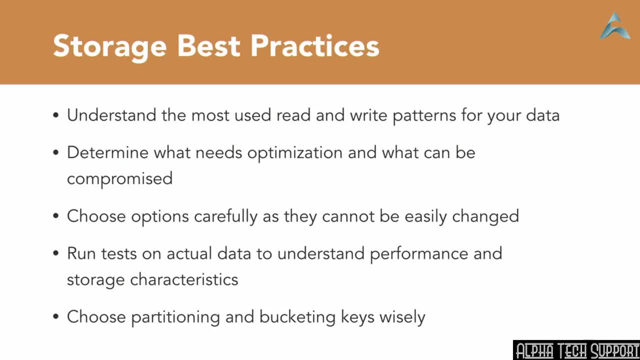 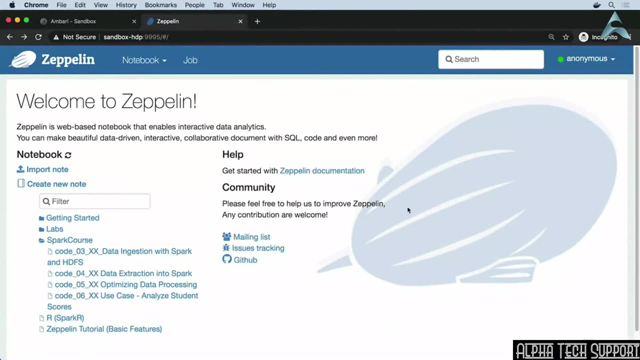 costs during writes while helping in reads. In the next chapter, let's start reading and writing HDFS files with Spark using these practices. In this chapter, I will demonstrate options available to ingest data into HDFS with Spark. We will be using the Zeppelin notebook titled code underscore. 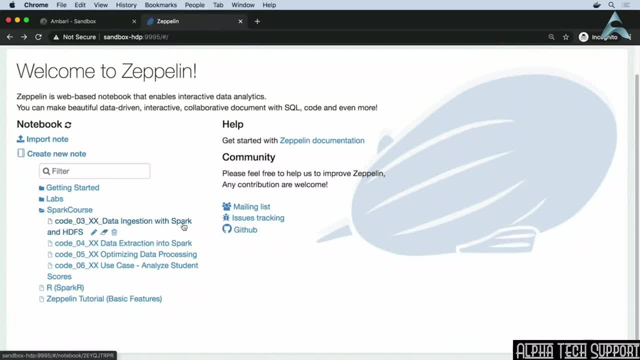 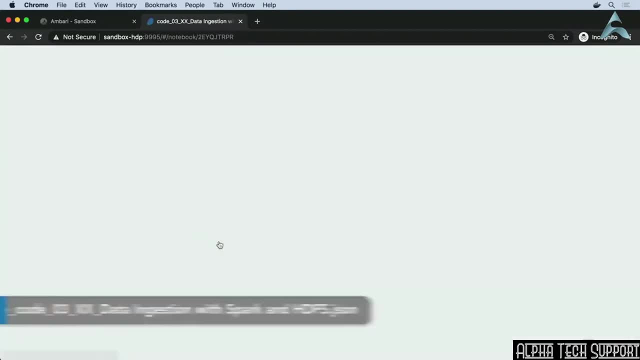 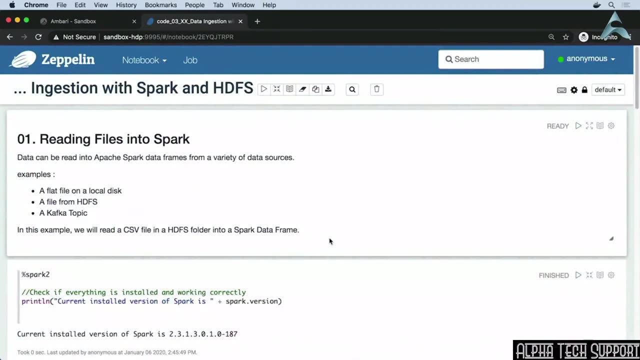 O3 underscore XX. data ingestion with Spark and HDFS. Navigate to this notebook at sandbox hyphen HTTP 9995.. On opening the notebook, you will find that Zeppelin is similar to Jupyter notebooks in many ways. We can create paragraphs, each with a different interpreter. The code can be: 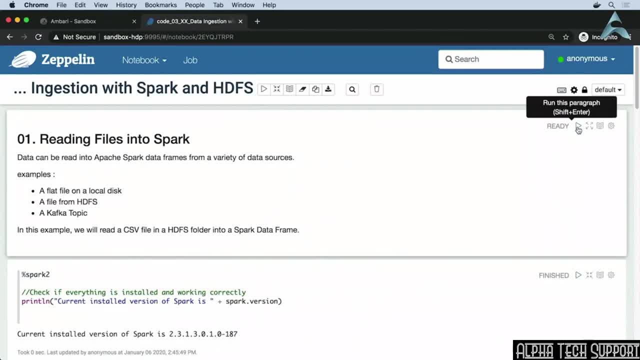 executed by clicking on the run button. Results will display immediately below the paragraph. In this video, we will focus on reading external data into Spark. Spark provides connectors to a number of external data sources, including a local file, a file from HDFS or even a kafka topic. The first. 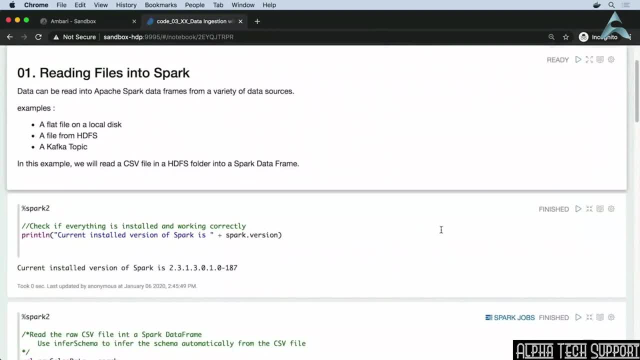 Next paragraph here is to test if Spark is successfully installed, and running The %spark2 in this first line indicates the interpreter to use. We can run this paragraph with the run button and the results will show up in the bottom. We see that the current version of Kafka is showing up correctly, so we are good to proceed. 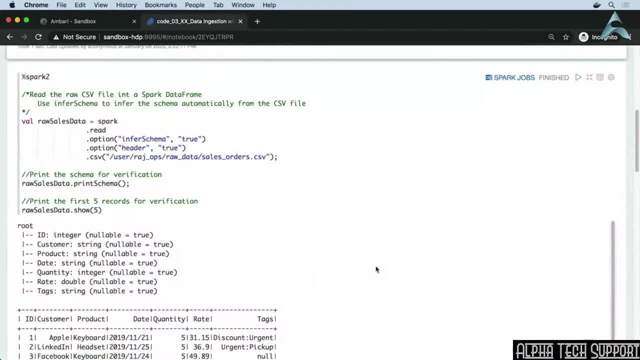 with the other exercises. In the next paragraph we read a CSV file. Since Spark is running under YARN in the sandbox, it uses HDFS as its disk. We will read the sales-orderscsv file that we uploaded earlier in the course into a data. 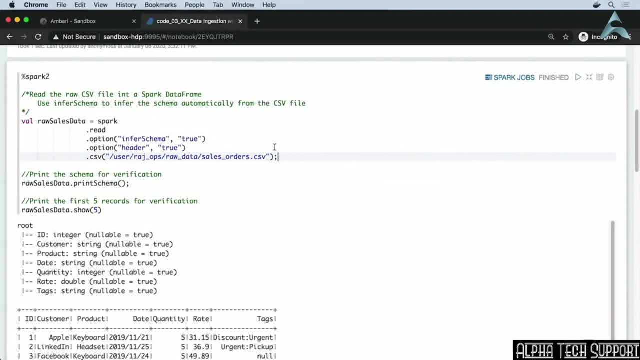 frame called raw-sales-data. We set the option for header to tell Spark to consider the first line of this file as the header. We also specify: infer schema equal to true. Spark will examine the first few lines in the file to infer the data type of each column. 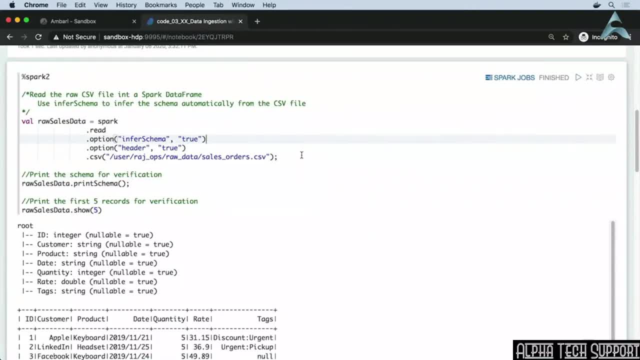 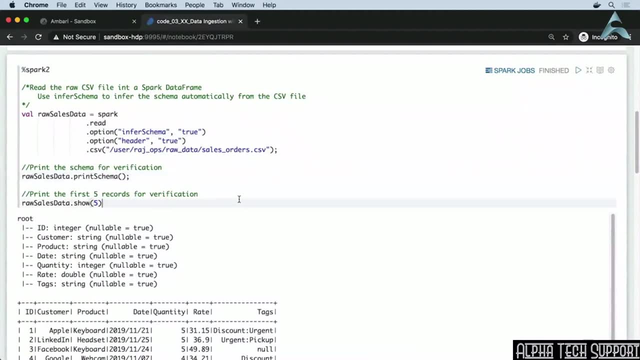 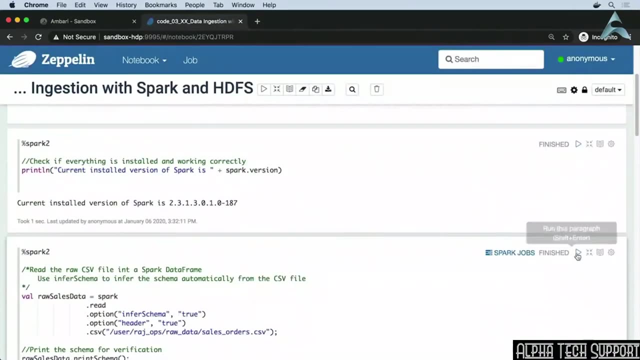 It will also use the header line to name the individual columns. We then print the schema for this data frame, as well as the first five rows, to make sure that the data is read correctly. Let's run this code now and review the results. We can see that the schema, as well as the data, shows up as desired. 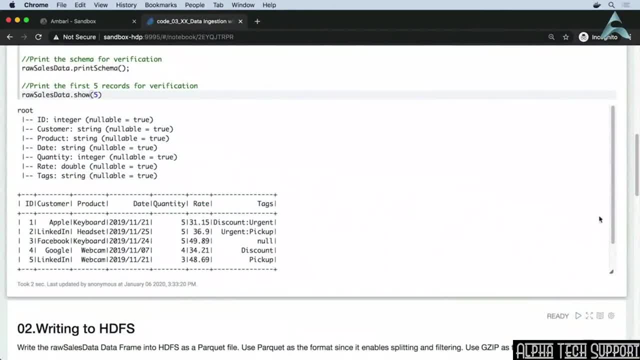 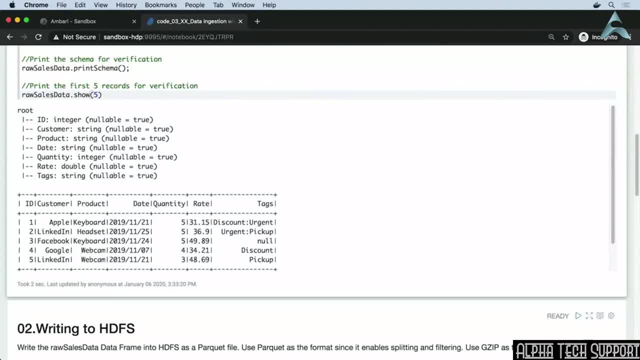 And, lastly, I will show you how to previously process change in the schema. Finally, we need to talk about тайma, where I was trying to like compel us to validate it if you are familiar with it, But in this video we already, fellows, learnt about that. 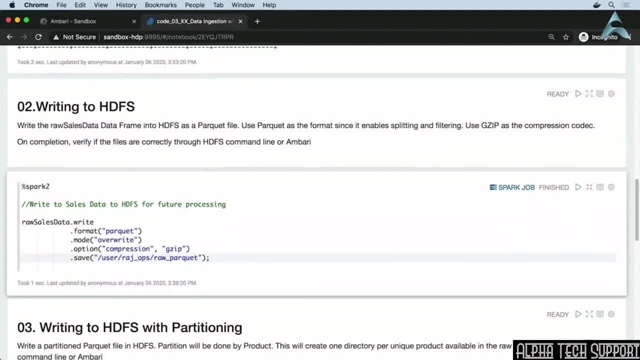 I hope it will be entertaining for you And, as discussed in the previous videos, CSV filetać not be used for parallel reads and writes. We need to convert demais to other formats like parquet for efficient processing of data in the later stages. 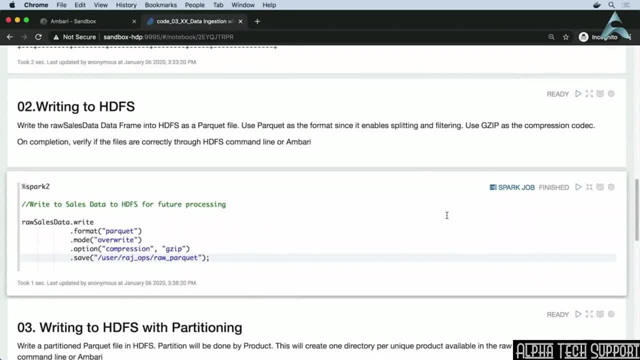 In this video we willt write the raw sales data data frame into a parquet file in HDFS. The code for this is MagnusXласти. There are VMs without disks. It will download the files from TMD database. iz class означates that there are pharmacy saved in дрfs distribution. 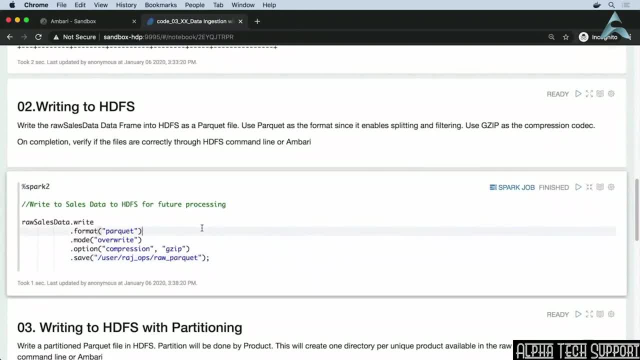 The code for this is simple. We will use the write function available in the data frame. We then set the format to Parquet. The mode is set to overwrite- to overwrite any existing contents In real pipelines, though append may be the better option if there are periodic additions to the data. 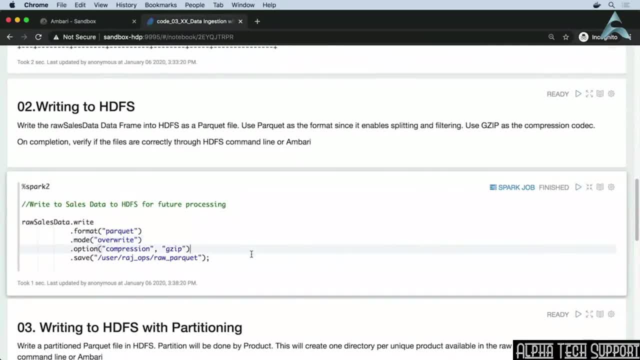 We then use gzip to compress the data. We save it to the raw Parquet directory under user slash raj, underscore ops. Let's execute this code and review the results. First, notice the Spark job feature appearing at the top of the paragraph. You can click on this to open the Spark UI and look at how Spark executed this job. 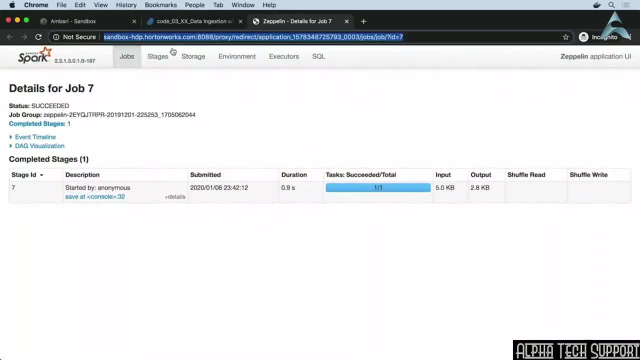 The Spark UI may launch with a fully qualified URL And this may generate a new job. You can overcome it by adding this URL to the ETZ host file. Here is how my ETZ host file is set up. We can also go to the HDFS file viewer to review the data that is created. 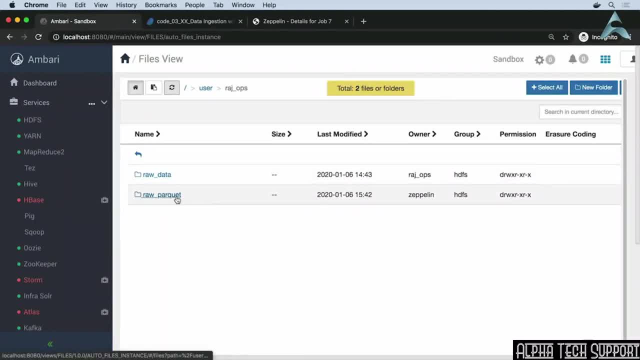 We can see a directory created called raw Parquet. If we go under that, you will see part files created under this specific directory and the extension shows that they are GC files of Parquet format. Depending on the size of the data, there could be more files that get created. 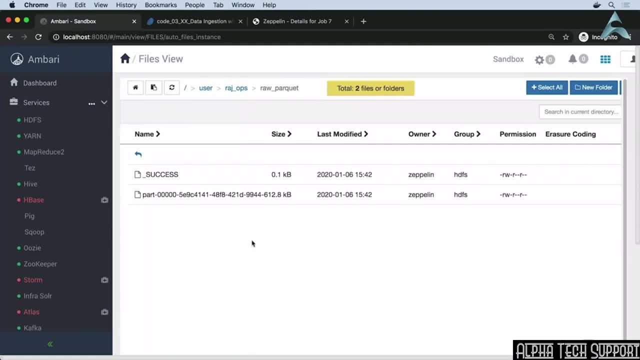 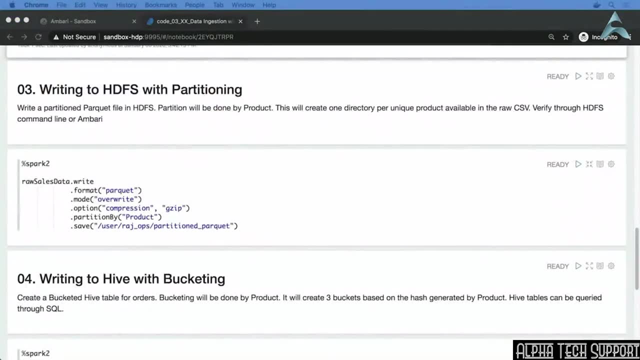 In the next video, I will show you how to partition data while writing to HDFS. As reviewed in the earlier videos, partitioning of data enables parallel reads and writes. It also helps in filtering of data while reading into memory. We will create a partitioned HDFS store based on the product column. 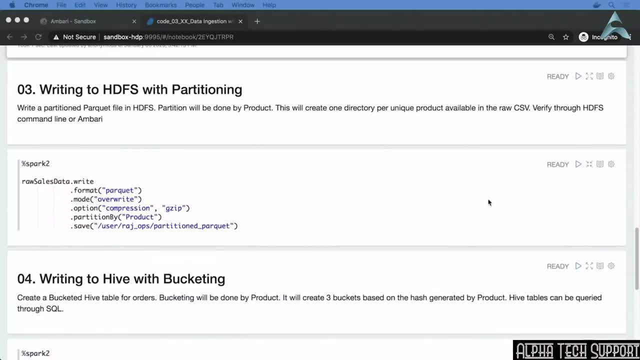 We will create a partitioned HDFS store based on the product column. There are only four unique products in the data set, so it lends itself to easier partitioning. There are only four unique products in the data set, so it lends itself to easier partitioning. 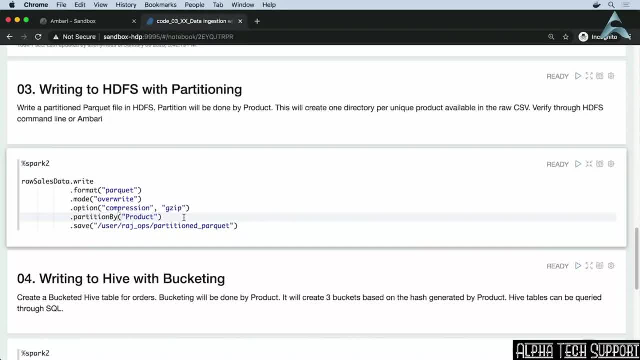 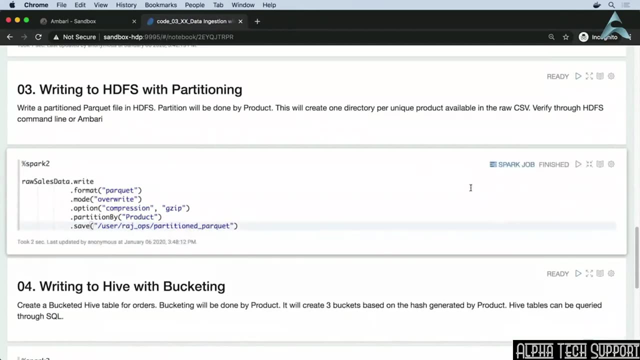 We simply need to add the partition by method in the write process to trigger partitioning while storing data. We then save this to the partitioned Parquet directory. Let's run this code and examine the HDFS files created. Let's go and look at the HDFS files. 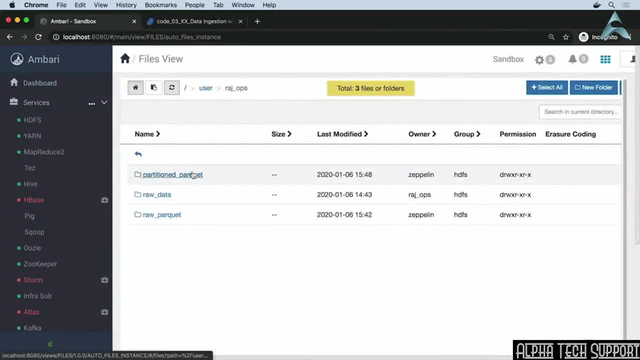 Let's go and look at the HDFS files When we navigate to the partitioned Parquet directory. When we navigate to the partitioned Parquet directory, we see four subdirectories created. we see four subdirectories created. They are one per partition. 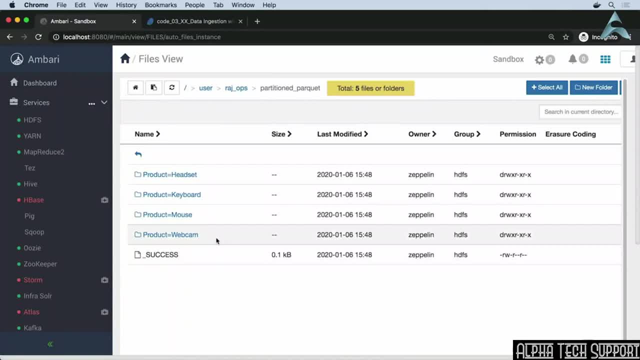 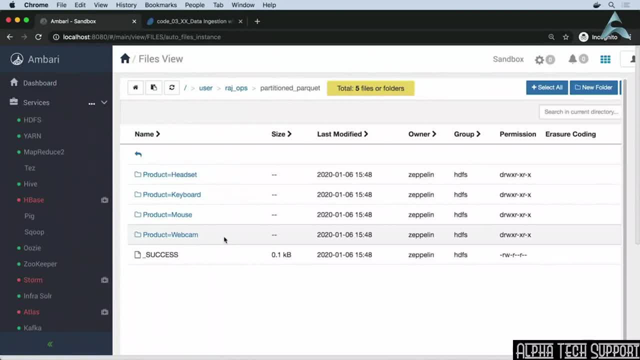 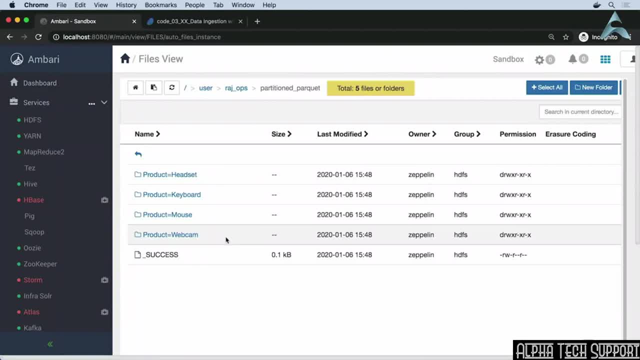 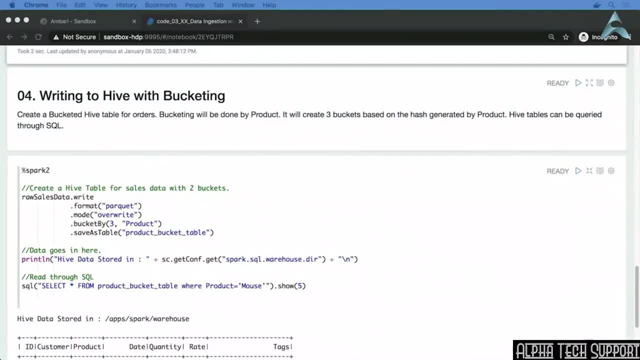 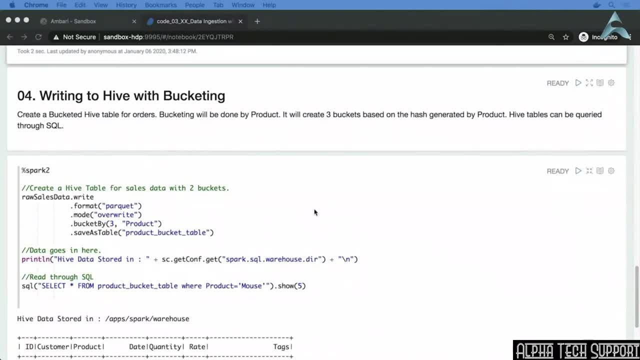 In this example, we will create buckets again based on the product column. In this example, we will create buckets again based on the product column. We will create three buckets. In order to do bucketing, we use the bucket by method. In order to do bucketing, we use the bucket by method. 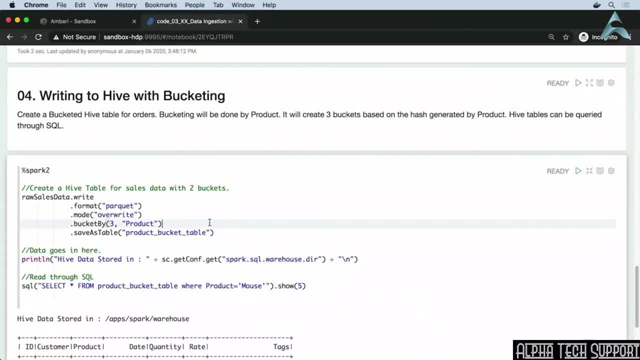 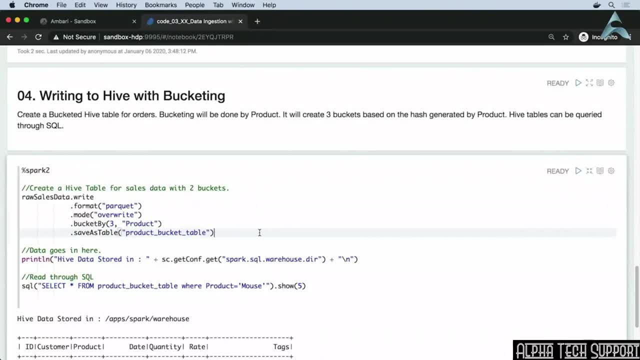 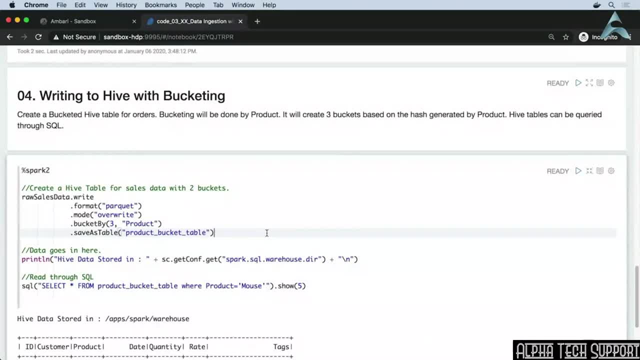 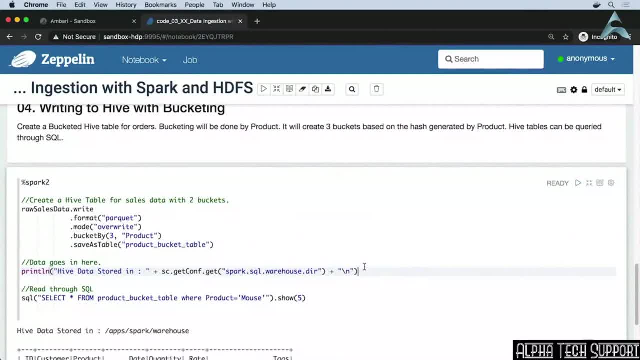 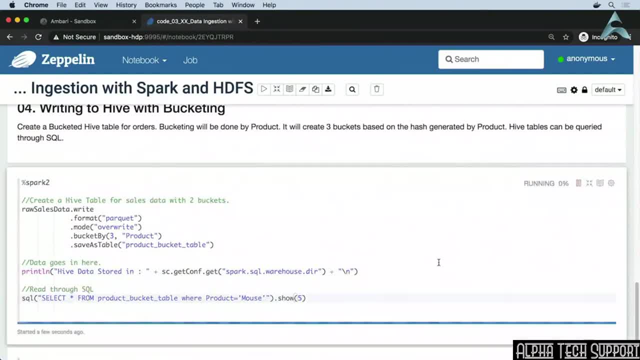 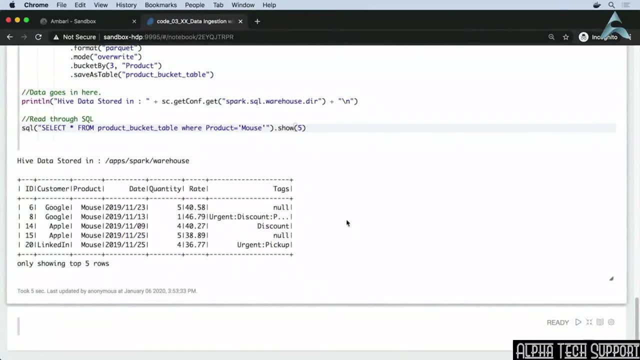 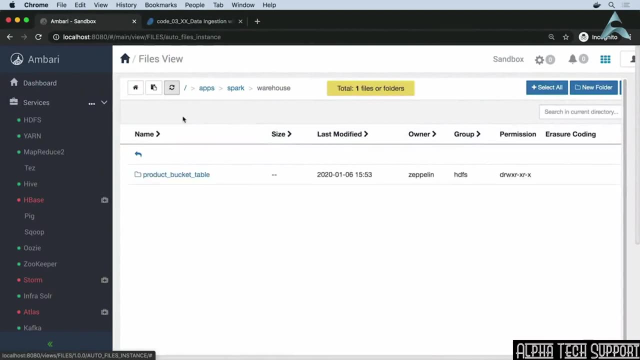 contents. Let's execute this code now. We see the contents printed correctly. We can go to the HDFS directory to examine the contents. The HDFS directory is apps, spark warehouse. We see the product bucket table created here. Navigating to this table, we see three parts. 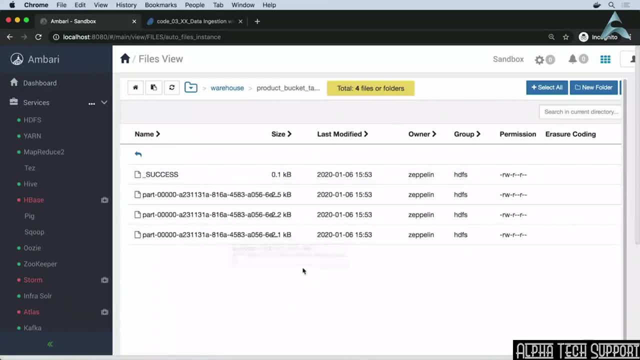 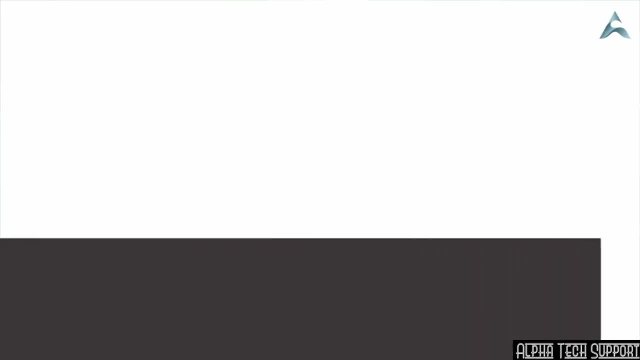 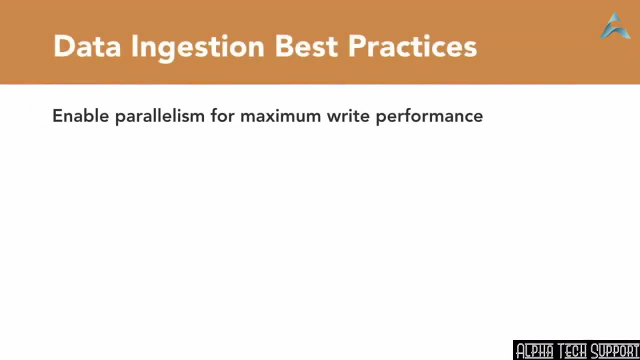 being created. They correspond to the three different buckets. In the next video, let us review some of the best practices for data ingestion. Let's review some of the best practices for data ingestion with Hadoop and Spark. Enable parallelism for maximum write performance. This can be achieved by using splittable file. 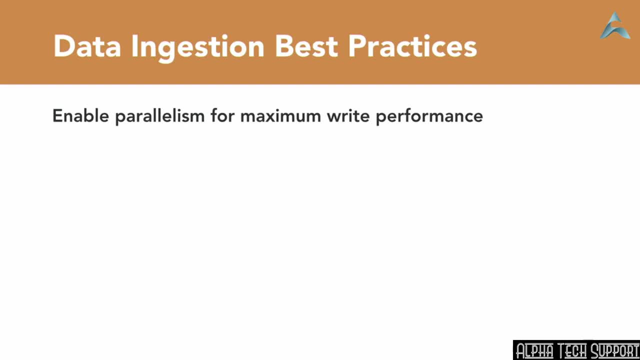 formats like Parquet and using partitions or buckets. When doing incremental data ingestion, use append. This will help optimally distribute the write loads to the data ingestion. While reading external data into Spark, prefer sources that can enable parallelism. This includes JDBC and Kafka Break down large files into smaller files if reading from disk. 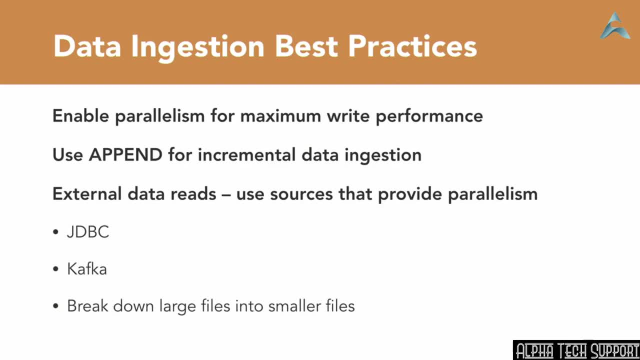 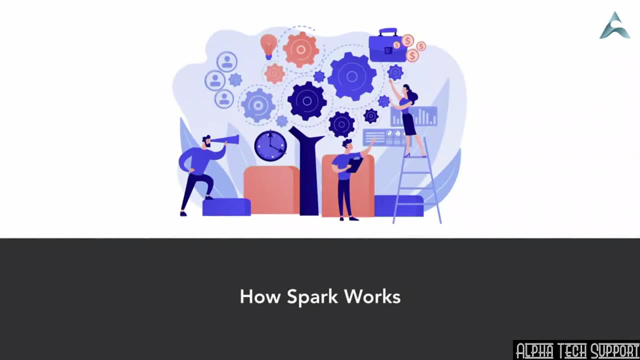 Request the data originators to create such parallelizable data sources. In the next chapter, I will show you how to read data that is stored in an optimal fashion in HDFS. In order to optimize an Apache Spark pipeline, it is important to understand how Spark works. 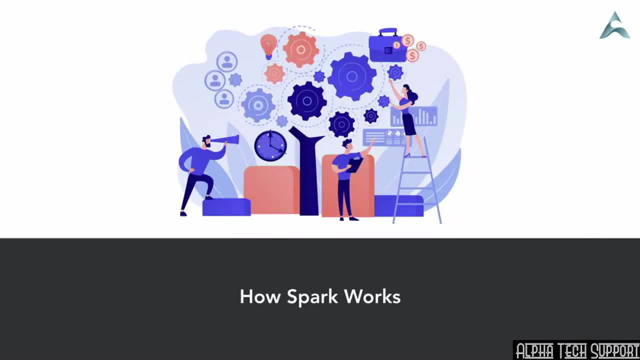 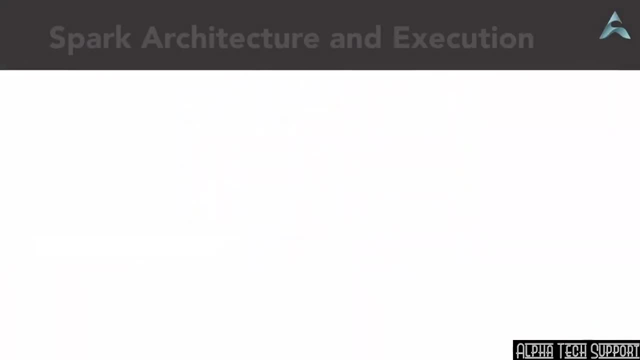 internally. When design decisions are made, they need to be analyzed on how they impact scalability and performance. In this video, I will review how Spark executes a pipeline and optimizes it. I recommend further reading on this topic to master the internals. In this video, I will review how Spark executes a pipeline and optimizes it. I recommend further 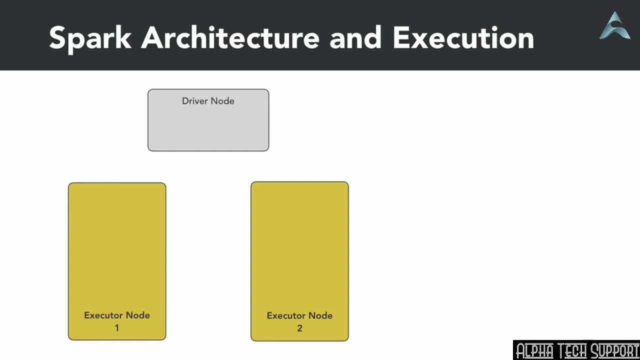 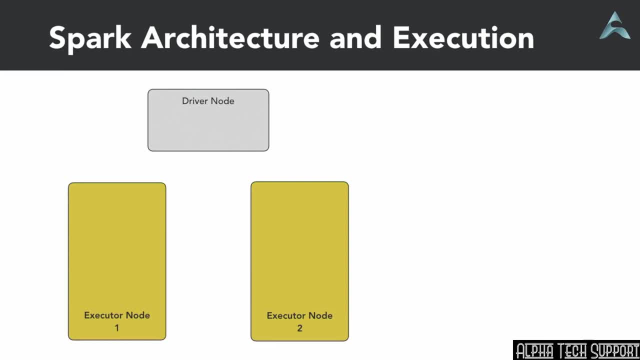 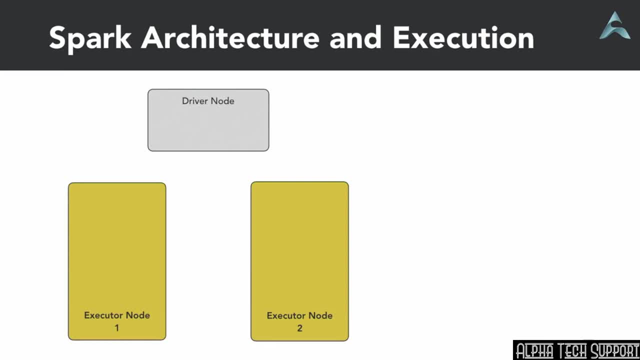 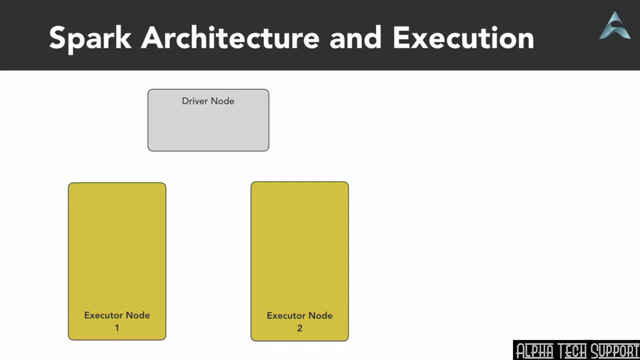 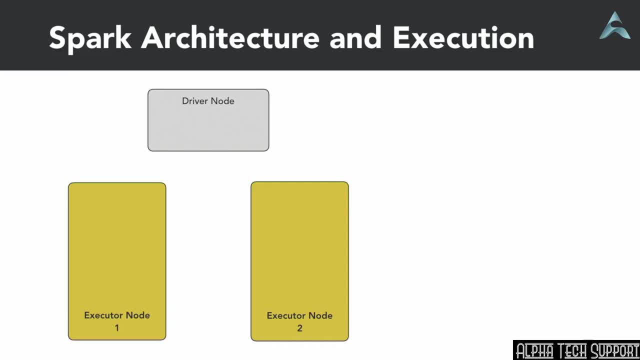 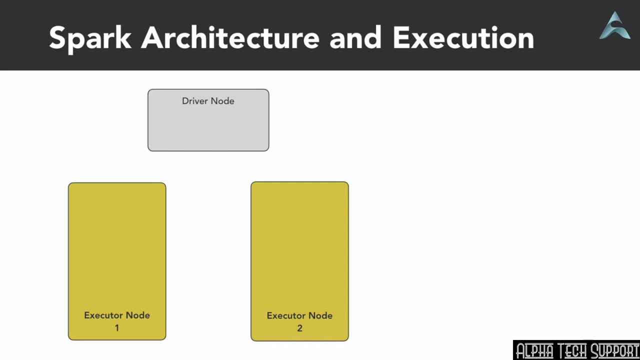 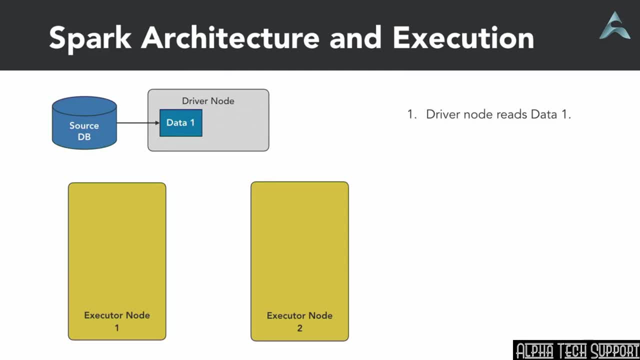 reading on this topic. to master the internals, First, the source data is thread from an external data source into a structure: data 1.. Data 1 is then converted to a data frame or its internal representation. IT is partitioned and individual partitions are assigned and moved to the executor nodes. 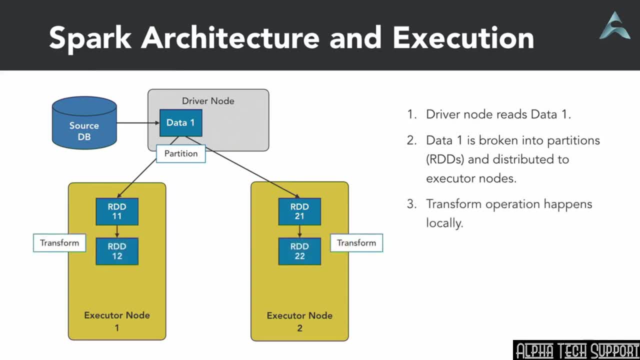 available. It is partitioned and individual partitions are assigned and moved to the executor nodes available. 他說, When a transform operation like Map or Filter is executed, these operations are passed through the RAM machine to the SCR memory and FalseROMs mode. 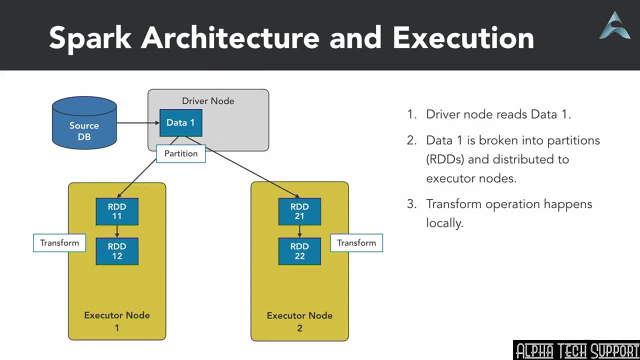 push down to the executors. The executors execute the code locally on their partitions and create new partitions. with the result: There is no movement of data between the executors. Hence transforms can be executed in parallel. Next, when an action like reduce or group by. 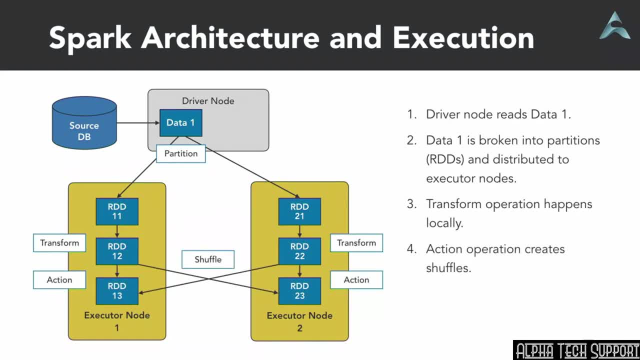 is performed, the partitions need to be shuffled and aggregated. This results in movement of data between executors and can create IO and memory bottlenecks. Finally, the data is collected back to the driver node. The partitions are merged and sent back to the driver. From here they can be. 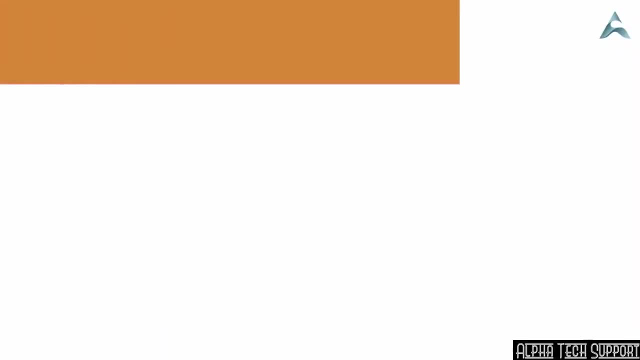 stored into external destination databases. Spark has an optimizer that analyzes the steps needed to process data and optimizes for performance and resources. Spark only executes code when an action like reduce or group by is performed Next, when an action like reduce or group by 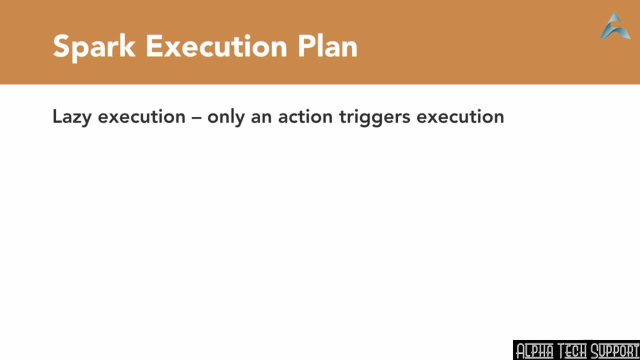 is performed. At this point, the optimizer kicks in and analyzes all the previous steps required to achieve this action. It then comes up with a physical execution plan. The optimizer looks for reducing IO shuffling and memory usage. If the data sources can support parallel IO, then Spark. 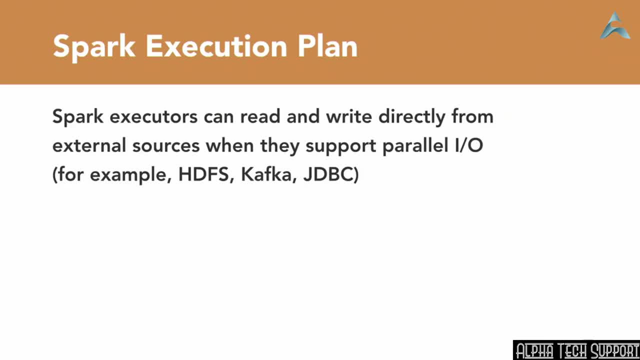 accesses them directly from the executor and parallelizes these operations. This provides improved performance and reduces the number of steps required to achieve this. action Spark also competitors, pizza systems, as well as Windows 365, Linux, CAN, Minecraft, Face Ahhh, Duoedar and Android dont. In the later anecdotes video, I will show you how to influence the 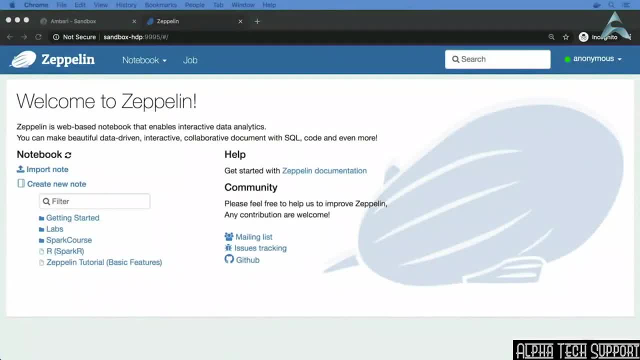 physical plans for better performance. In this chapter we will read the parquet files we created earlier into Spark. We will examine the execution plans to understand how Spark works. to read these files We will use the exercise files. code 04-XX- data extraction. 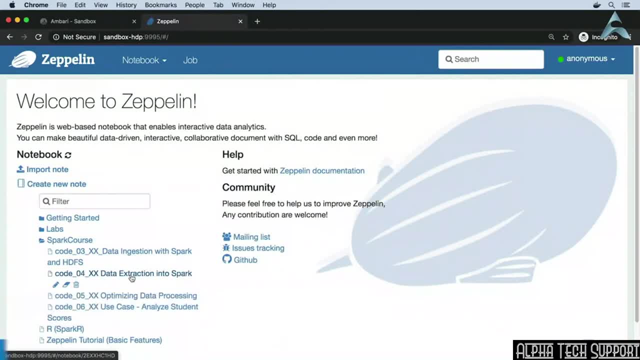 into Spark for this practice, Assume that we run DPU of ddPD in the cellszione file. This is the file for the Spark work, not as rice folder or shader and for storage Using these Bose for this chapter. Let's open this. We can read the non-partitioned raw parquet file into Spark. 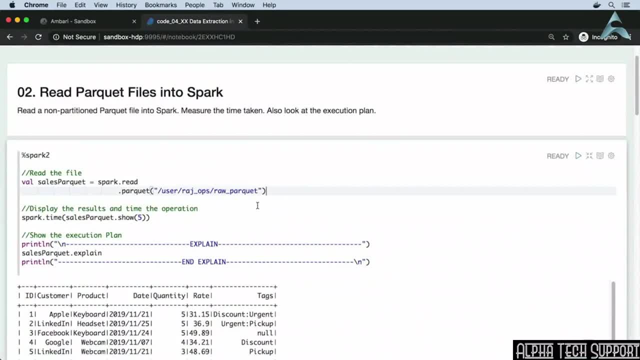 using the readparquet function, We print the first five records in the data frame. We also use the sparktime function to measure the elapsed time for the total operation. Sparktime can be used to compare the performance of different approaches while designing data pipelines. Finally, we execute the explain function to print out the physical plan. 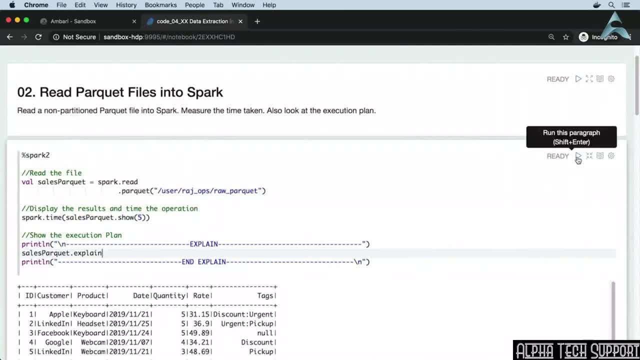 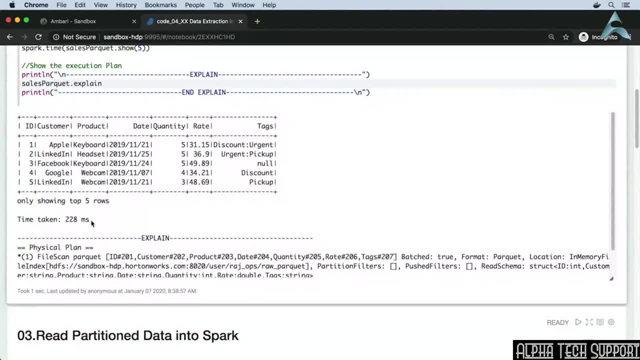 Let's run this code and examine the results. The operation took 228 milliseconds. For a small data set like the one we have here, most of the time is overhead and may not make sense for comparison, but for operations that run for many minutes or a few hours, this can provide a true measure. 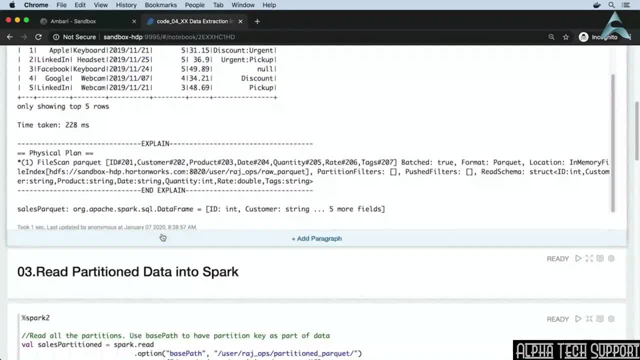 Let's examine the physical plan to understand what it shows. It does a filescan for a parquet file. It shows the columns that are read from the file, It shows the location of the file and then it shows the schema that is used to read the file. 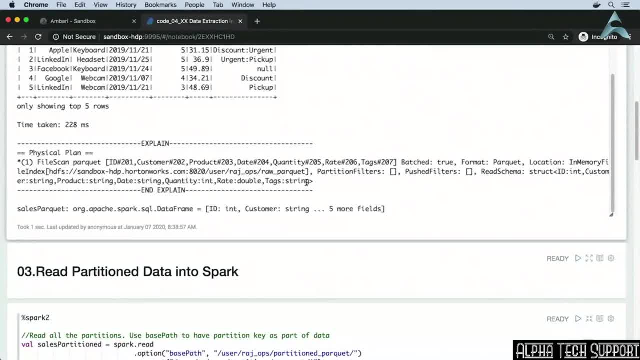 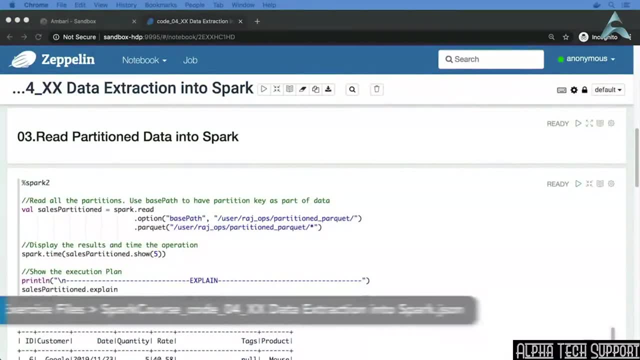 We will examine the rest of the contents in the future examples as we exercise them. In this video we will review the first two achievements: SWIA tests. In the second content we will consider the read a partitioned data set into Spark and understand how it works. We will read the parquet. 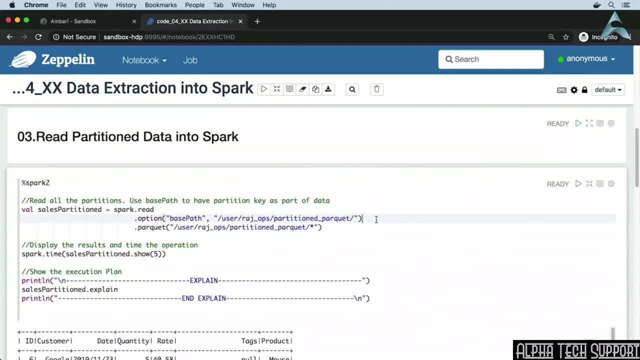 files under the directory partitioned parquet. The product name, which is the partition value, will not be stored inside the files as it is already available in the directory name. The base path needs to be provided for the data to read the product name also as a column. We. 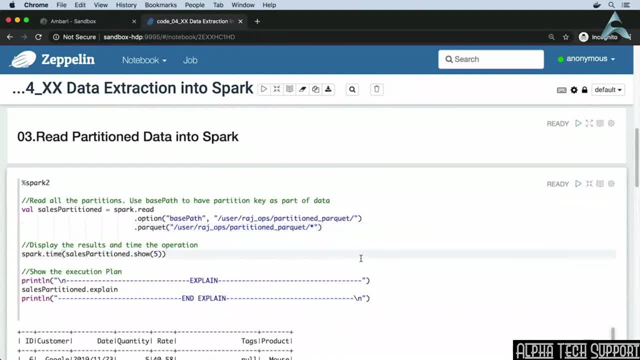 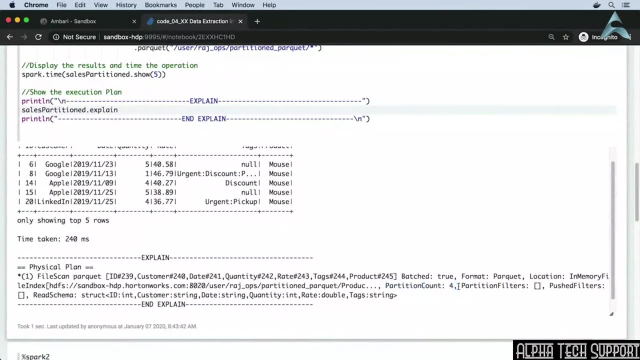 again time the operation and display the first five roles. We will also print the execution plan. Let's run this code and review the results. The most important addition to the physical plan is the partition count. This shows the number of partitions read into memory. More partition means more IO and memory. 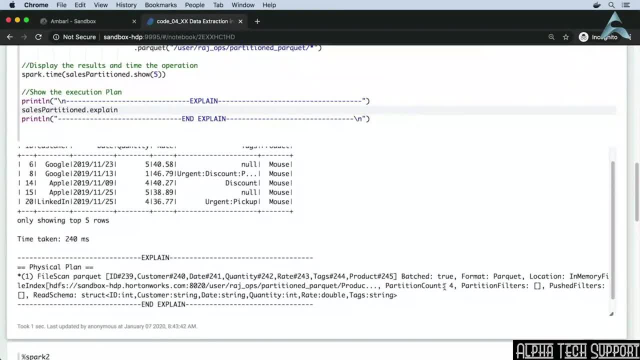 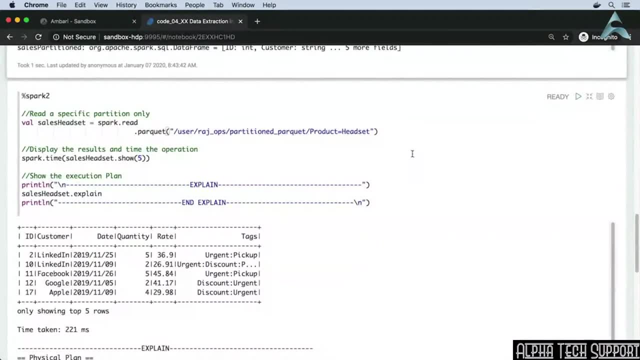 requirements. Reducing this count will lead to better performance. We will see techniques for this later in the course. Next, we only read one partition from the stored data. If we need to analyze only a subset of data, it is recommended to only read that subset and minimize IO and 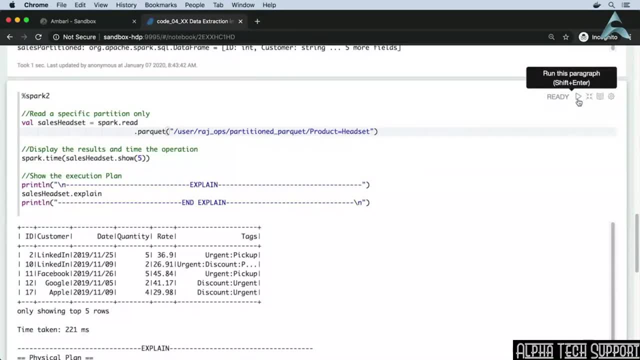 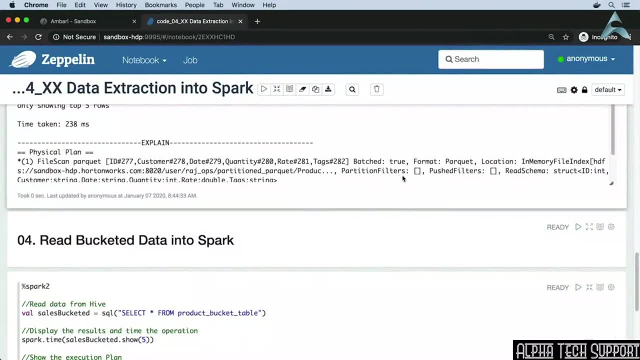 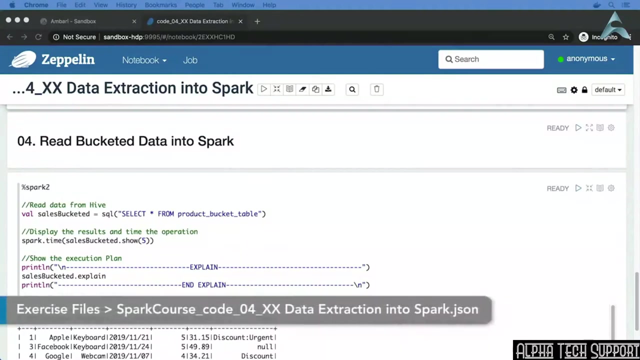 memory. Let's run this code now In the physical plan. you will notice that the partition count is not printed, as only one subdirectory has been read. In this video, I will show you how to read bucketed data from Hive. In this video, I will show you how Spark reads bucketed data stored in Hive. 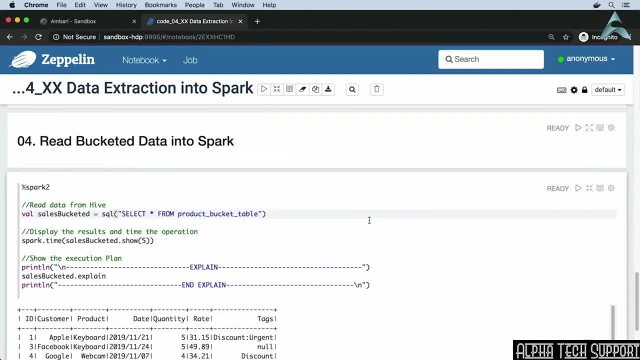 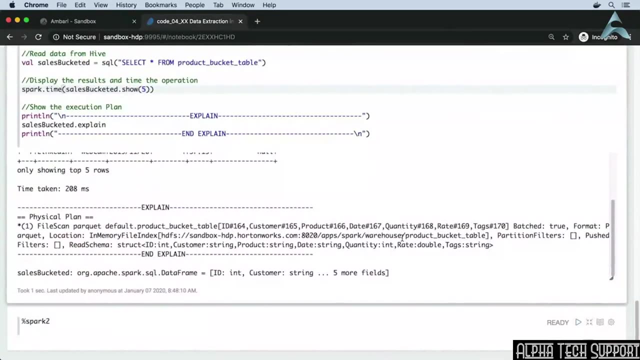 We can read data in Hive using a SQL command. We do a simple select statement to read the entire table and print its contents. We also print its execution plan. Let's run this code and examine the results When we look at the execution plan. 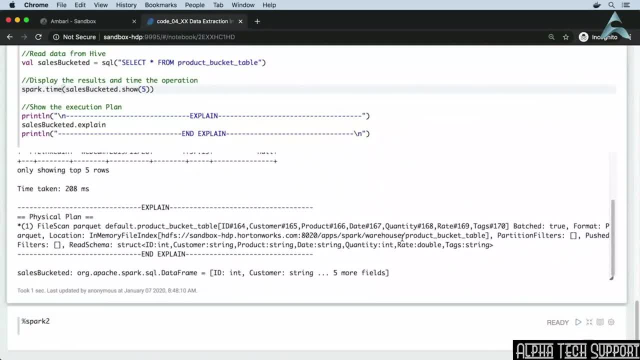 can see that it is no different than reading a file from HDFS. Data frames, data sets, SQL and RDDs provide different interfaces to the same underlying operations, So the execution plans will be similar, irrespective of which API we use. The plan still shows what HDFS file is read. 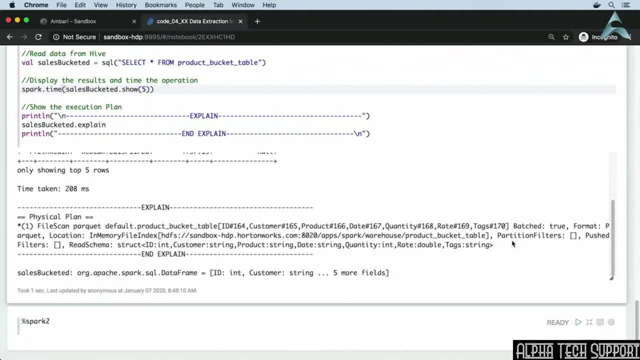 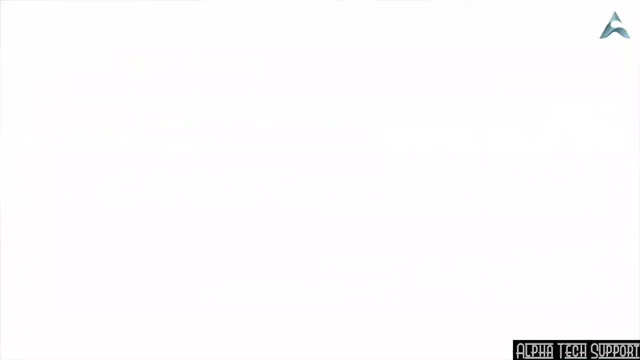 and will also provide partition information if it is used. We will now review some of the best practices for reading data into Spark in the next video. What are some of the key best practices for data extraction from HDFS into Spark for analytics? The first is to read only the required data into memory. This means read subdirectories. 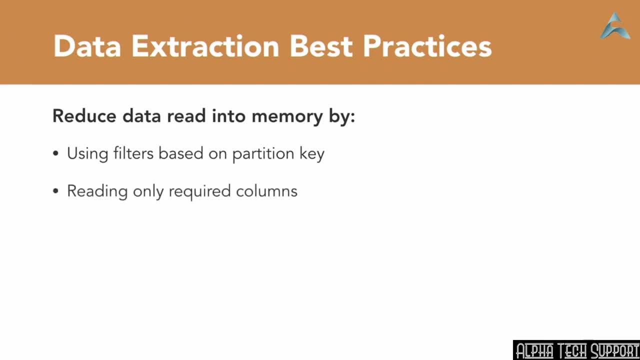 subset of partitions and subset of columns. Less data means less resource requirements and less time to execute. Use data sources and file formats that support parallelism. Avro and Parquet are some of the recommended ones. The number of partitions in the data files are important. Each partition can be independently. 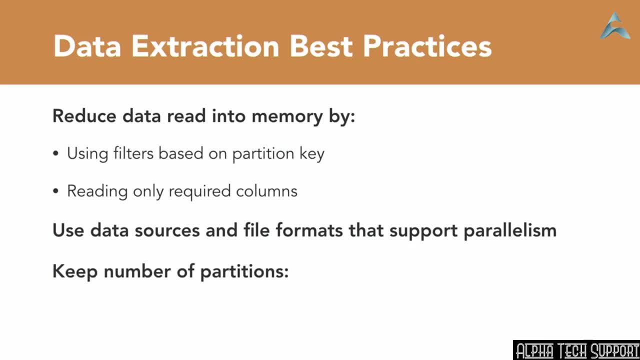 read by a separate executor code in parallel. The number of parallel operations in a Spark cluster is the number of executor nodes multiplied by the number of CPU codes in each executor. If the number of partitions are greater than this value, it will trigger maximum parallelism. 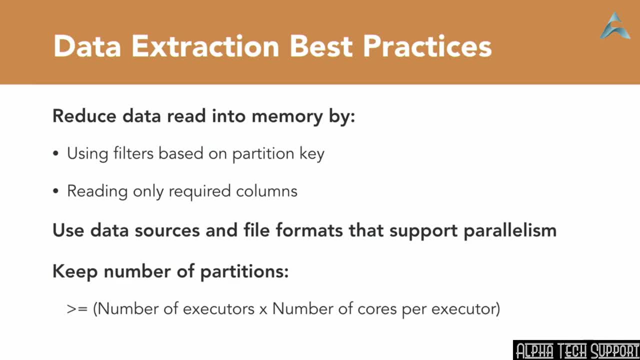 Please keep in mind that other jobs running at the same time will also require parallelism. Please keep in mind that other jobs running at the same time will also require parallelism. Please keep in mind that other jobs running at the same time will also require parallelism. 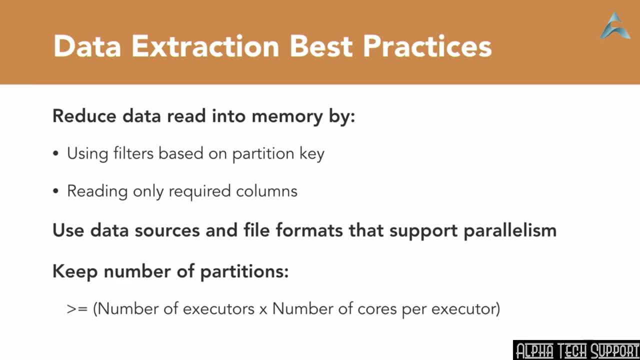 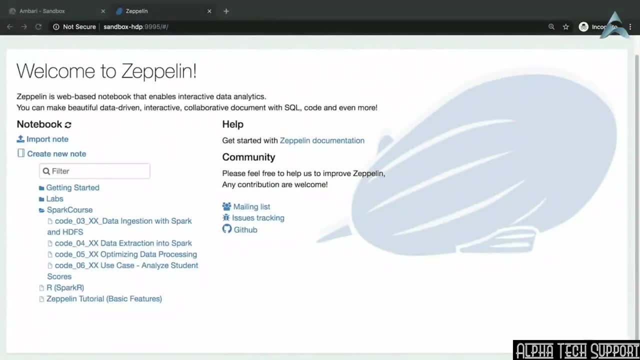 In the next chapter I will focus on optimizing processing data read from HDFS. In this chapter, we will review some of the techniques that can be used during data processing to optimize Spark and HDFS performance. The code for this chapter is available in the notebook. 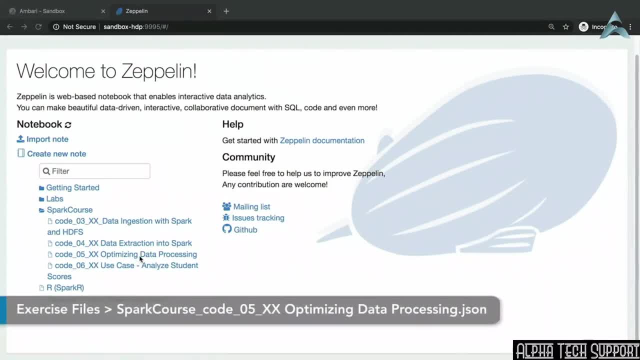 code: 05-xx- Optimizing Data Processing. 05-xx Optimizing Data Processing e: 1. 1. 1 1 2. 1, 2, 3, 4, 4, 5, 6, 5, 7, 6, 6, 7, 7, 6, 7, 7, 7, 8. 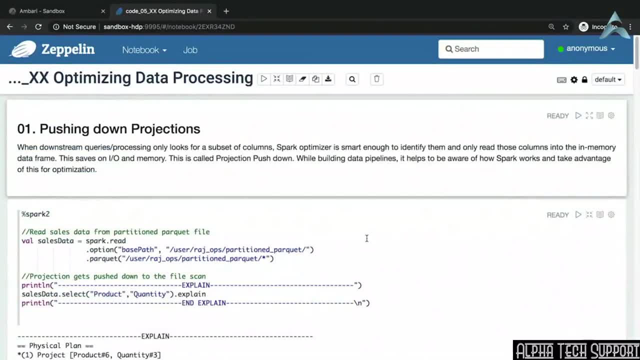 8, 7, 7, 7, 7, 8, 8, 7, 7, 7, 7, 7, 8. We first start with pushing down projections. Projection here means the set or subset of columns that are selected from a dataset. Typically we read an entire file with all the columns into memory and then use only. 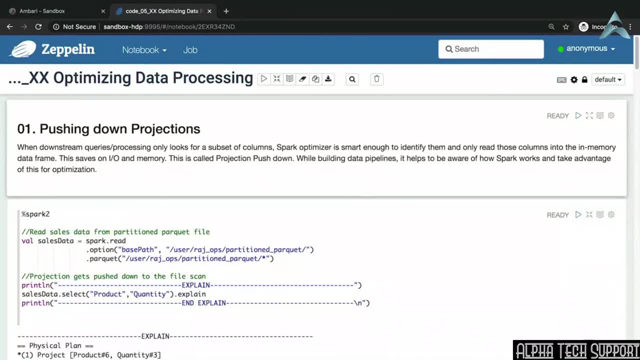 a subset of columns later for computations During lazy evaluation, Spark is smart enough to identify the subset of columns that would actually be used and only fetch them into memory. This is called projection pushdown. In this example, we read the entire Parquet file into the SalesData data frame. 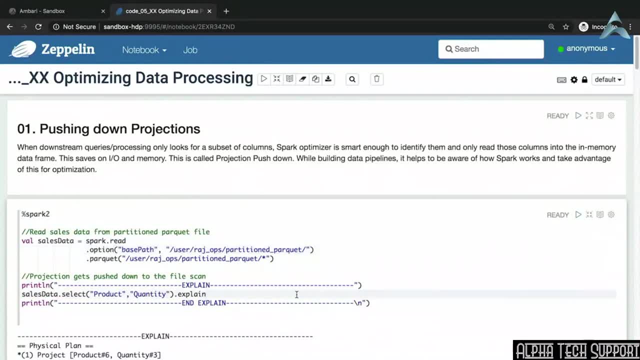 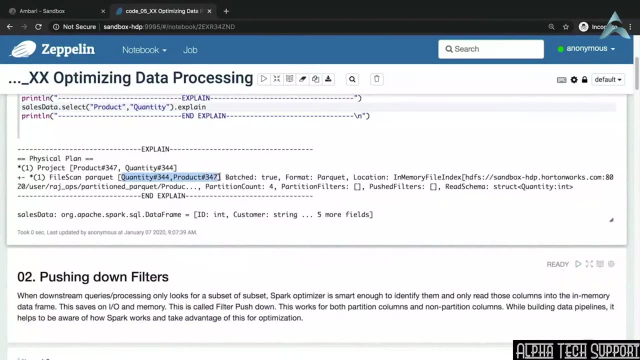 Later we only select the product and quantity columns. Spark identifies this and only fetches these columns into memory. Let's run this code and review the execution plan. In the execution plan, the file scan reads only two columns- quantity and product, and this provides optimization. 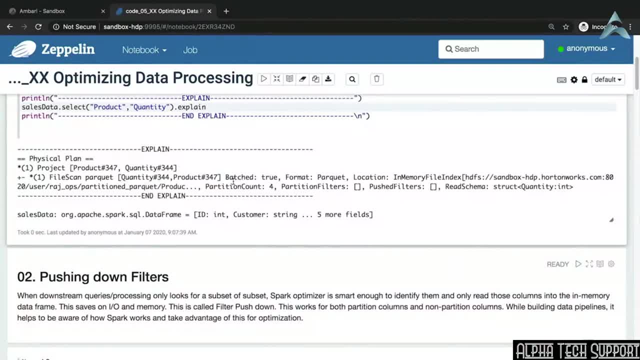 A pipeline developer needs to help Spark to do these optimizations by not using columns unnecessarily. For example, using a show function with all the columns, even for troubleshooting, would fetch all the columns and prevent projection pushdowns. In the next video, let's look at pushing down filters. 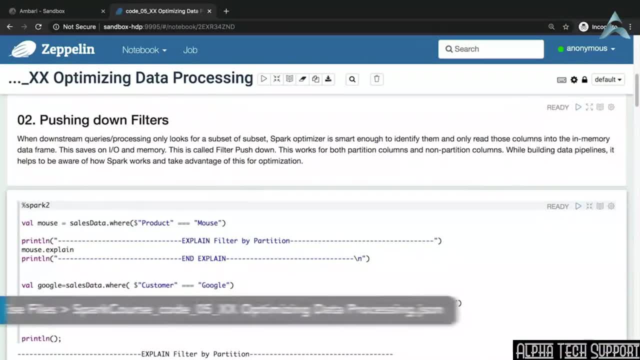 Similar to projection pushdowns, Spark is capable of identifying a subset of rows that are actually required for processing and fetch them into memory. If the subset of rows correspond to specific partitions, Spark will only read those partitions. In this example, we try two filters. 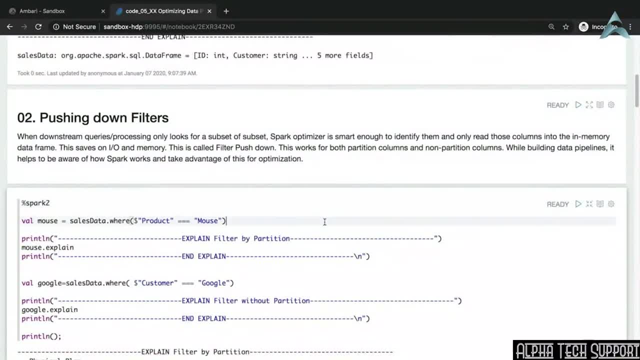 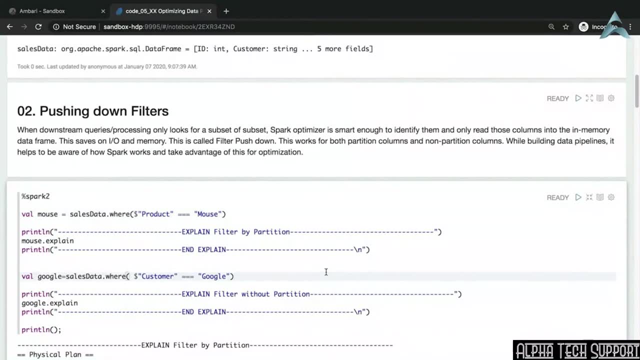 One is a filter on product. Product is a partitioned column. The other is a filter on a non-partitioned column called customer. The other is a filter on a non-partitioned column called customer. Spark will push down both these filters to the file scan so it will not read unnecessary. 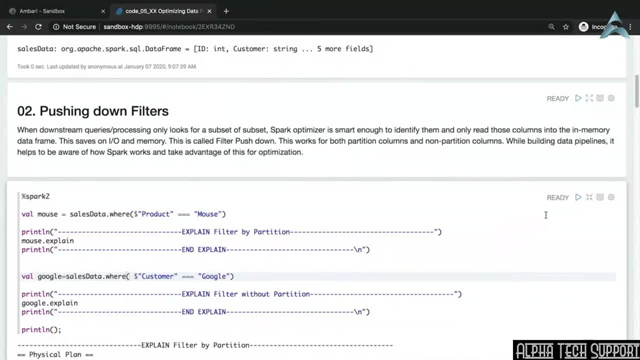 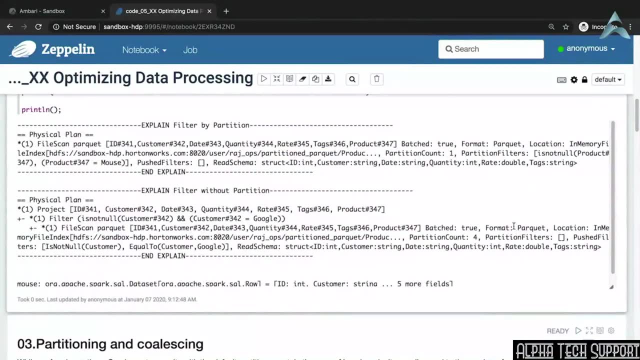 rows into memory. Let's execute the code and review the results. In the case of a filter on a partitioned column, we see partitioned filters being used. The partition count is also 1.. This means that Spark has identified that the filter is on a partition and only one. 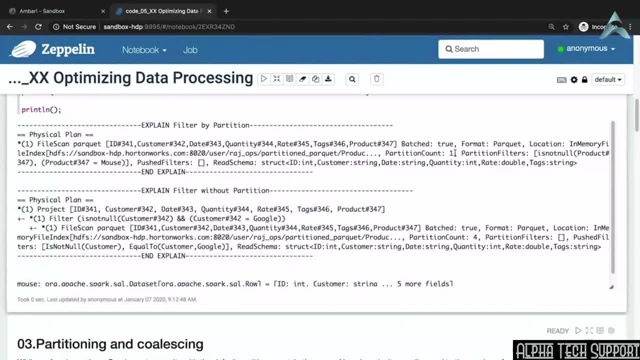 filter is on a partition. This means that Spark has identified that the filter is on a partition and only one filter is on a partition, So it will only attempt to read files for that partition. In the case of a filter without a partitioned column, we see pushed filters on the file. 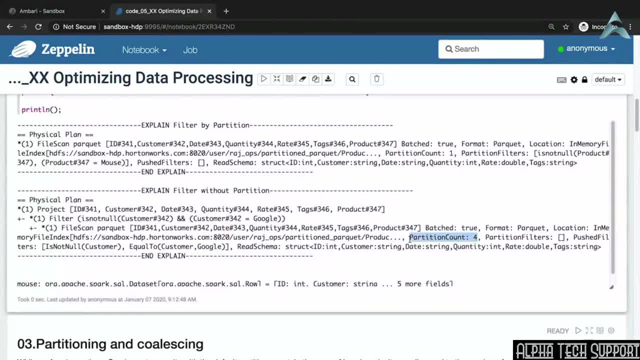 scan, but the partition count used is still 4.. Partition-based filter pushdown is most efficient, since Spark will only attempt to read files within that partition. In a non-partitioned case, it has to read all the files or partitions, but only load those. 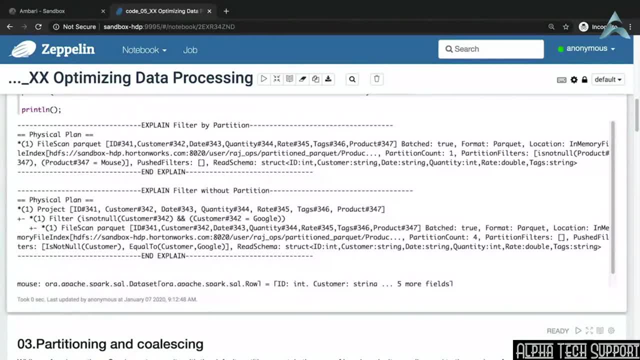 brackets that match the filter condition. The result is a partitioned column. Understanding this mechanism helps design partitions to maximize push-downs. This saves on IO and memory. The earlier the filtering happens, less data needs to be processed in the later stages in the pipeline. 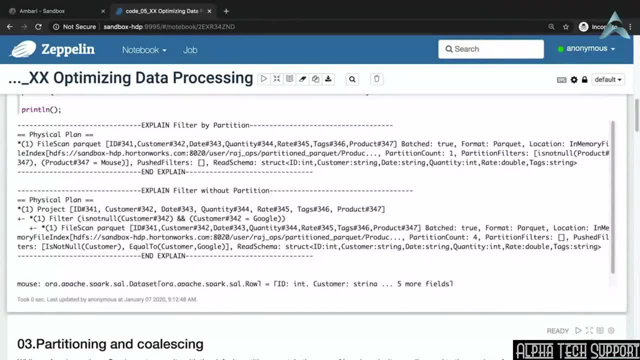 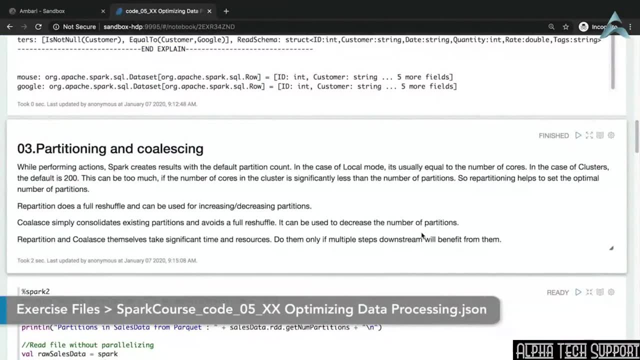 In the next video I will discuss partitioning and collasing. One of the key aspects to understand about Spark internals is partitioning. This is different from HDFS partitioning. When Spark reads a partition file, it creates internal partitions equal to the default parallelism set up for Spark. 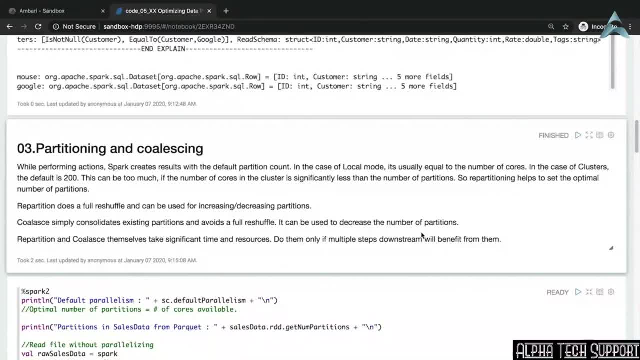 Transforms maintain the same number of partitions, but actions will create a different number, usually equal to the default parallelism set up for this Spark instance. Typically in a local node parallelism is 2 and in a cluster mode it's 200.. 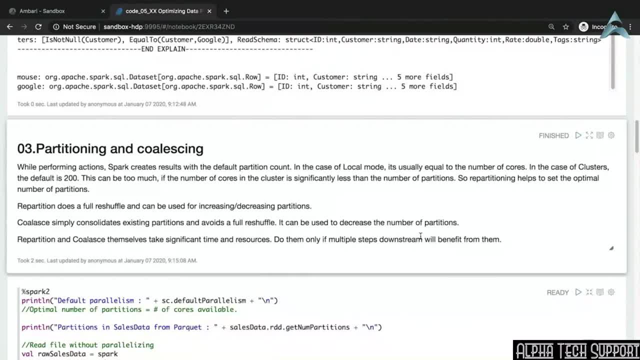 Having too many or too little partitions will increase the number of partitions. This is called impact performance, As discussed in the earlier video. the ideal number of partitions should be equal to the total number of codes available for Spark. We can change the number of partitions by repartitioning and collasing. 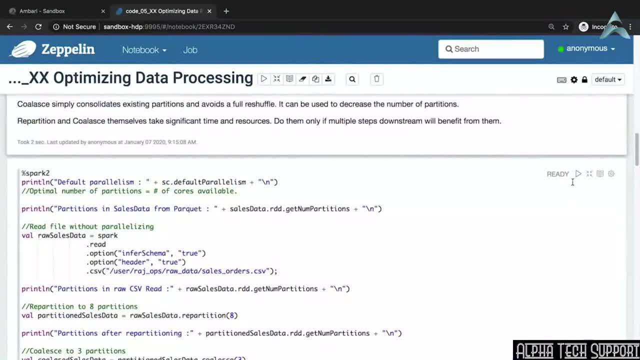 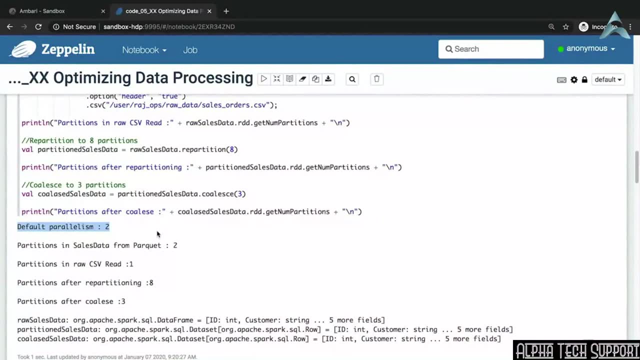 Let's run the exercise code first and then review the results. We first print the default parallelism set up for this cluster. It's 2.. This number can be changed in Spark configuration. Then we look at the number of partitions on a partitioned data source, which is sales data. 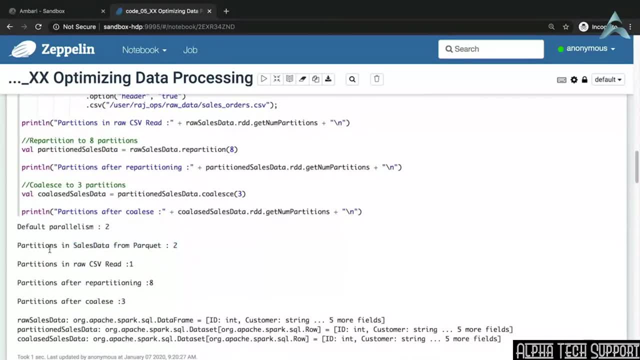 The number of partitions is again 2.. Next, we read a non-partitioned data source, which is the raw orders file, and look at the partition count. This number is only 1.. This is the problem with having data sources that do not support parallelism. 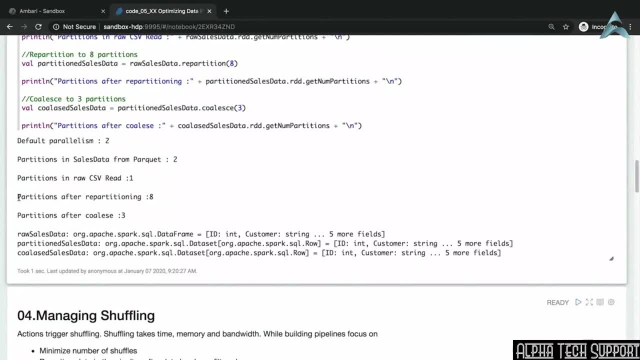 An RTD can be repartitioned. This number can be repartitioned to a new number of partitions. using the repartition function, We can specify the number of partitions. We repartition raw sales data into 8 partitions and confirm that count. 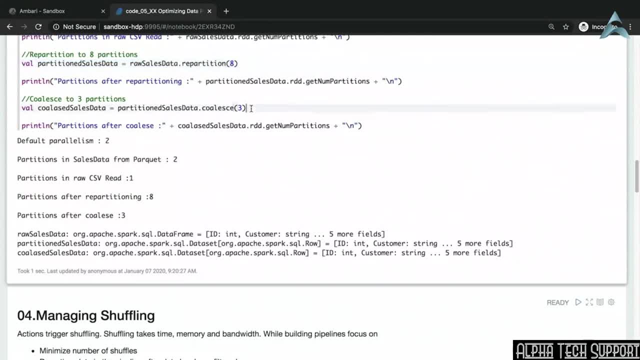 Next, we can also coalesce a data frame to reduce the number of partitions. We coalesce the partition sales data from 8 partitions to 3 partitions And we also print and confirm that size Repartitioning does partitioning from scratch. 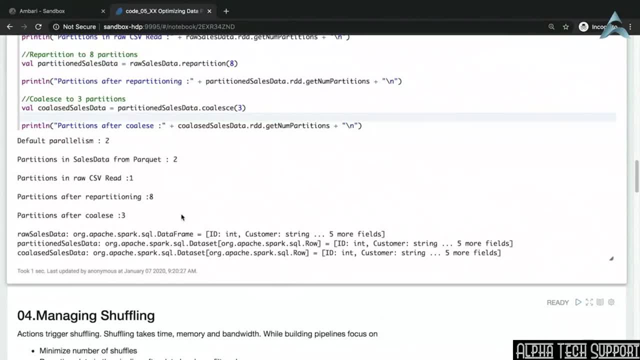 Coalescing simply combines existing partitions to create a larger partition. Note that both these activities themselves take significant amount of time. Typically, actions upset the ideal partition count and hence repartition need to be done after that, But it's recommended to do that only if there are multiple transforms that follow the action. 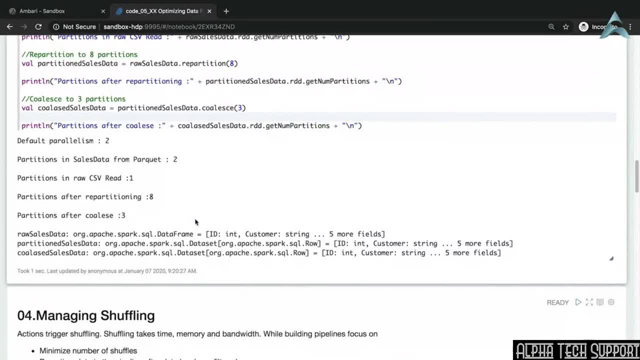 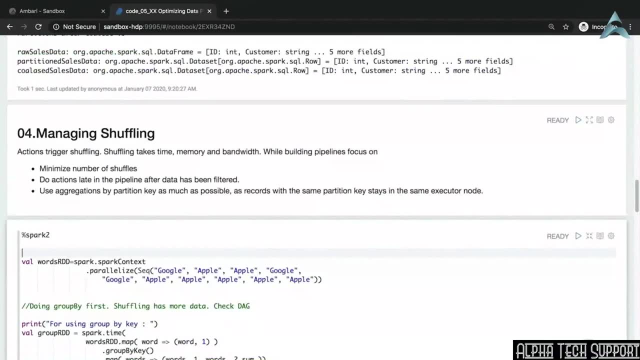 and can take advantage of these resized partitions. In the next video, I will show you how to optimize shuffling. As seen in the earlier videos, Spark actions like reduce and groupby cause shuffling of data between executor nodes. This creates IO and delays in overall processing. 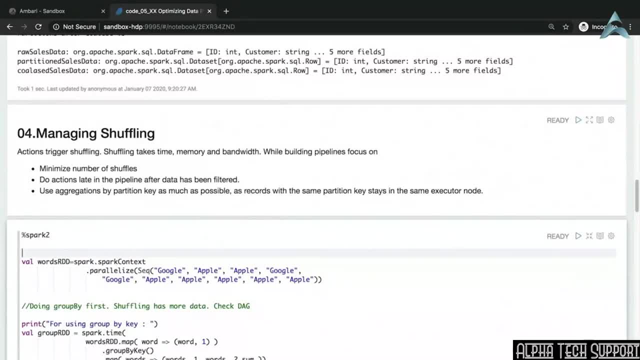 Spark optimizer does a lot of work in the background to minimize shuffling. However, as a designer, it's still important to understand the shuffling impact of the design and focus on minimizing it. We can either eliminate shuffling steps or minimize the amount of data being shuffled. 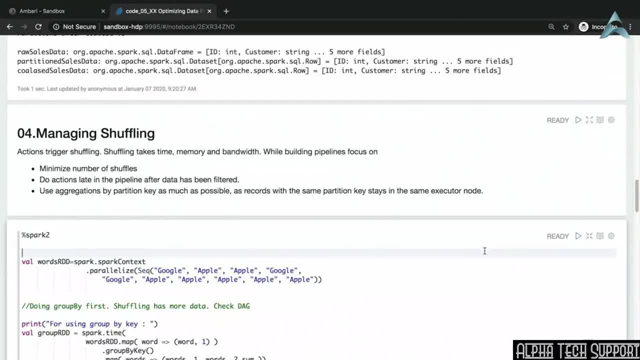 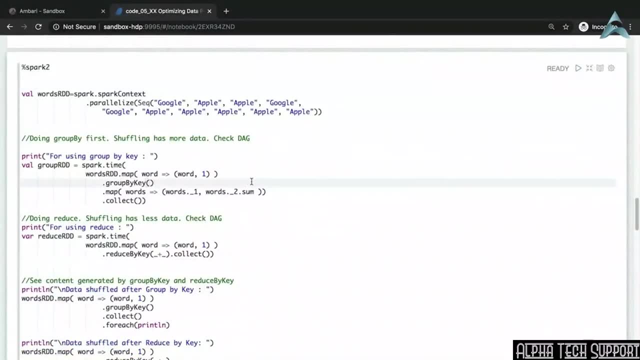 In this exercise we will implement two different word count logics and compare the shuffling between them. The first method uses a groupby key and then a map to compute the word count. The second method uses a reduceby key directly. Let's run this code and review the results. 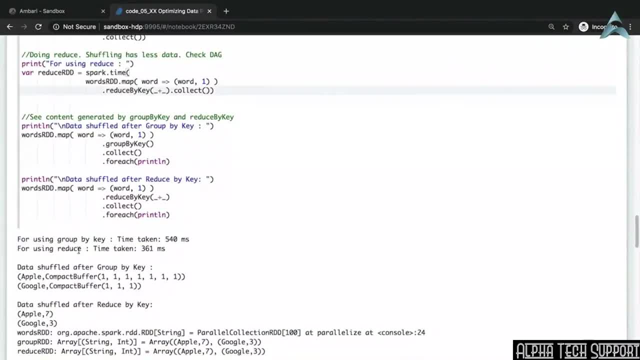 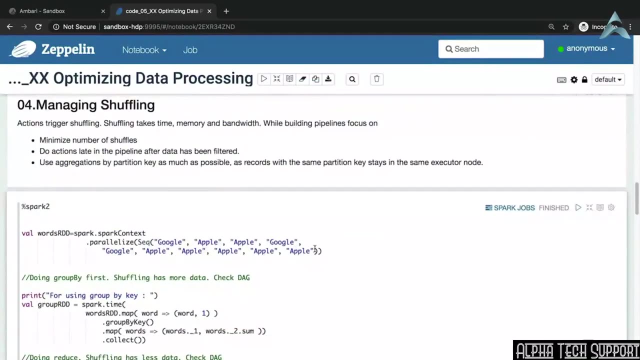 The groupby key took 540 milliseconds. the reduce took 361 milliseconds. Comparison of time taken may not make sense for small datasets, but doing the same on large datasets will provide the real difference. Let's check the Spark UI for the execution plan for these alternatives. 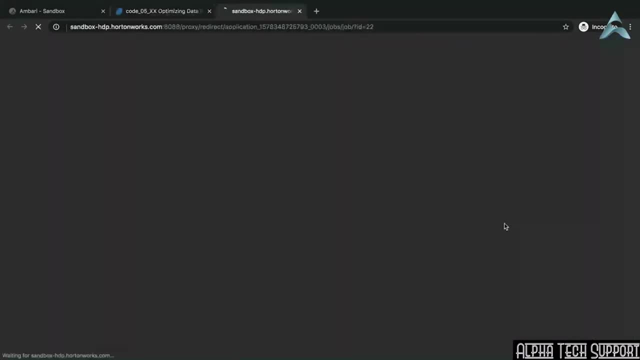 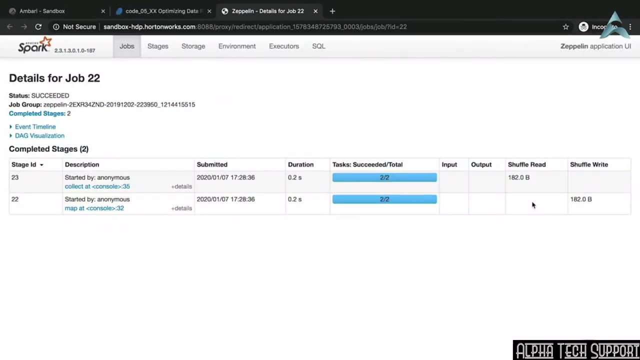 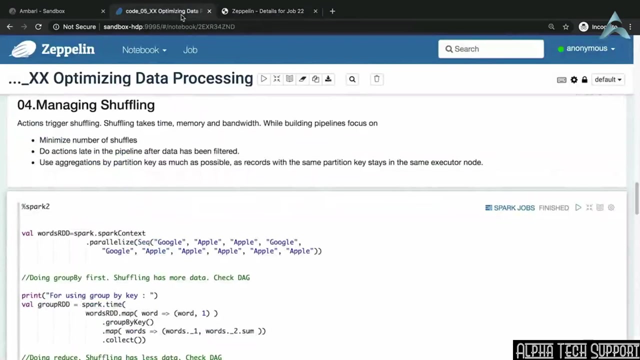 First let's click on job 0 for the execution plan for groupby. Look at the shuffle read and shuffle write numbers here. They indicate the amount of data being shuffled. This is 182 bytes for groupby. Next let's look at job 1.. 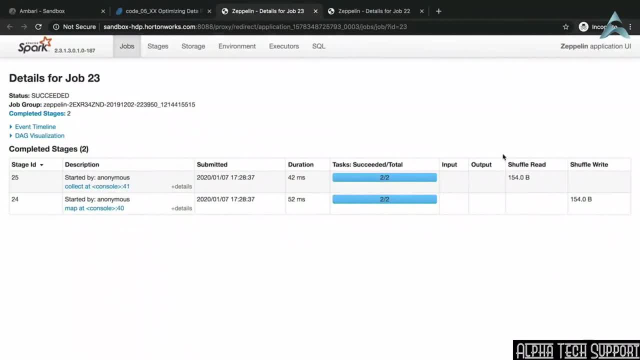 This is the execution plan for the reduceby key. We see that the shuffle read and write numbers are 154.. The data shuffled here for reduceby key is less than that of the groupby key. Let's also look at the actual data being shuffled. 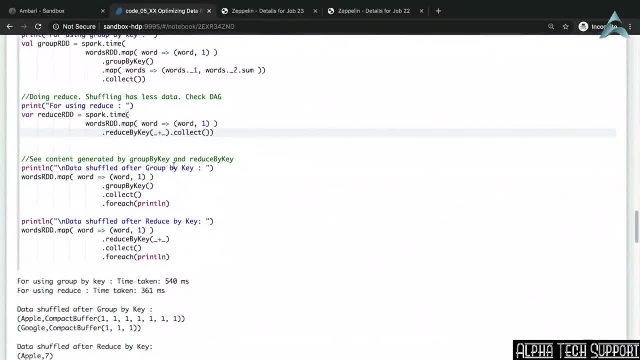 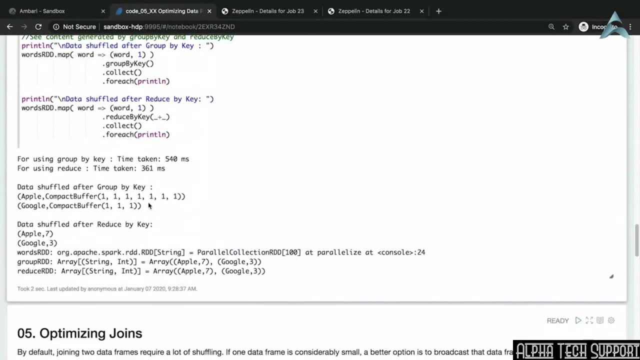 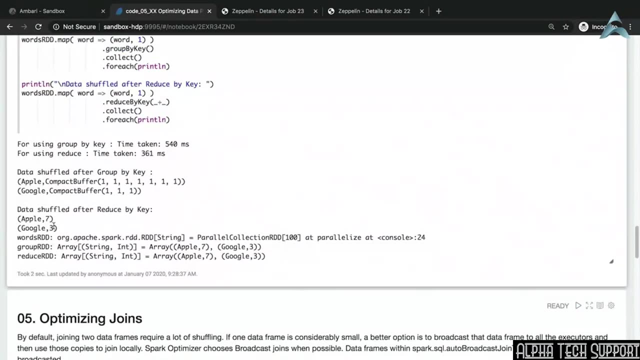 To look at the actual data being shuffled. we print the outcomes of these activities. We see that, in the case of a groupby key, individual values are being shuffled, whereas in the case of a reduceby key, only the sum is being shuffled, leading to less data. 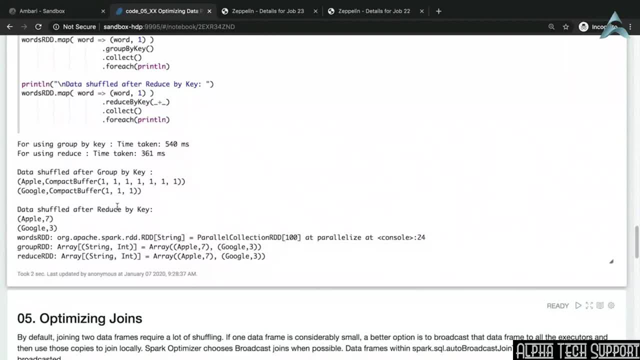 This is a very small dataset. In the case of large datasets, the difference can be significant. It is important to look at execution plans and the data sizes being shuffled and optimize them for building faster processing pipelines for analytics. In the next video, I will show you how to optimize joins. 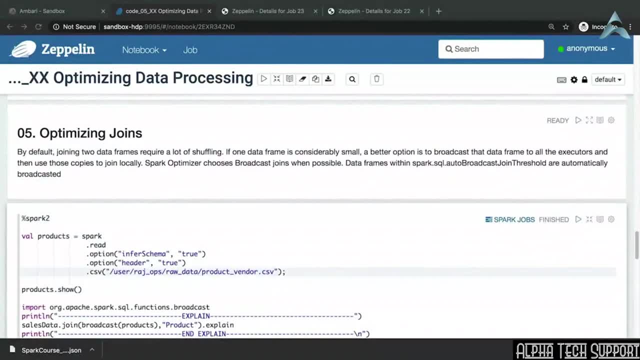 Joins in Spark help combining two datasets to provide better insights. As important as they are in analytics, they also cause significant delays. Joins between two dataframes require that the partitions of these dataframes to be shuffled so rows that match the join condition are in the same executor nodes. 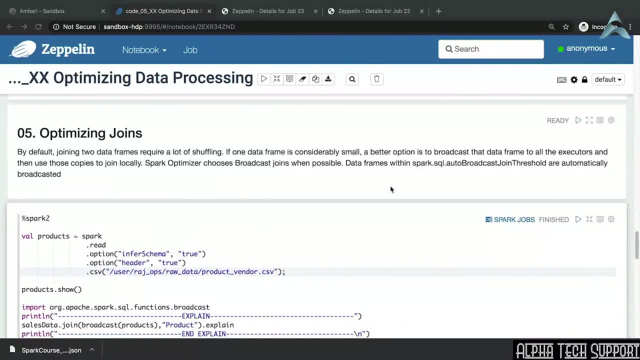 Spark Optimizer again does a lot of behind-the-scenes work to optimize joins. One of them is called a broadcast join. If the size of one of the joined dataframes is less than the sparksqlautobroadcast join threshold, then Spark broadcasts the entire dataframe to all executor nodes where the other dataframe resides. 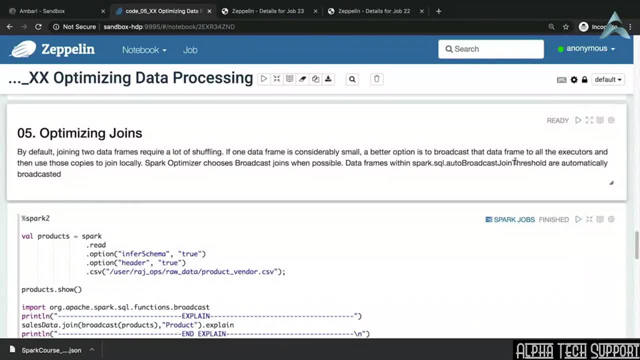 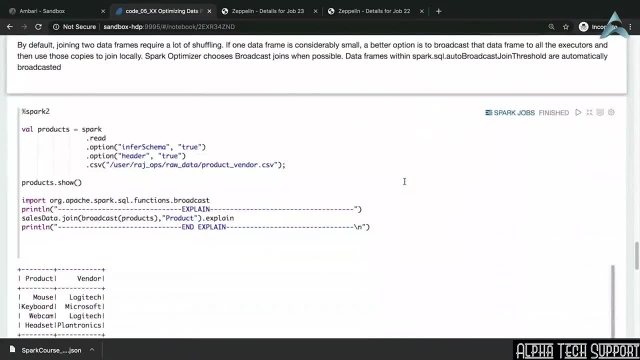 Then the join itself becomes a local activity within the executor, since the entire copy of the smaller dataframe is available in that node. In this example, we read the product-vendorcsv into the product's dataframe. This dataframe itself is very small. We then join it with sales data to produce a combined dataframe. 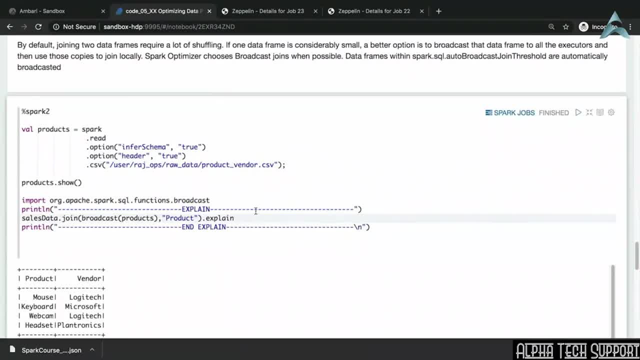 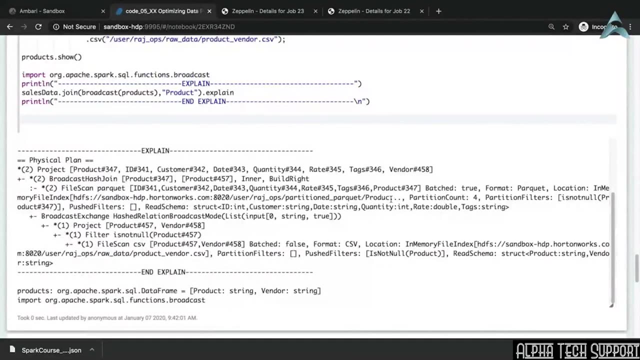 In Spark we provide a join int to recommend the use of broadcast joins using the broadcast function. Let's execute the code and look at the execution plan that Spark has generated. We see that there are two parallel file scan operations to read both the files. 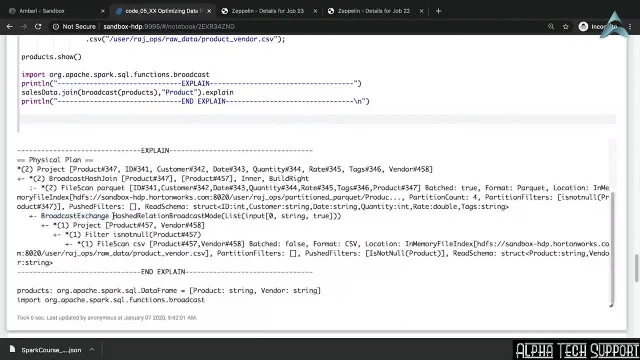 Then we see a broadcast exchange operation for the smaller product's dataframe. This means that this dataframe is broadcast to all executor nodes. Then we see the broadcast hash join function for the actual join. It is recommended to use denormalized data sources and avoid joins if possible. 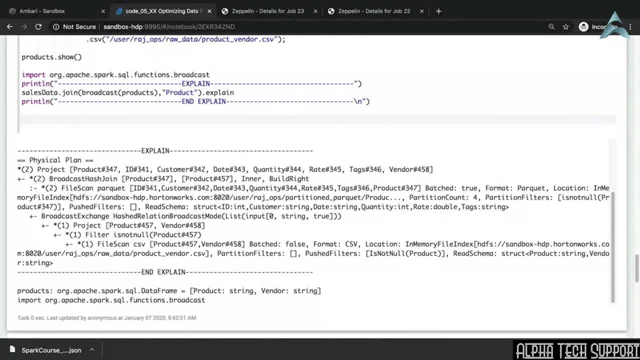 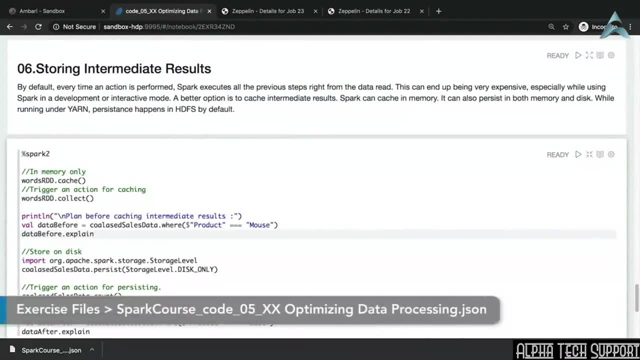 Else review the execution plans to make sure that the joins are optimal. As we have seen in the previous examples for execution plans, every time an action is performed, Spark goes all the way to its data source and reads the data. This happens even if the data was read before and some actions were performed. 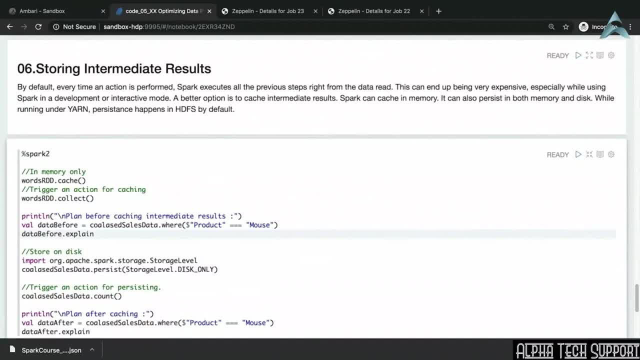 While this works fine while running automated jobs, it is a problem during interactive analytics. Every time a new action command is executed on an interactive shell, Spark goes back to its source. It is better to cache intermediate results so we can resume analytics from these results without starting all over. 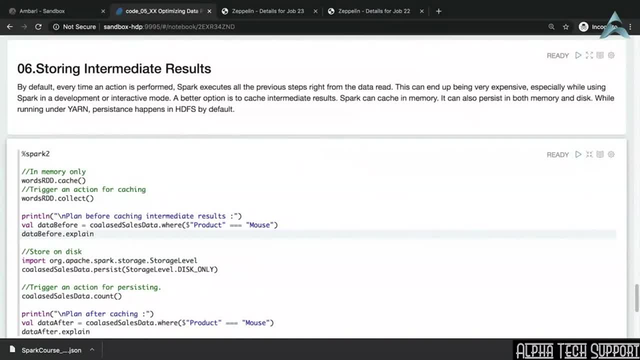 Spark has two modes of caching: in-memory and disk. The cache method is used to cache in-memory only. The process method is used to cache in-memory, disk or both. In this example, we first cache the words RDD into memory using the cache function. 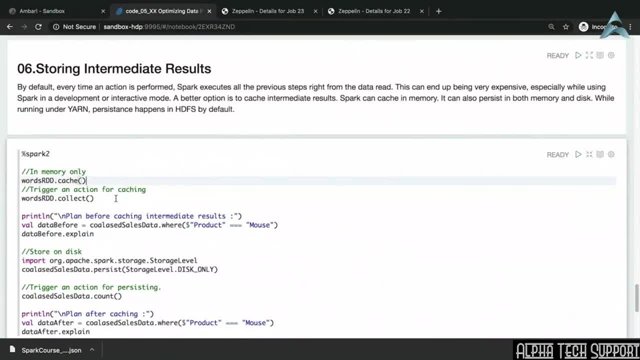 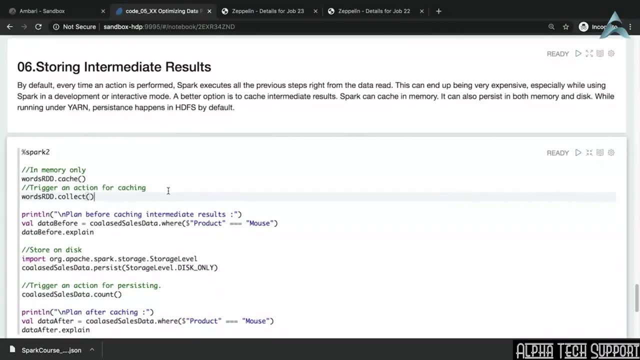 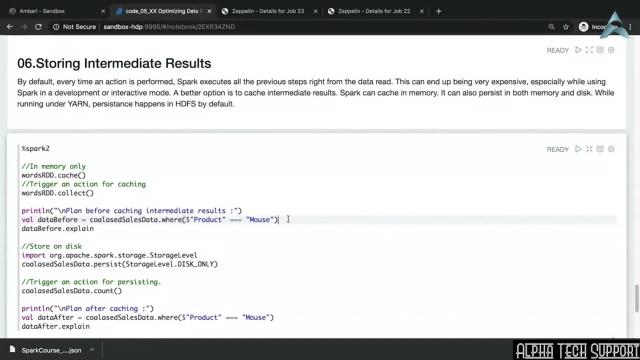 Spark does lazy evaluation so we need to execute an action to trigger the caching. Next we will compare execution plans before and after intermediate caching. First we do a filter for product equals mouse on the Koalas sales data. Then we use the purses function to store the intermediate Koalas sales data data frame to disk. 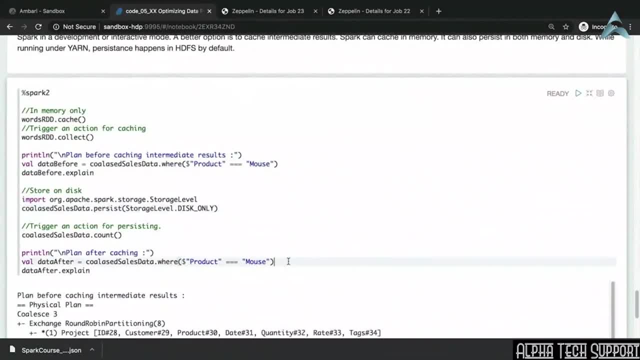 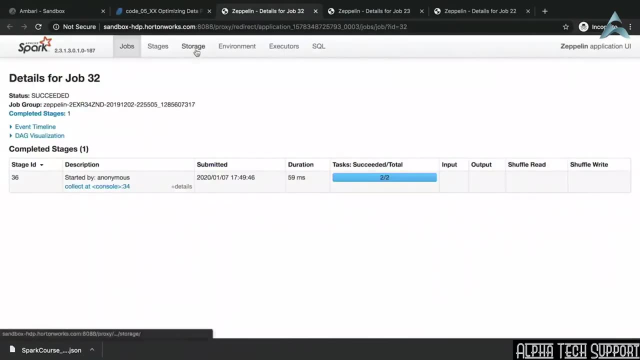 We then run the same filter for product equals, mouse on this data frame and then review the execution plan. Let's run this code and review the results. First let's open the Spark UI, Go to the storage tab. This shows all the cached and persisted data frames. 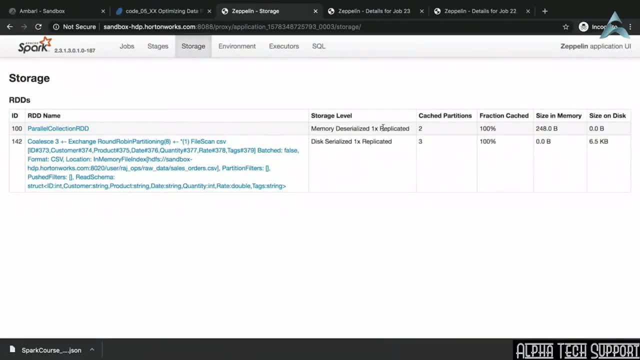 We see the first words RDD showing as stored in memory. We also see the Koalas RDD being stored in disk. We Koalas into three partitions before and we see the same partition count here. Next let's review the execution plans. 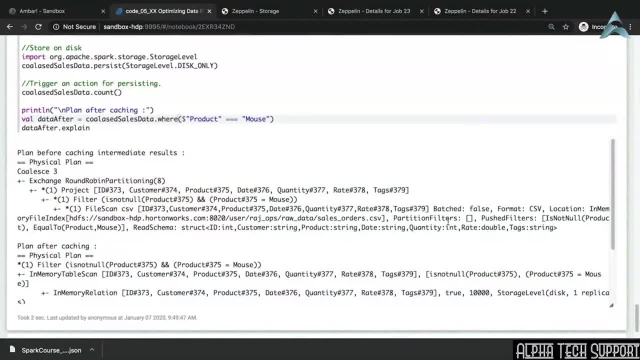 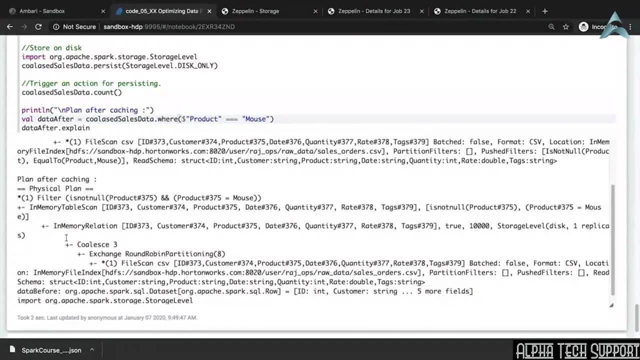 In the plan before caching, we see that there is a filter pushdown. The filter pushdown goes all the way to the file scan. This means that Spark goes all the way back to the file and re-executes all the code. In the second plan, after caching, we see that there is an in-memory scan and the filter is on this in-memory scan. 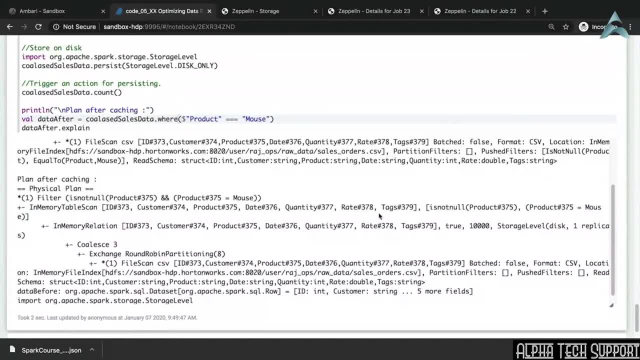 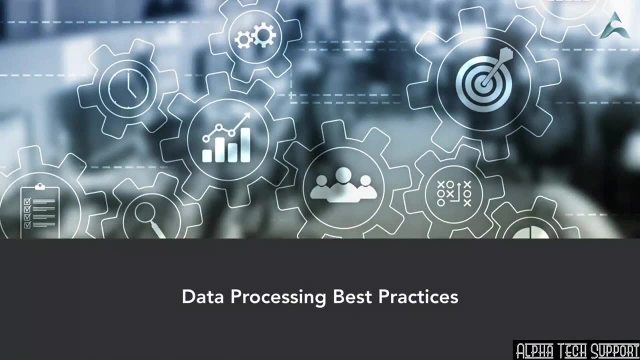 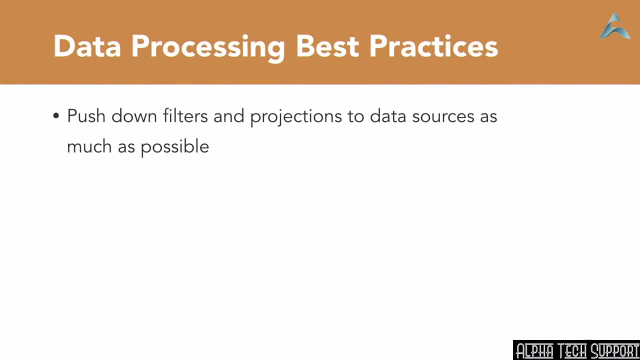 This means that Spark is using the temporary persisted data frame for doing this. filter Caching helps in performance and reuse, especially while doing interactive queries. In this video, I will review the best practices for data processing with Spark and HDFS. Use pushdowns for filters and projections to data sources as much as possible. 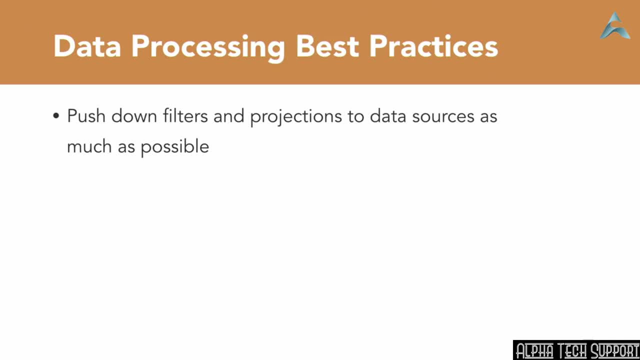 The smaller the data being transferred, the better is the performance. Choose and design partition keys based on the columns most used in filters and aggregations. This speeds up both reading and processing data. Use, repartitioning and coalescing wisely. These activities themselves take significant time, so only use them if there are a series of transforms that can take advantage of them. 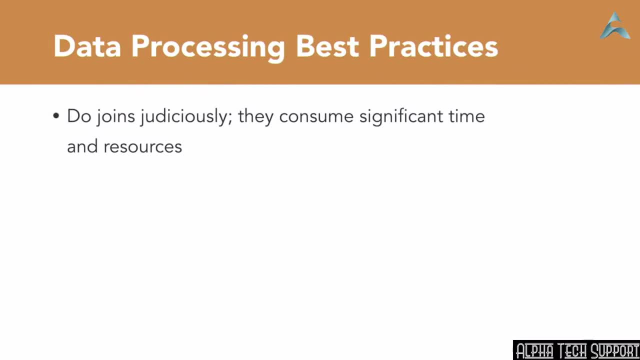 Avoid joins as much as possible. Use denormalized data sources If required. use them judiciously and check execution plans. Clock all operations with sparktime on production. equivalent data to understand slow running operations and take actions. Use caching when appropriate. 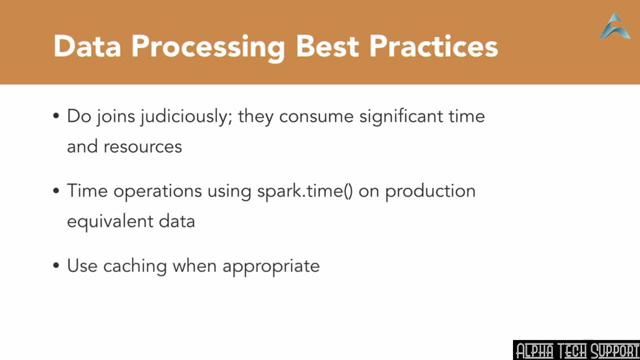 Caching takes memory and disk space, hence choose them for intermediate results that are frequently reused. Use explain plan to understand the physical plan and look for ways in which the plan can be made better. In the next chapter we will do a use case project to exercise the learnings in this course. 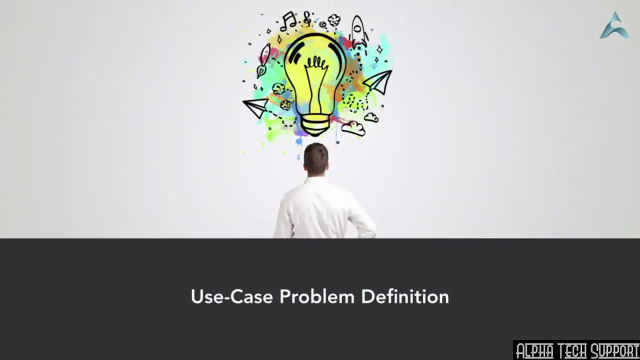 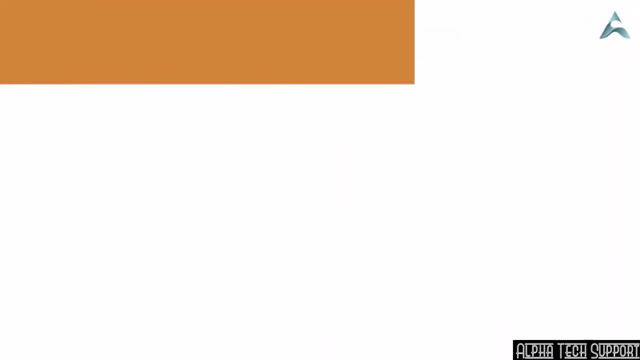 In this chapter we will take up a use case problem and build a solution using Apache, Spark and HDFS. During this process, we will leverage various tools and techniques we learned during the course. Here is the problem we need to solve. We have our source data in studentscoursescsv file as part of the course resources. 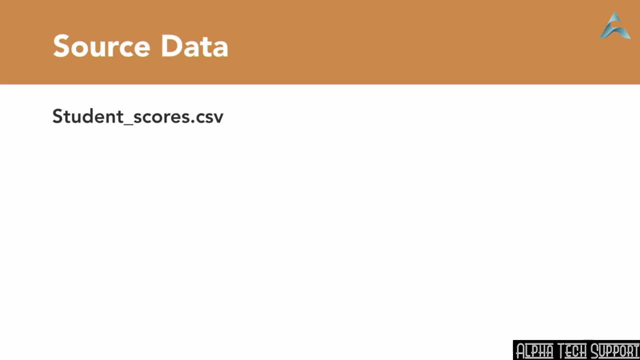 This file has students' course by subject during a school year. There are four attributes in this data source: The student name. The subject. The test score which indicates the score the student got from his assignments. And the test score which indicates the score the student got from his final examination. 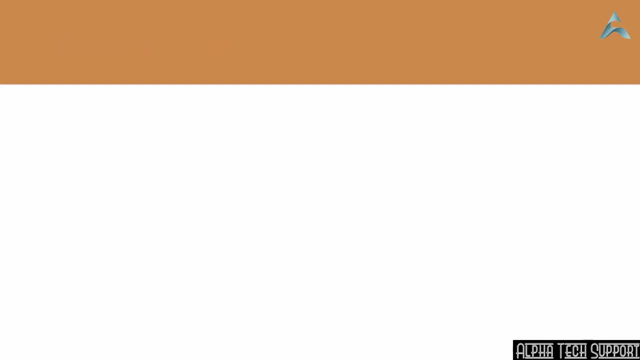 The use case. actions to execute are as follows: Load the CSV into HDFS. The data should be loaded in parquet format and the compression used should be gzip. Choose a partitioning scheme that would fit this data, based on the analytics problems solved in this use case. 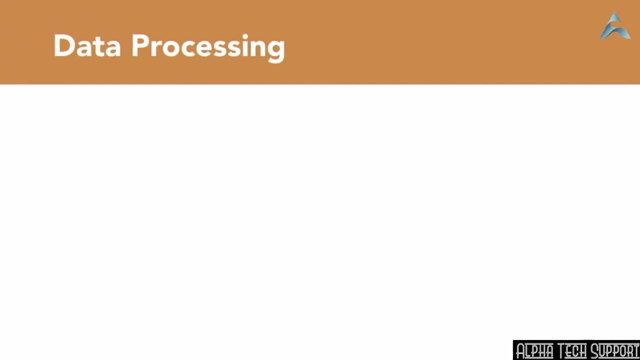 Next, read the data from this HDFS store and analyze the following. First, compute the total score for each student per subject. The total score is the sum of class score and the test score. Then print the scores that each of the student received in physics. 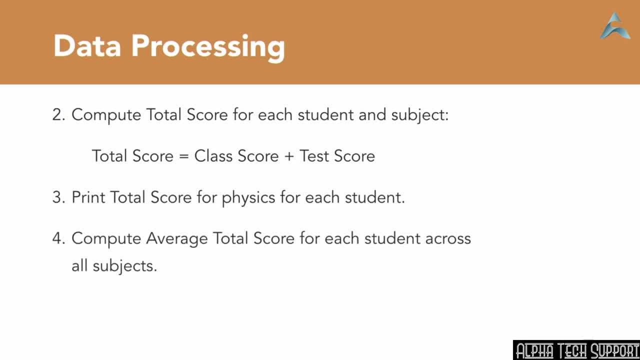 Next compute the average score of the total scores each student got across all subjects. Finally, find the student with the highest score for each subject. Analyze execution plans for all of these use case exercises. It is recommended that you try these exercises and find solutions yourself before checking on the reference solutions in the following videos. 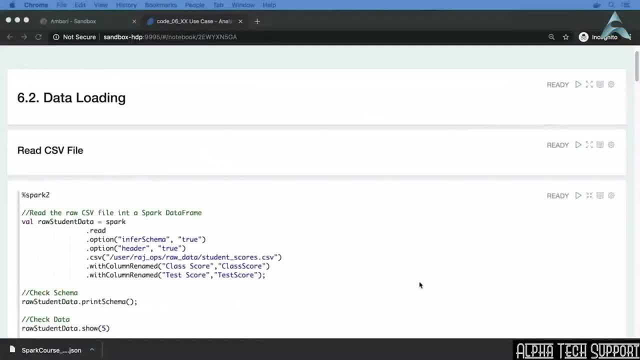 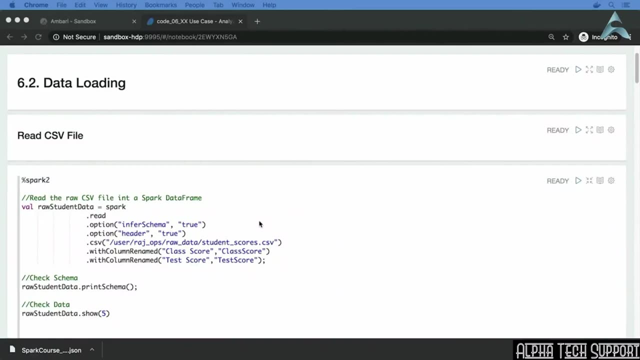 Best of luck with this use case. In this video we will look at loading the use case data into HDFS. This is pretty straightforward. First we read the CSV file into the raw student data data frame. You may face problems writing this data frame back to parquet since some column names have spaces in them. 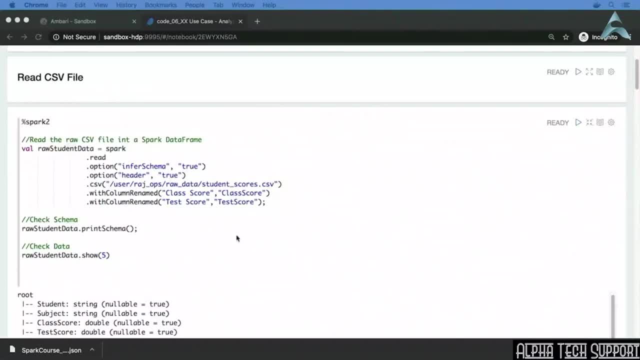 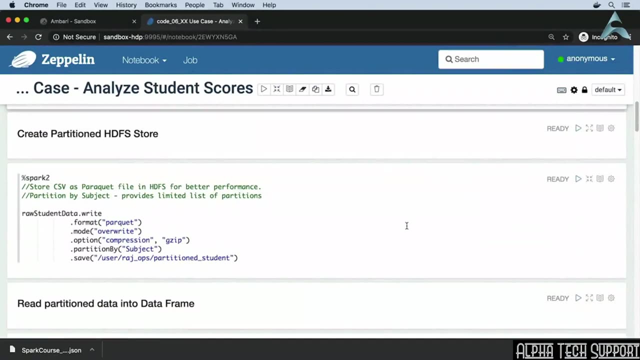 So we also rename these columns to have no spaces. We print the schema and the data. to make sure that everything went fine with the reading process, Let's execute this code. Next, we create a partition data store in parquet format and with compression as gzip, as required by the use case. 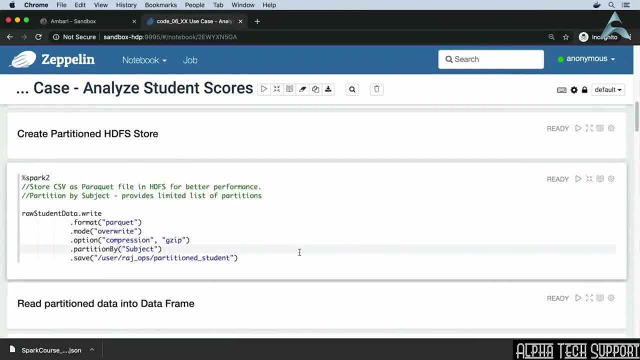 In the case of partitioning, we have two columns that are frequently used in the future exercises. They are student and subject. Both are extensively used in these exercises. We could have gone with either of them or both of them for partitioning. Given that subject has a limited number of values as opposed to student names, we go with subject as the partition key. 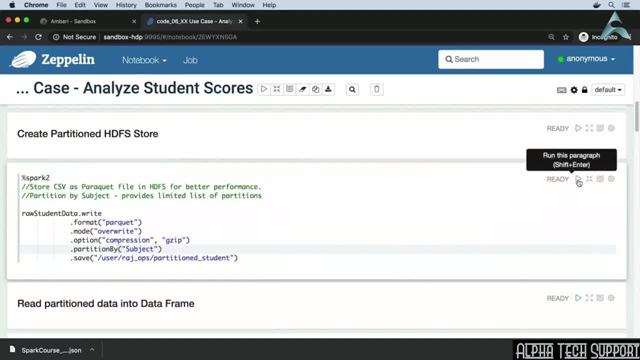 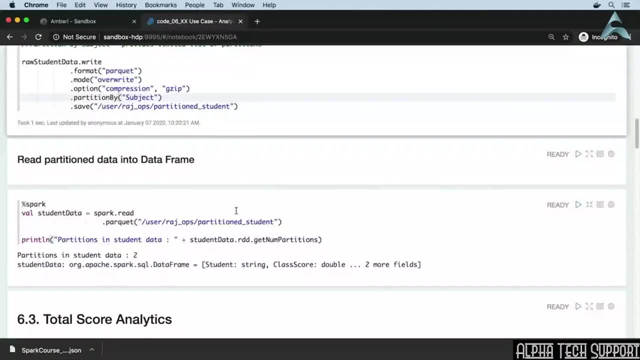 Let's execute this code too. We can check the HDFS file browser to see if the files are created correctly. Next, we read back this data into a partition data frame called student data. We check the number of partitions in the data frame. 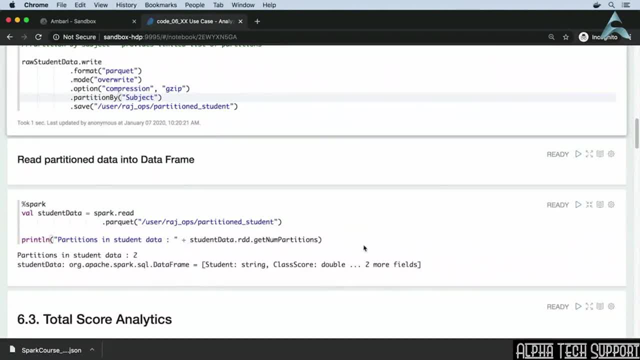 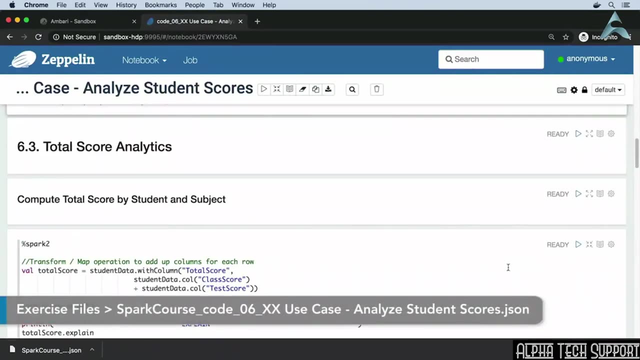 We see a value of 2, which is the default parallelism for this installation. In the next video we will perform the required analytics on this data frame. In this video we will compute the total score for each student by subject and print the total scores for physics for all students. 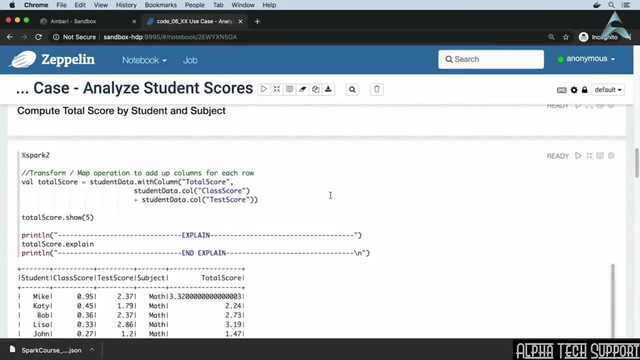 To compute total score, we will use the map transform in the data frame. We can simply use the with column function to compute the new column from existing columns and create the total score in the data frame. We then print the results. Let's execute the code now. 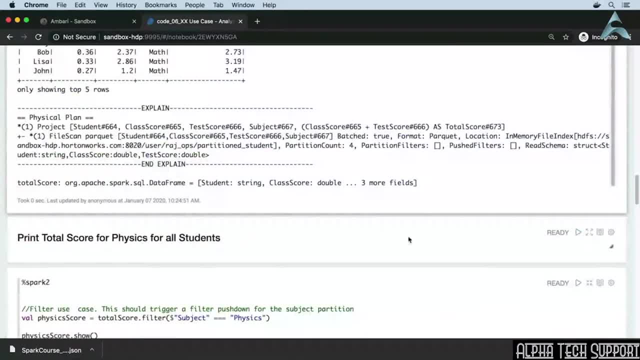 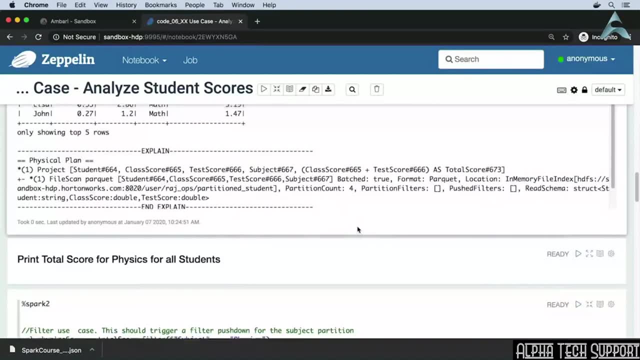 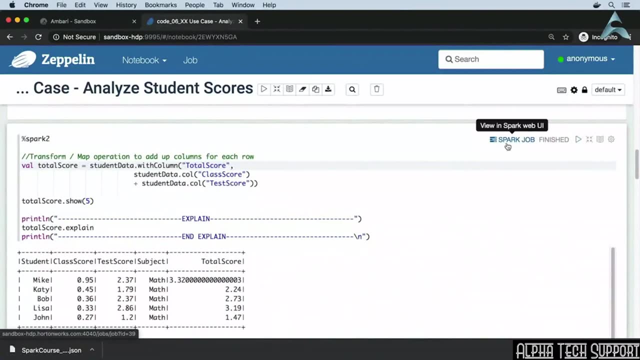 We can see the total scores computed correctly. We can also look at the execution plan to understand how the read was executed. We can also look at the Spark job UI To see how this map operation was executed. We can see that this is a simple map operation. 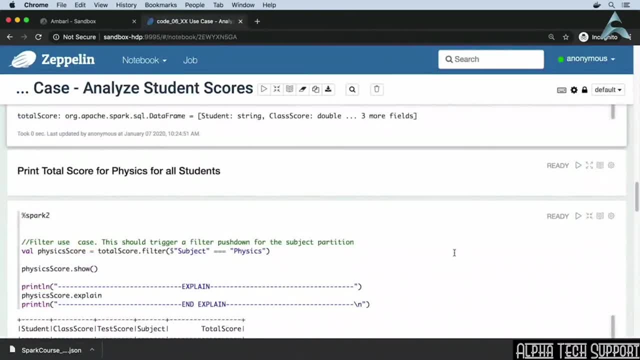 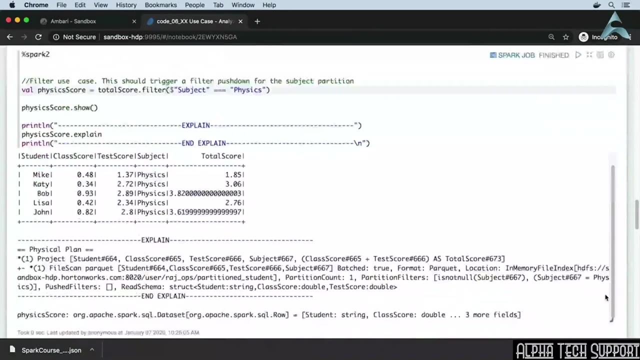 Next we print the total score for physics for all students. This is a simple filter that we execute on the subject column. Let's execute this code. We see the scores for physics printed for all the students. If you look at the execution plan. 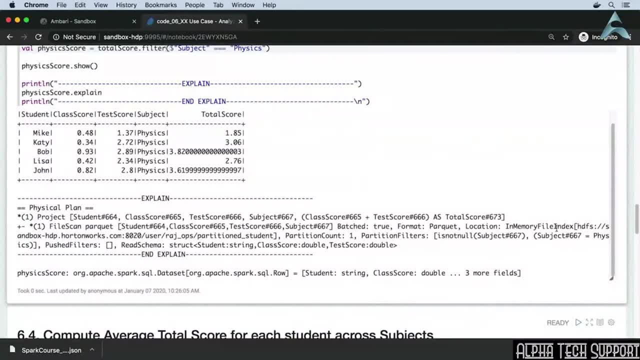 it shows that this filter has been pushed down to HDFS And only one partition has been read. But this read the data source again and computed the total score again with no caching. In the next video we will cache this data for future analytics. 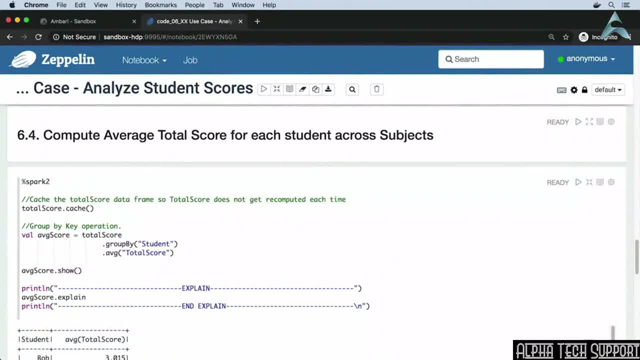 In this video, we will compute the average of the total score for students across all subjects. To begin, we will cache the total score data frame, So we don't have to read the data source and compute the total scores again and again. Then we compute the average score for each student by executing an action. 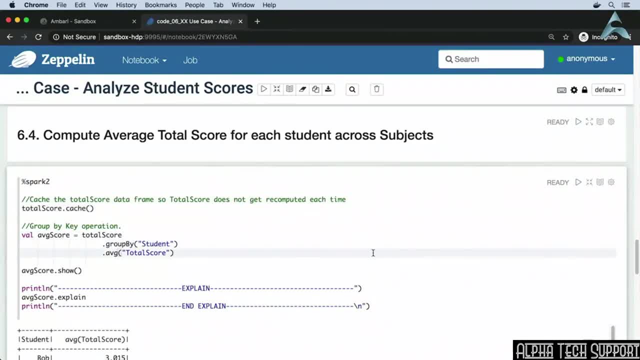 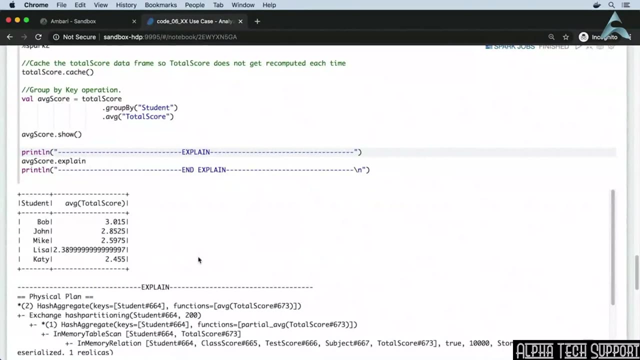 We group by the student and compute the average of the total score. We display the results as well as the execution plan. Let's execute this code now. First, we see that the average total score shows up correctly for each student, as desired by the use case. 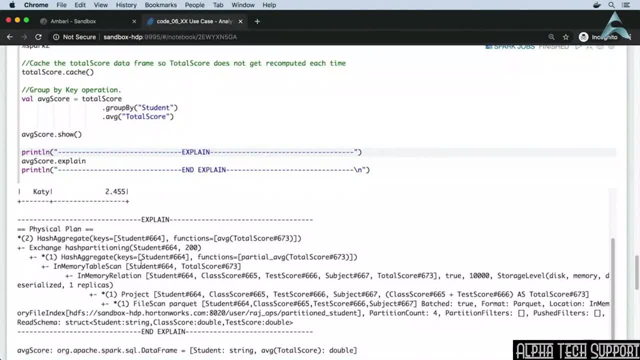 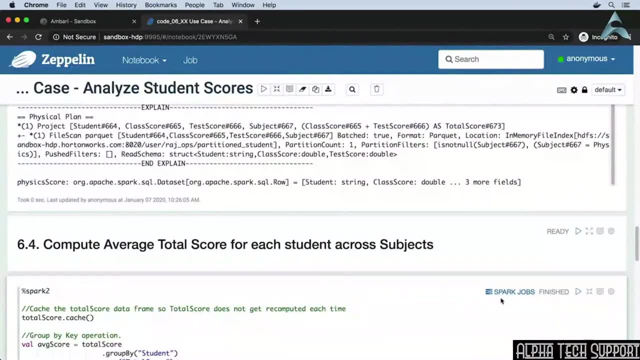 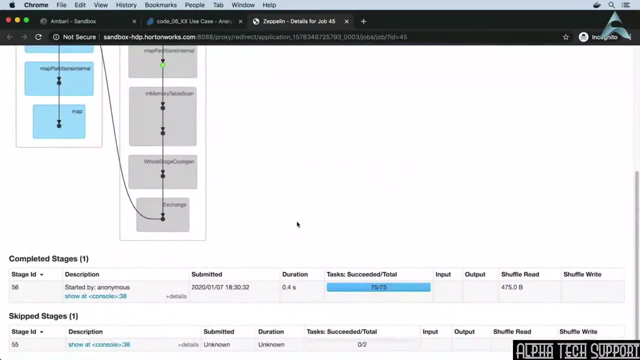 Then in the execution plan, we see that an in-memory table scan has been used. This means that the cache is working and total scores are not getting computed again. We then look at Spark jobs, number 4.. We see that there is shuffling happening, as expected, because of an action. 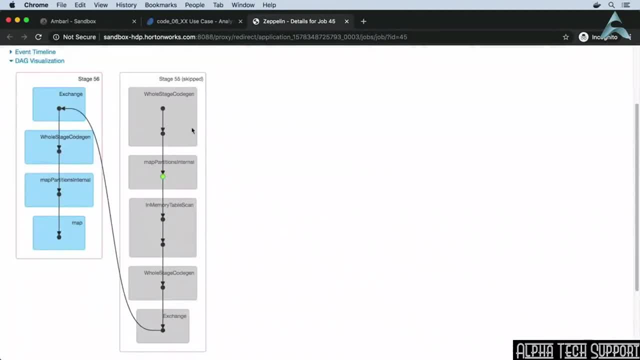 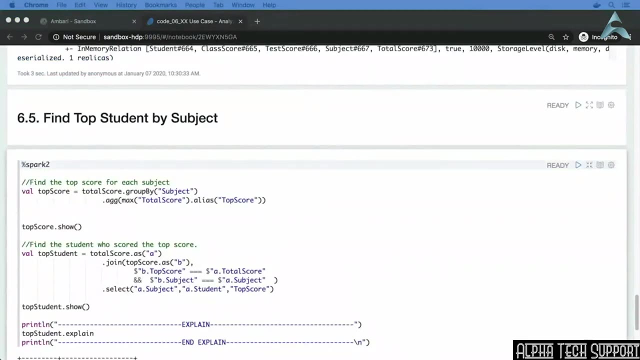 But we also see that an entire stage has been skipped because of caching. This is the desired outcome. In the next video, we will find the top student for each subject. In this video, we will find the top student by each subject in the data source. 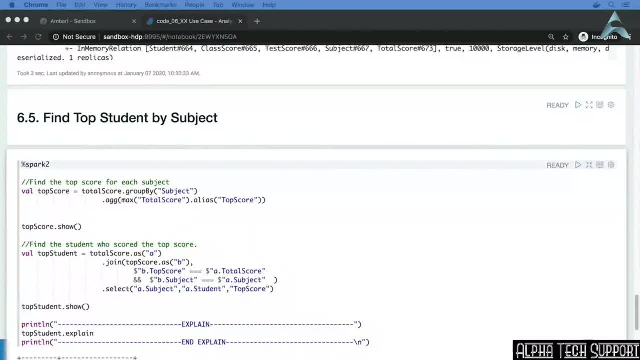 This is the time to evaluate if we need to do repartitioning. Given that we have not generated any result data frames from an action that needs further transformations, we don't need to look at repartitioning. Finding top students by subject is a tricky use case and there are multiple ways to achieve it. 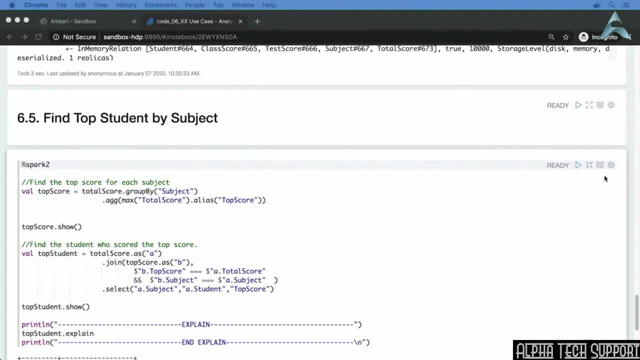 In this reference, we first find the top student for each subject, Then we find the student who got the top score. To find the top score for each subject, we simply group by subject and find the maximum of the top score. The results are stored in the top score data frame. 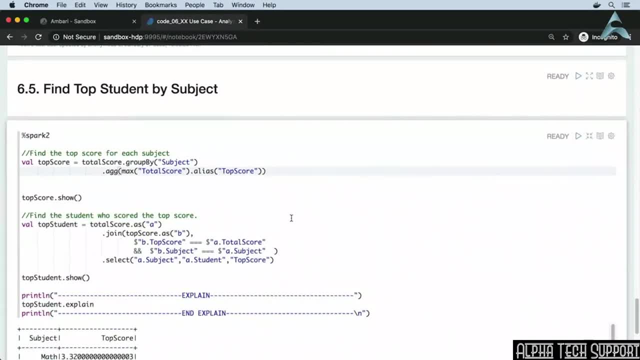 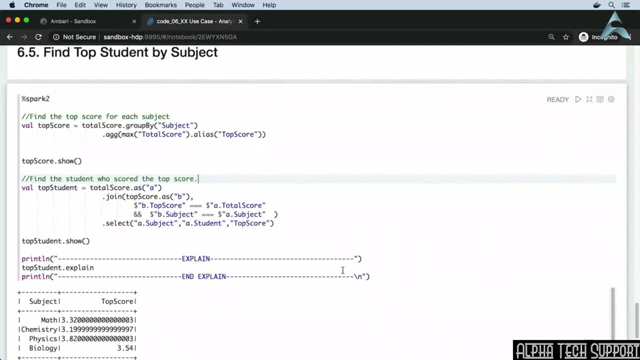 Then we join the top score data frame with the total score data frame, based on both the subject and the total score value. This will extract the list of student records that had this top score. We then print the results and also run an explain of the results. 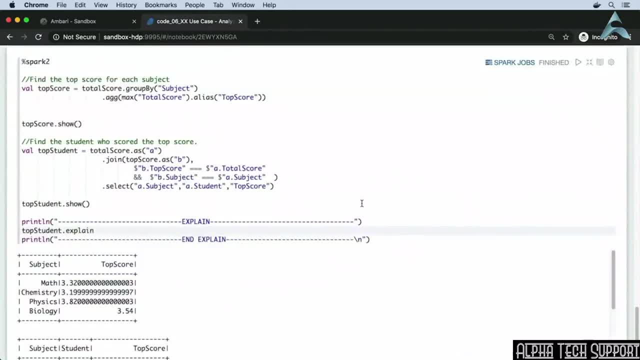 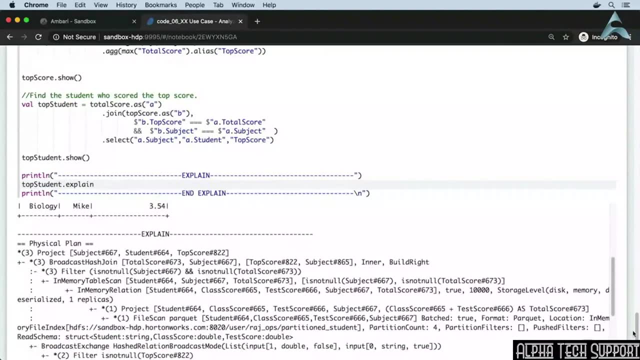 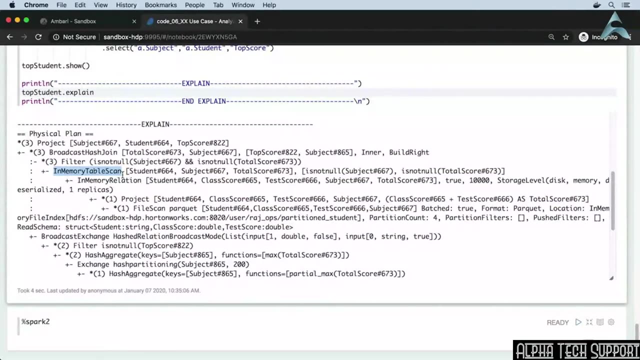 Let's execute this code now. We see that the students with the top scores are printed correctly, as required by the use case. In the execution plan, we again see that the cache is being used Also. Spark optimizer has automatically decided to broadcast the top score data frame.